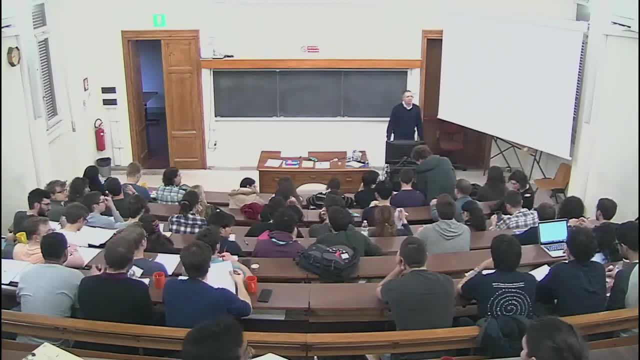 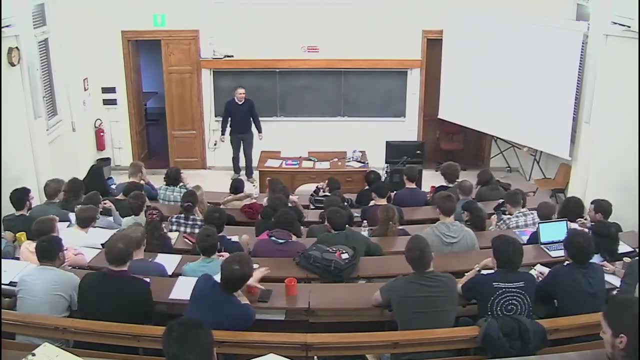 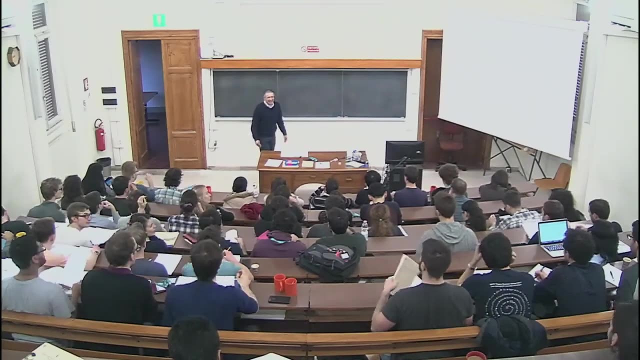 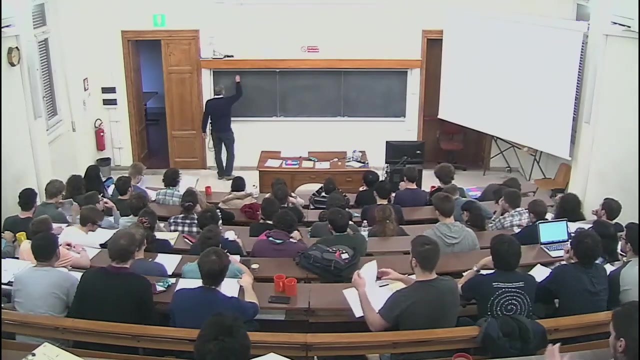 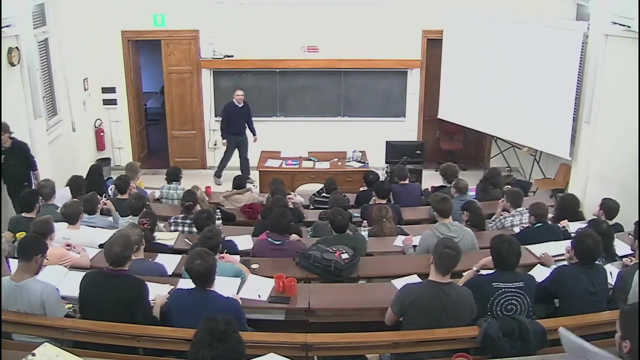 Okay, so good morning. I have a couple of leftovers from yesterday's lecture because my friend Ricardo pointed out that a few things I said were not exactly correct. so now I correct myself. First one is the following: The three matrices, tau1, tau2, and tau3 deserve the name of generators. 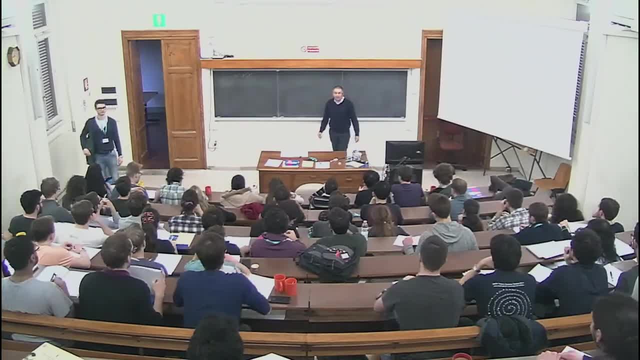 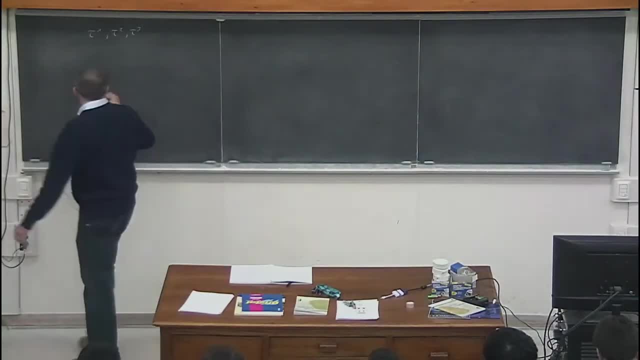 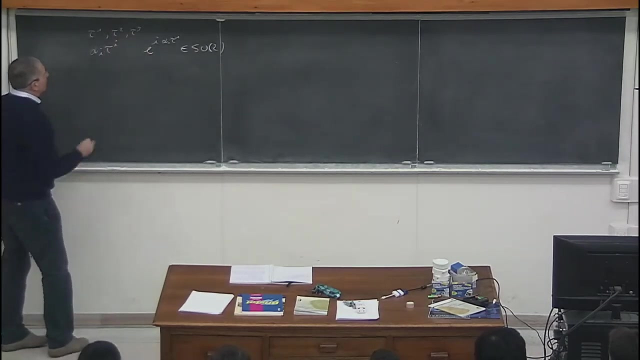 of the SU2 algebra in the fundamental representation, in the sense that if you take a linear combination with real coefficients of these three matrices, then the exponential of i, alpha, i, tau, i- is a member of SU2.. And in order for this to be true, these three matrices must be: 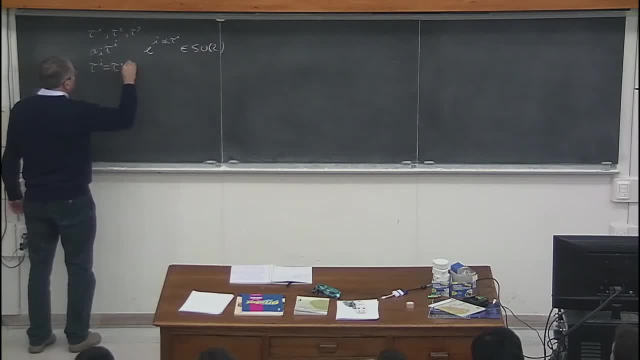 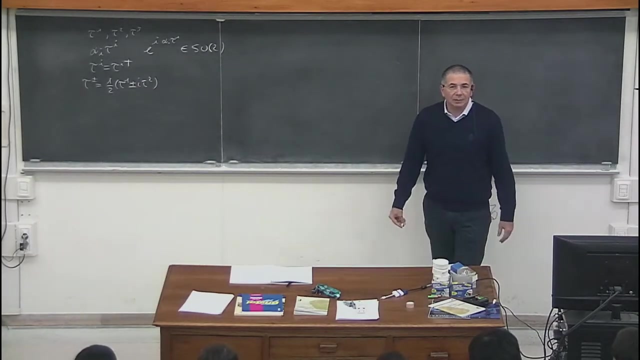 omission- self-adjoined matrices. For the same reason, tau plus and tau minus, which are defined like this, do not deserve the name of generators because they are not self-adjoined matrices. So this procedure is very familiar to all of you because it's the procedure which is used in the Cartan method to determine. 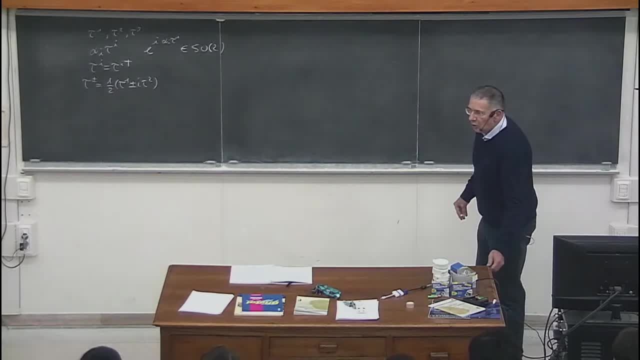 the representations of the algebra of the rotation group. But anyway, these are not strictly speaking generators. The three generators are tau1, tau2, and tau3.. This is the first thing. The second thing is that the three generators are not self-adjoined matrices. They are not self-adjoined matrices. 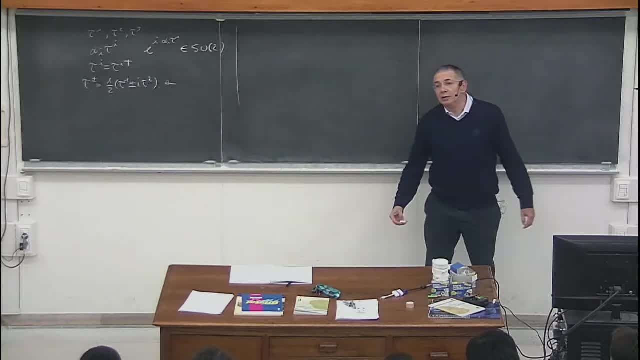 The second one is that I said something about the unitarity of the Fermi theory, and I said that the Fermi theory is not unitary in the sense that the S matrix, which you get from computing amplitudes by the Fermi theory at some point 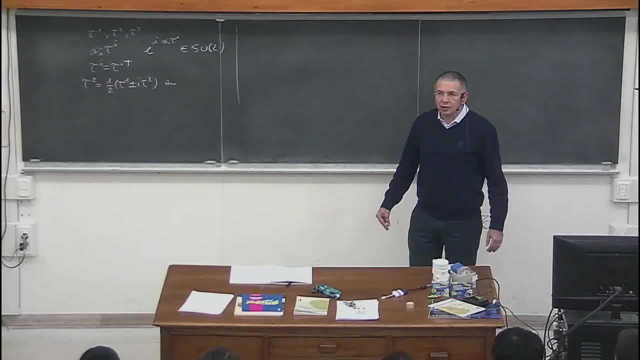 for sufficiently high values of the energy do not respect the unitarity bound. This is true, but of course it's true in a perturbative sense, in a sense in which the amplitudes are identified with the amplitudes computed at the lowest order in perturbation theory. If one were able to compute the exact matrix elements, 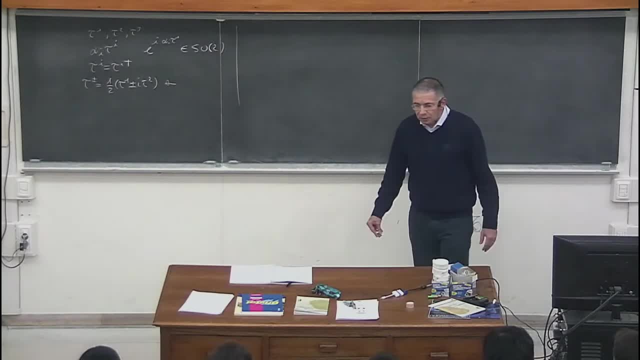 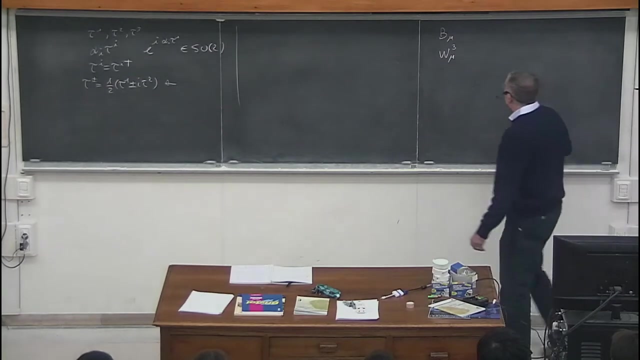 of the scattering matrix, then one would obtain a unitary, presumably a unitary matrix, but this is not possible in the context of the Fermi theory. And finally, I promised you remember that we traded the two vector fields which are coupled to neutral currents in our construction for a new pair of vector fields. 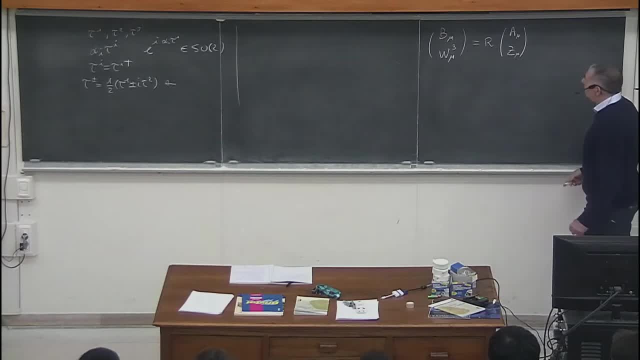 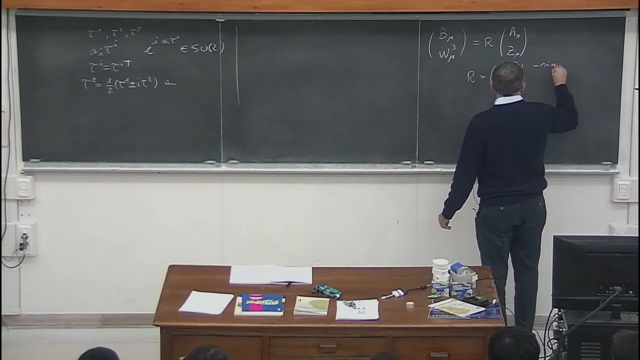 which I called a mu and z mu, and the relationship between the two pairs is given by a matrix which I chose to be a rotation matrix. This is an orthogonal matrix- R, R transpose is equal to identity matrix, and I promised you that I would give you a motivation for this choice, which I 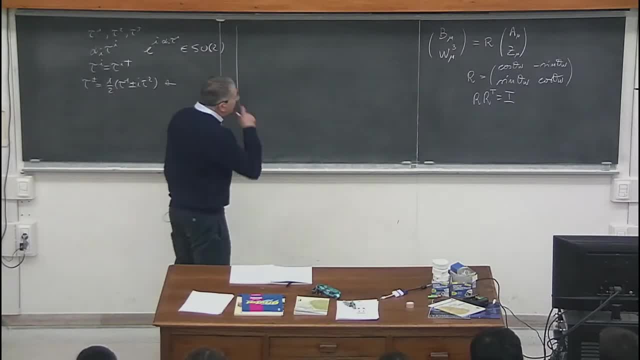 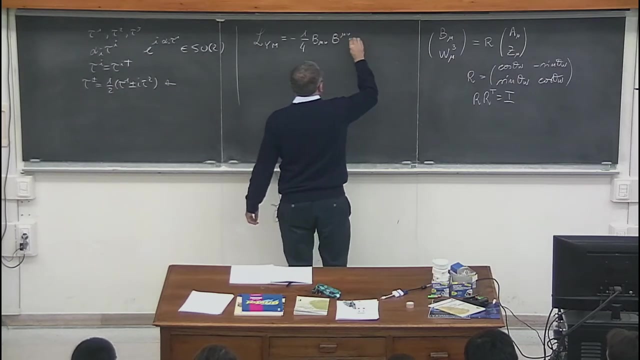 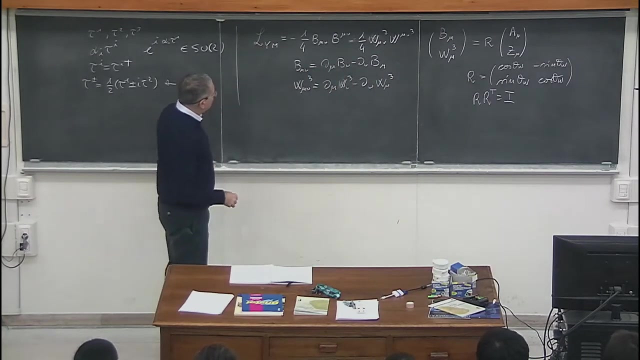 didn't. so I now keep my promise, And umm reason is the following: you remember that the young mills terms term for the full Lagrangian density has a term which is like this: well being, you know, is equal to and, of course, since the parameter theta W, which appears in R, is a constant, 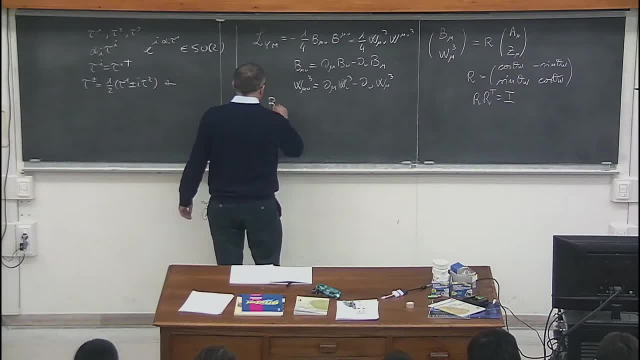 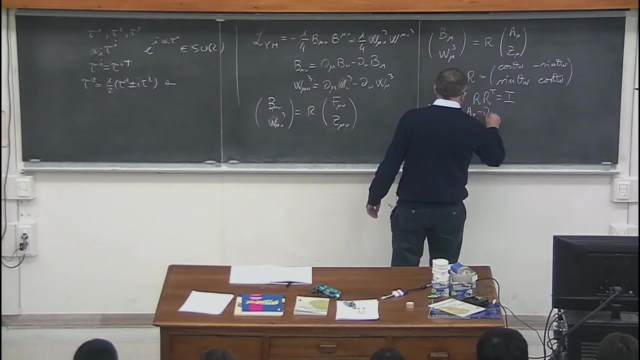 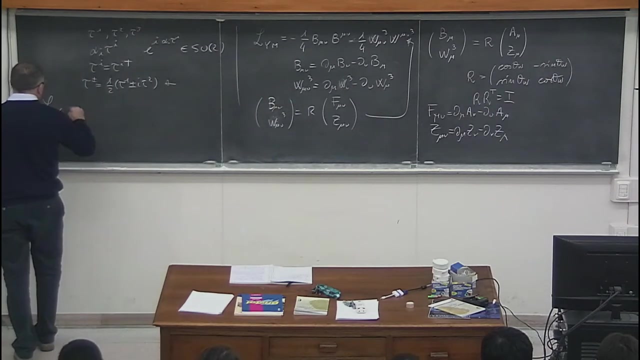 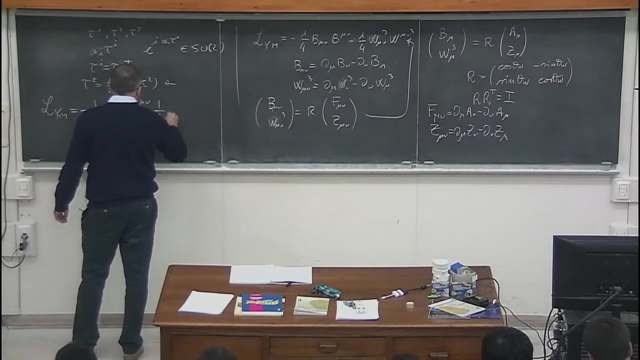 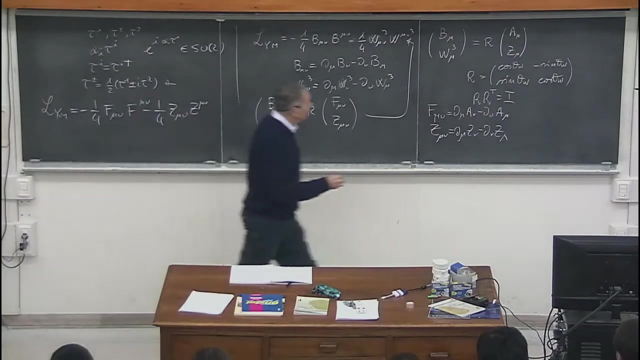 parameter is not X dependent. you have that being. you knew W. you knew three is equal to R, have you said, you know where. so if you plug this into these, what you get is- and it is because of the choice of the matrix- are as an orthogonal matrix if 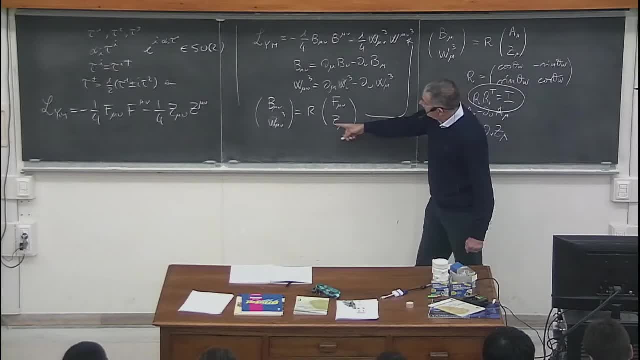 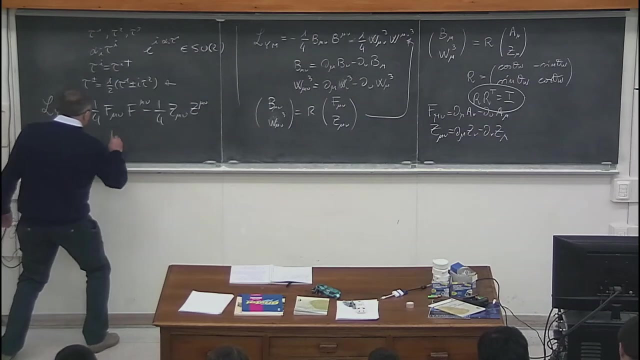 you replace being you knew, and W million three by this expression. here you get an R, R transpose here, or rather R transpose are, and this cancels because the matrix R is orthogonal and you get again a diagonal term for the kinetic terms, for a new, and there is no mixing between the two, which would be nasty. 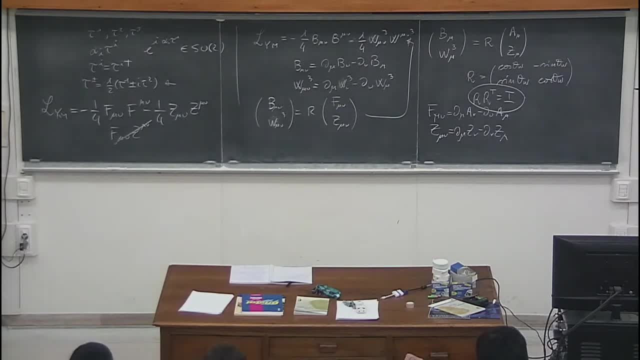 because when you compute the propagator, what you would like to have is a quadratic part of the Lagrangian which is diagonal in each field. So this is the reason why Glashow decided to rotate B mu and W mu nu 3 by an orthogonal transformation. 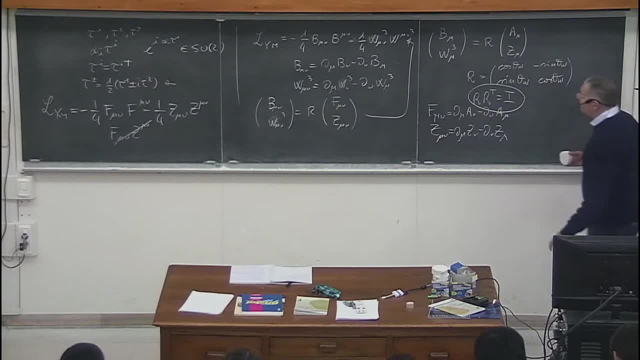 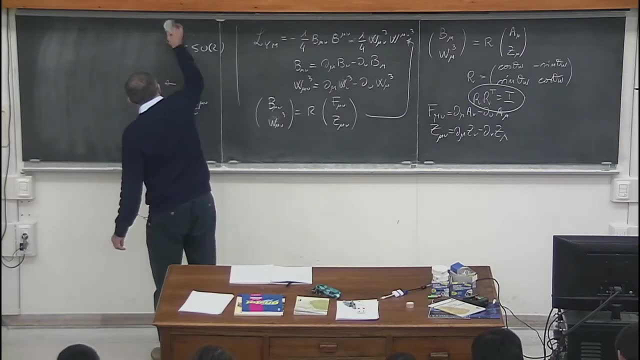 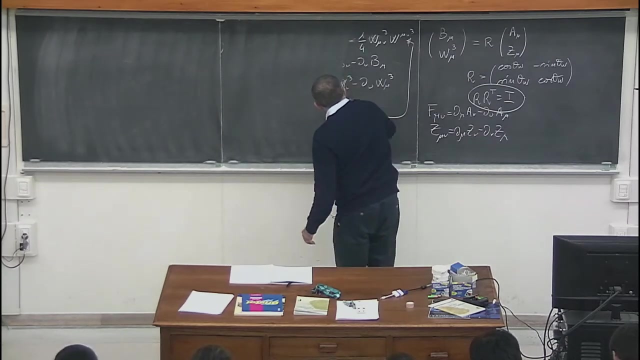 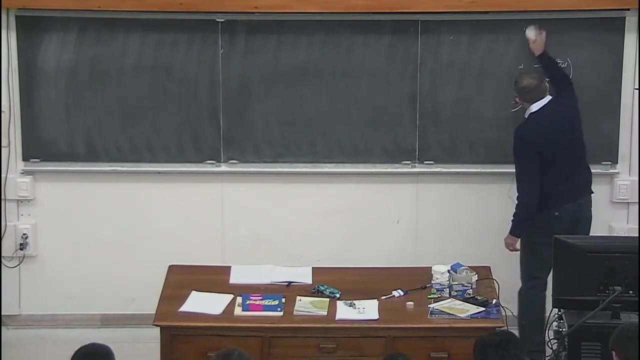 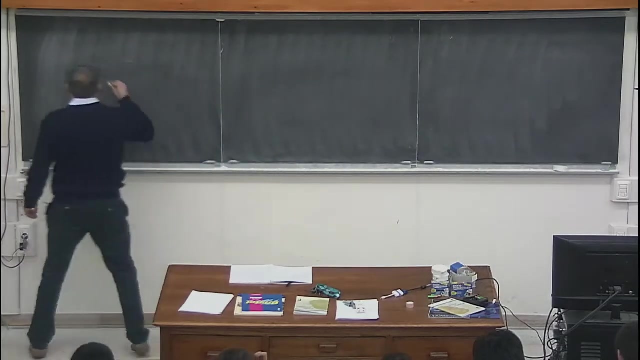 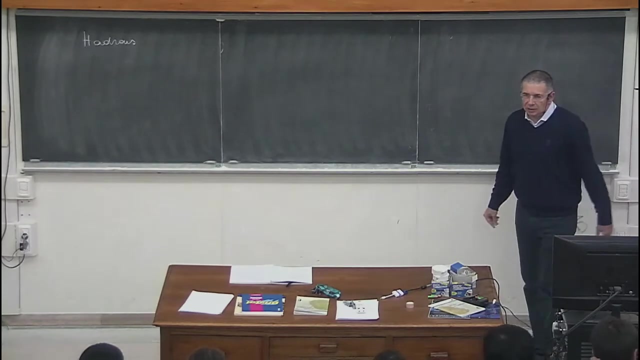 So this completes yesterday's lecture. We can start today's lecture. As I said, our next task is to include hadrons in the game. So far, we have only described the weak and electromagnetic interaction of LEP. We have described the weak and electromagnetic interaction. 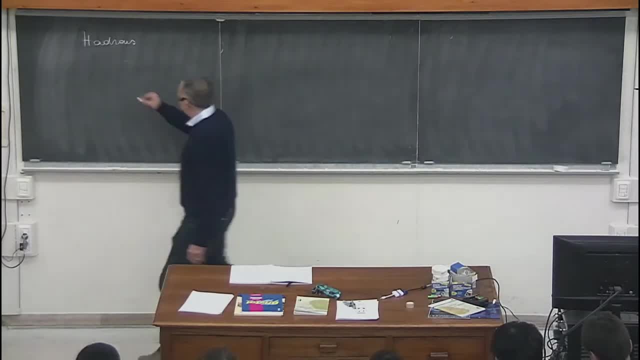 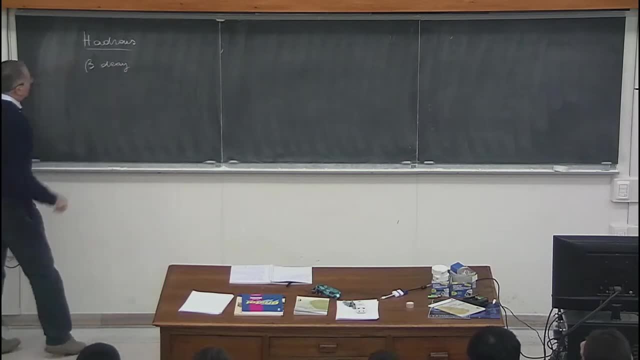 of the two neutrons: the muon, the electron and their neutrinos. And now we have to say something about hadrons. We already said that there is beta decay of nuclei. Beta decay can be interpreted as a decay of a neutron. 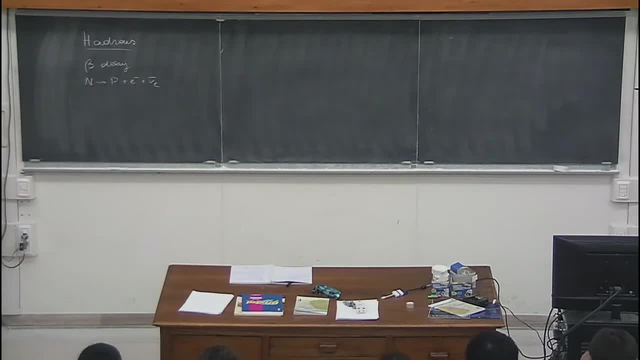 into a proton plus an electron plus an anti-neutrino, And this is something that we all are familiar with. This can be, since the neutron has a composition in the quark model which is up down down, and the proton is up up down. 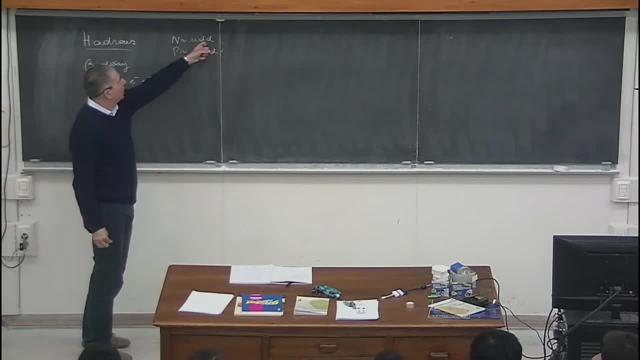 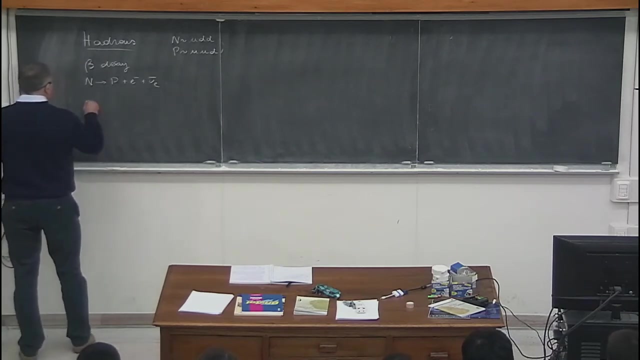 the up quark has charge 2 thirds in units of the proton charge and the down quark has charge minus 1 third. So you can interpret this decay in terms or in the context of the quark model. 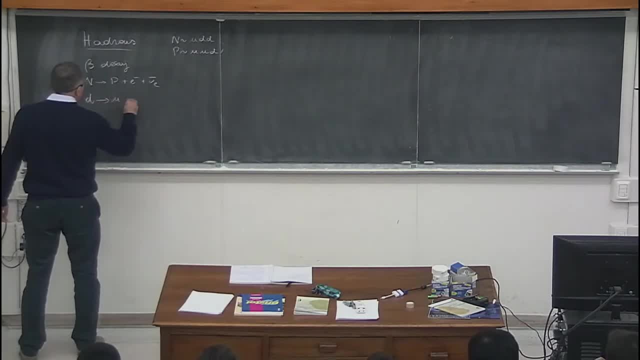 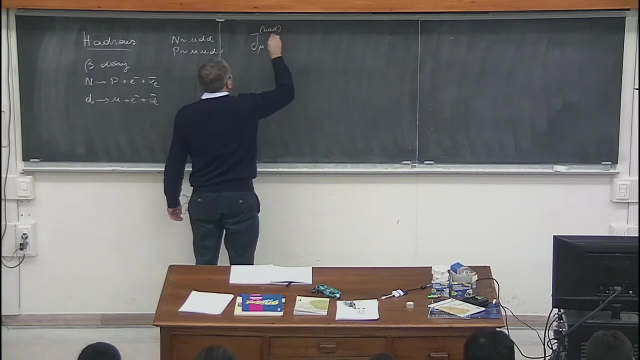 as the decay of the d-quark into an up quark plus an electron plus an anti-neutrino. So what you need is a term in the hadron category, in the Hadron current, which is something like. I leave some space here for reason. 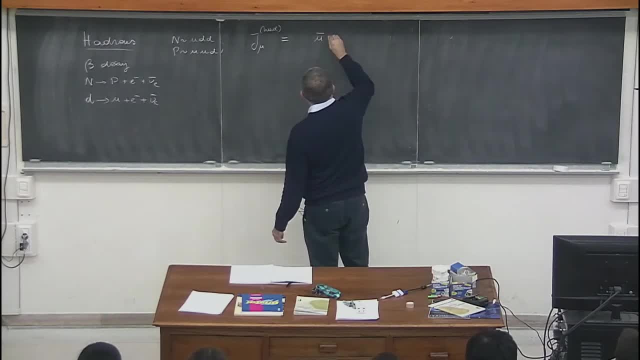 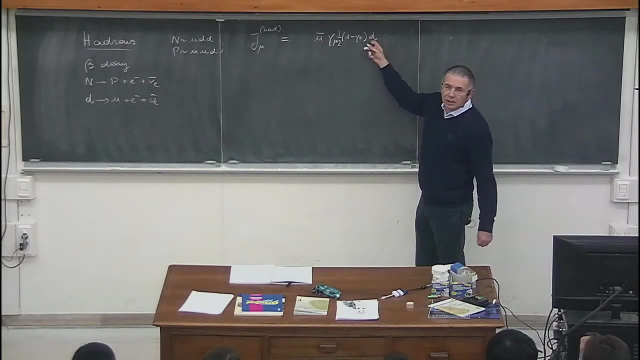 that will be clear in a moment. U bar gamma mu. one half one minus gamma five D. This is what you need in order to destroy a D quark, a down quark, in the initial state and to replace it by an up quark in the final state. It was clear very soon in the history of weak interactions that the up and down quark are not enough to describe the real world. The real world contains much more than this. In particular, it contains strange particles. There is a family of Hadrons. which you can produce By making a pion-nucleon collisions at sufficiently high energies, And this new family of Hadrons carry a new quantum number which was called strangeness at the time, And it is still called strangeness. Strange Hadrons are, for example, the lambda baryon. 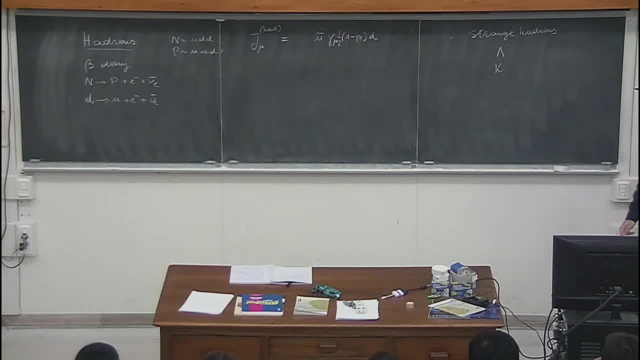 the k mesons and so on, And this family of Hadrons are produced in strong interaction processes But they decay only by weak interaction. They have a strong production process but they can only be produced by weak interaction rate. but a long lifetime because they did. yes, the reason for left projector is: 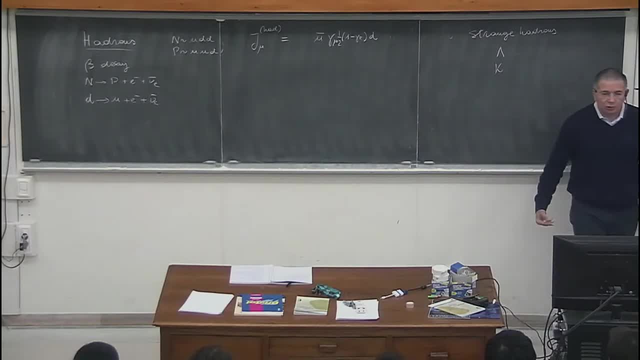 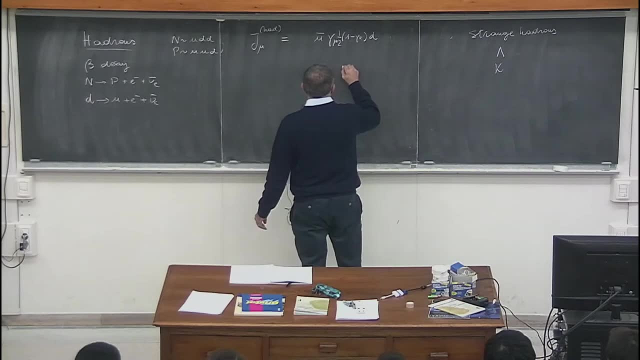 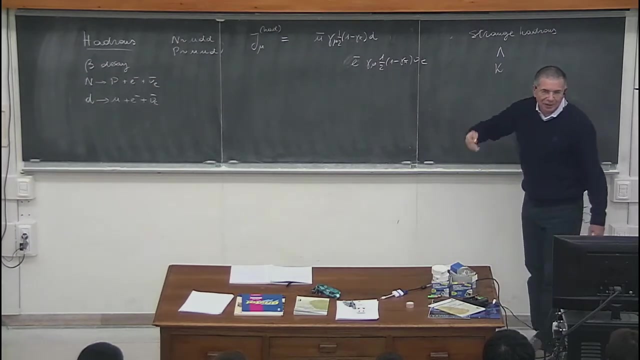 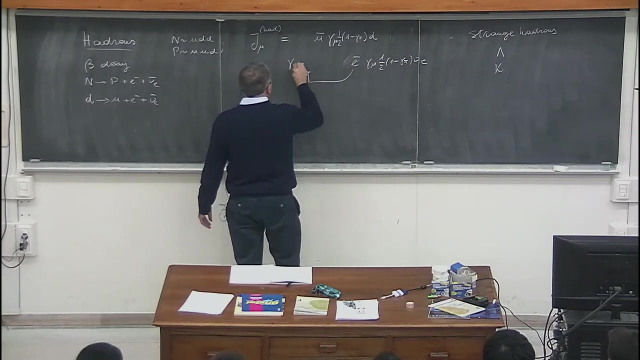 the same as the reason for left projector in cases these are coupled to a weak lepton current and this has a left projector because of the measurement of the collaborative experiment that measures the illicit e of the neutrino, which means that this is coupled to another on current which can contains both gamma Mu and gamma mu gamma. 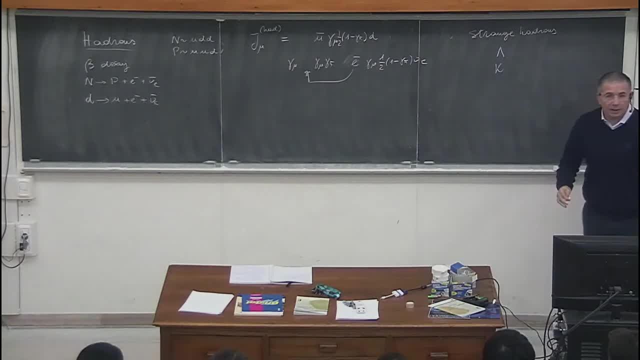 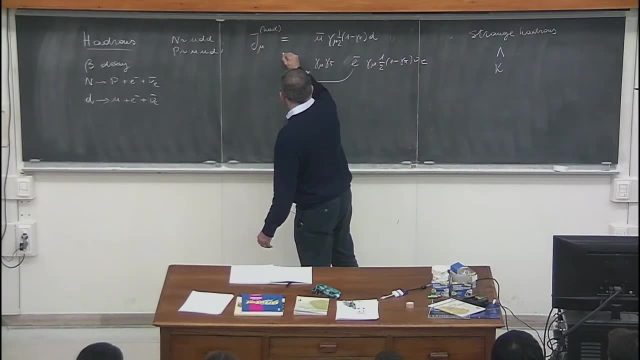 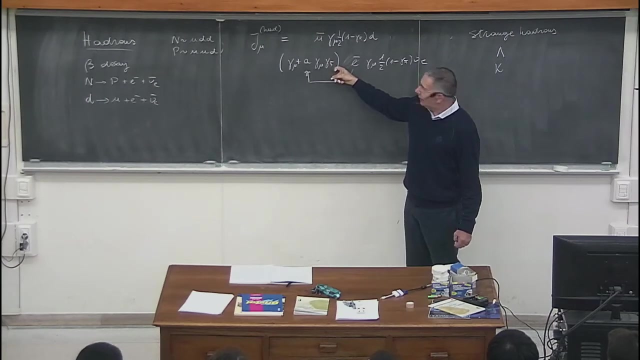 5 in principle, with arbitrary weights. then of course you can factorize the coefficient of gamma mu and give a name to the coefficient of gamma mu, gamma 5, and it turns out experimentally that this coefficient here is very close to 1, and in fact it is exactly 1. 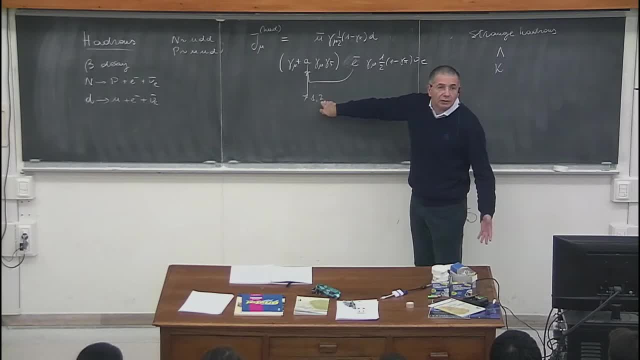 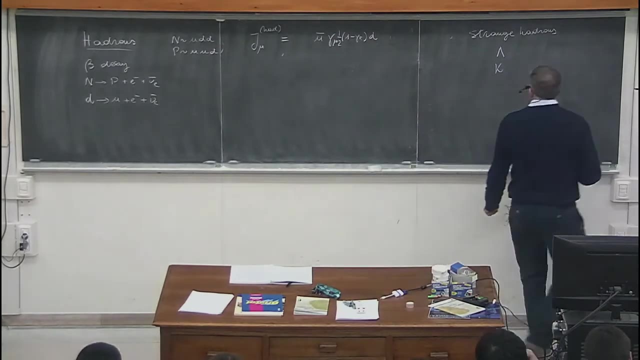 this deviation from 1 is an effect of strong interactions only. so you get left-handed production, even in the hadron sector. so you have strange hadrons, and strange hadrons decay through weak interactions, and what you need is to introduce a new quark which is called S. 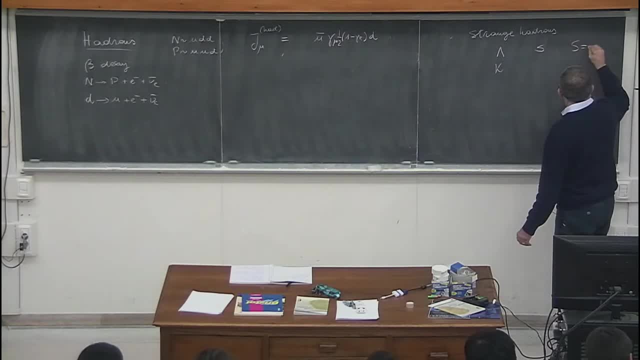 the new quark carries strangers. and the new quark carries strangers. and the new quark carries strangers. strangeness. quantum number equal to minus 1. don't ask me the reason for this minus sign. I never knew. and the electric charge is the same as the electric charge of the down quark. 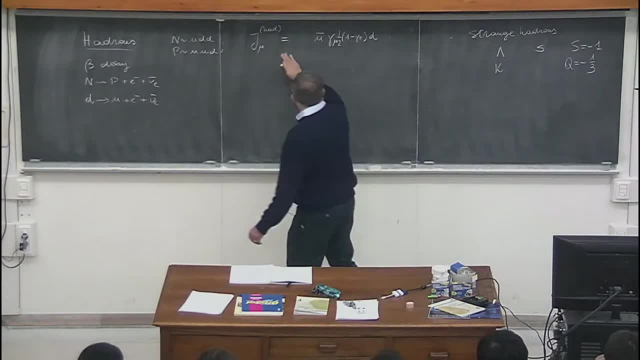 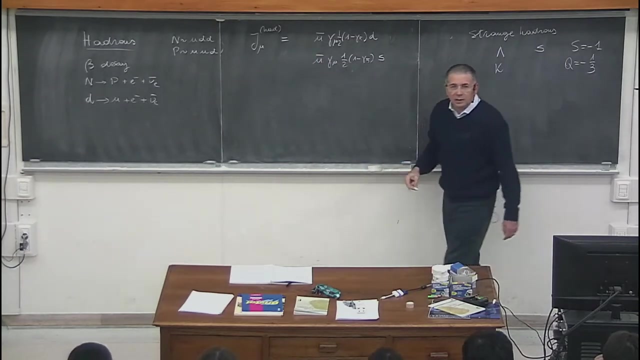 so it was soon recognized that what you need here is another term which has the same structure but with an S? quark in the place of the down quark of the previous current. and it was Nicola Khabibbo who recognized that the relative weight of these two terms in the hadron current 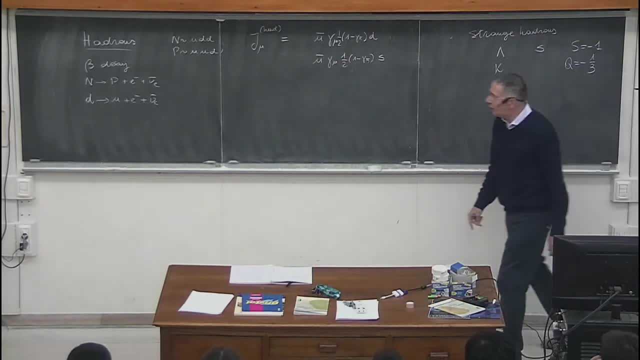 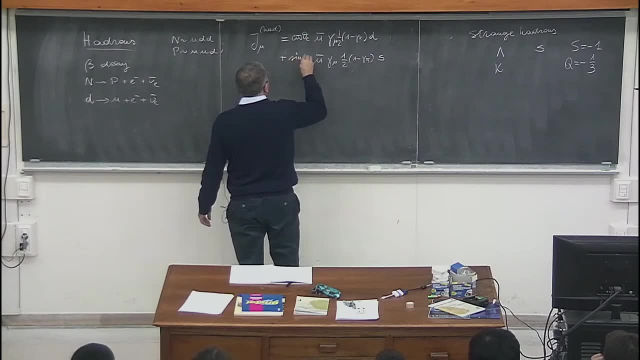 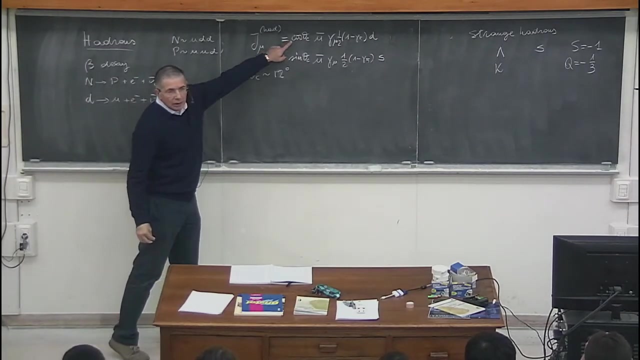 are in the same ratio as the cosine and the sine of an angle which is called the Khabibbo angle since then, and the Khabibbo angle is a small angle. right here you can see that the degree of the weight of the charge is 12 degrees, something like that. the weight of the charge hadron current, which governs beta decay, is much larger than the weight of the charge current term governing strange hadron decay. this is phenomenological. this comes from the measurements of the lifetimes of the lambda barion, of the k-masons and so on. 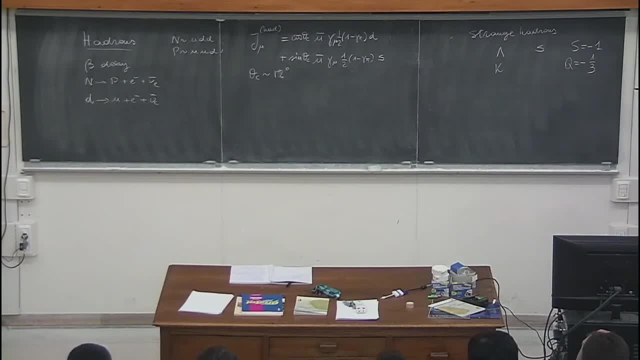 so one would be tempted to proceed as in the case of leptons. I can write this like: U bar L, gamma, mu times, a linear combination of the down quark and of the S quark Dirac fields like this: cosine theta W times d left, plus sine theta cabibbo S left. 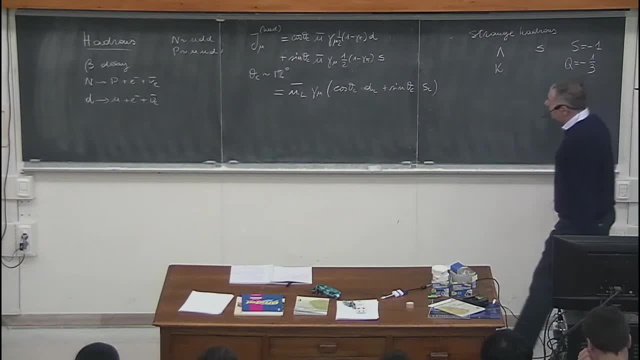 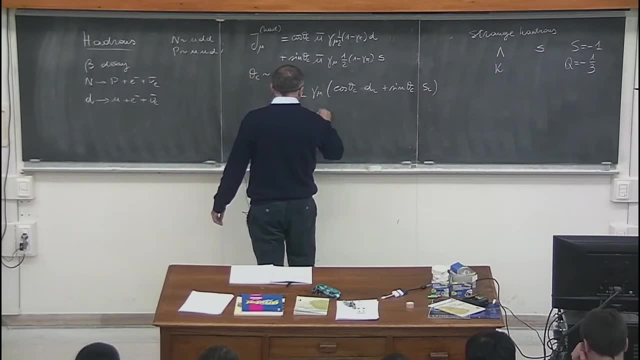 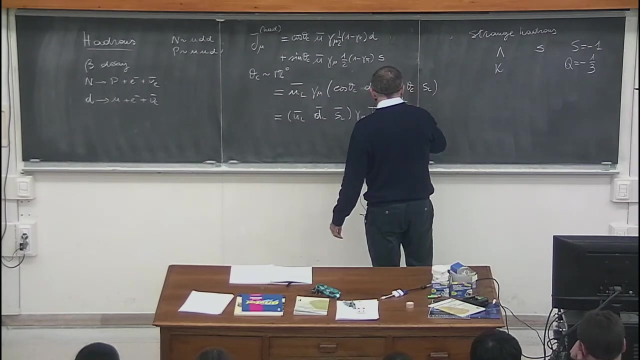 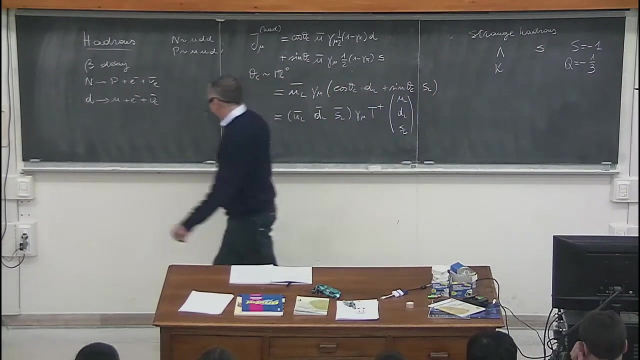 and again I can cast this in the form of a noether current by introducing a triplet of left-handed quarks. and again I can cast this in the form of a noether current where this matrix here, which I don't dare calling a generator, is. 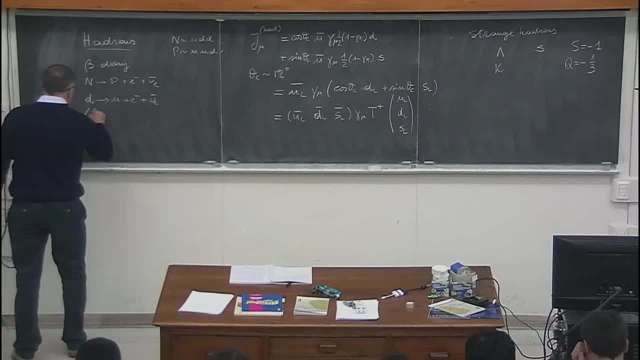 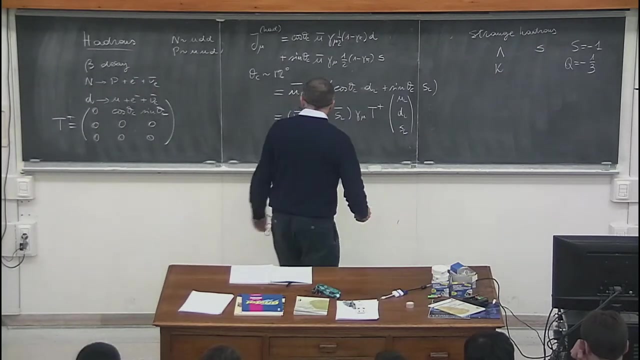 0 cosine theta cabibbo sine theta cabibbo, 0, 0, 0,, 0,, 0, 0, and again, I can cast this in the form of a noether current, but this looks nice. I can observe that there is also the Hermitian conjugate current. 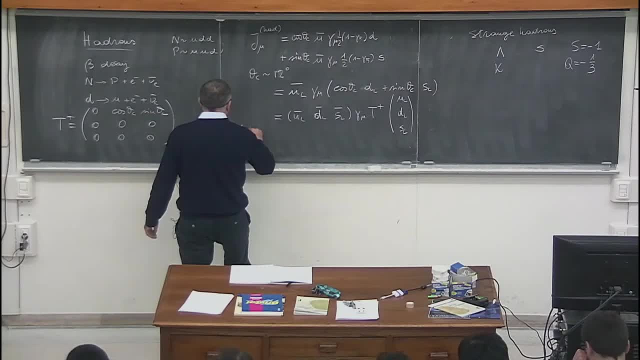 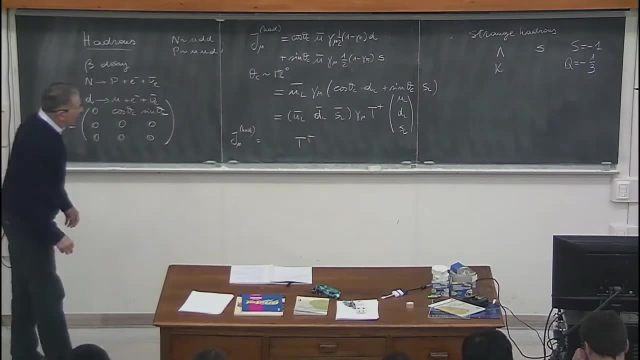 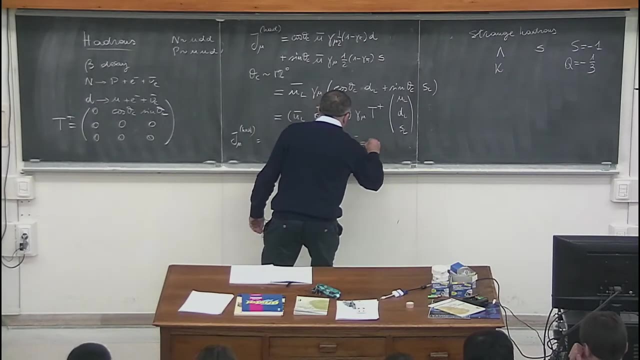 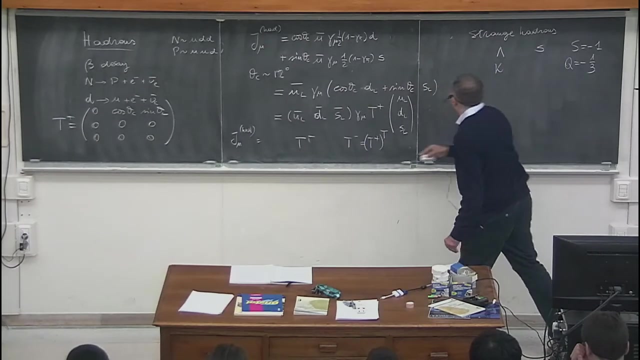 J mu hadronic, which is just the same with T minus, T plus replaced by T minus and T minus, is simply transpose matrix of T plus and if I do that, I should proceed as we did yesterday with tau plus and tau minus and compute the commutator of T plus and T minus. 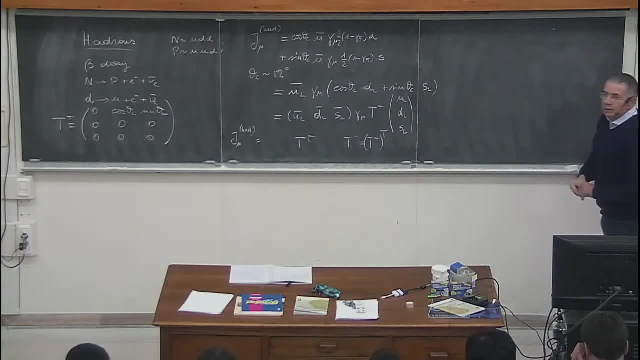 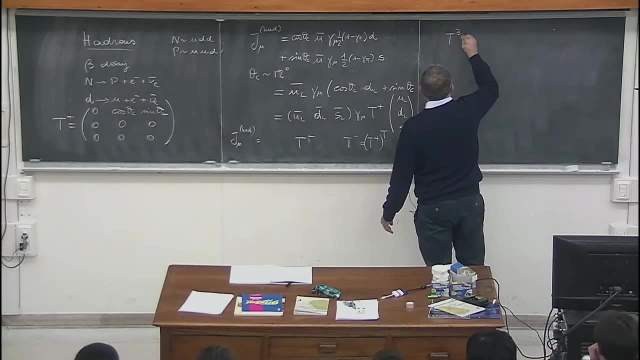 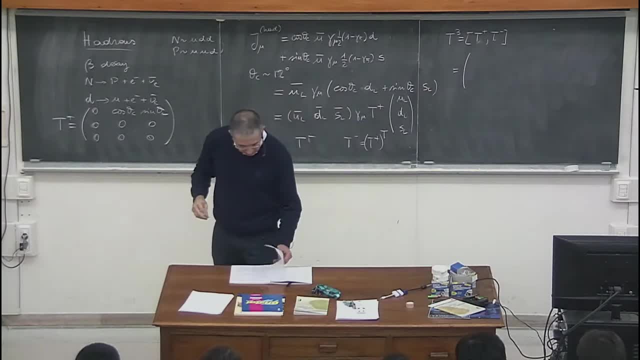 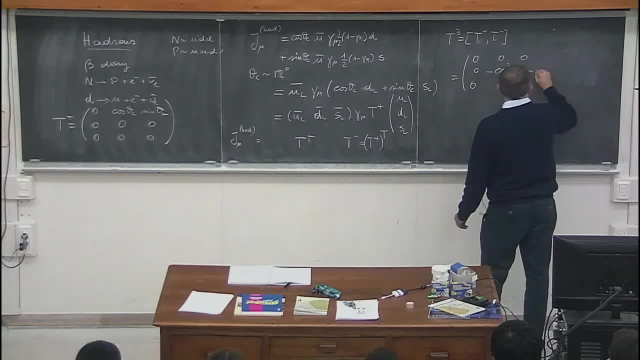 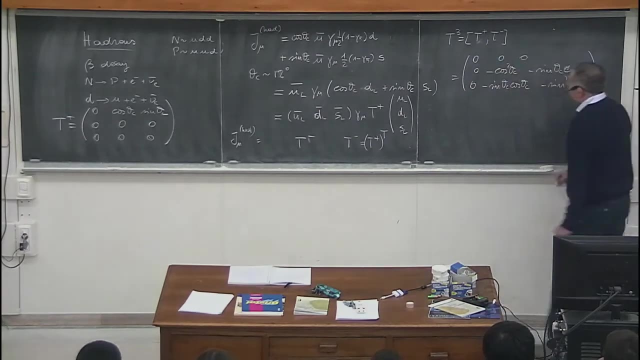 T30, T31, T32, T33, T33, T34, T35, T36, T37, T38, T39, T40, T41, T42, T43, T45, T46, T47, T48, T49, T50, T51, T52, T53, T54, T56. 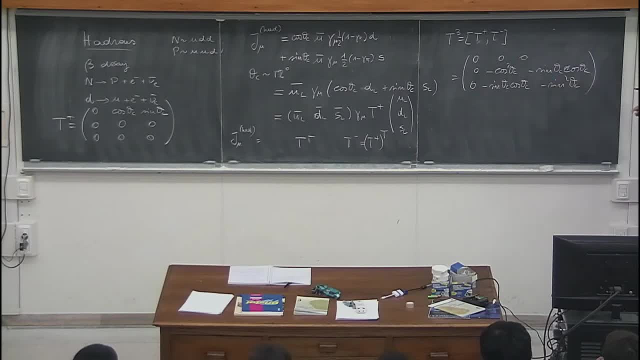 T57, T57, T58, T59, T30, T31, T32, T33, T33, T34, T35, T36, T37, T38, T39, T40, T41, T42, T43, T44, T45, T45, T46, T47, T48, T49. T49, T51, T52, T53, T54, T55, T56, T57, T58, T58, T59, T60, T61, T62, T63, T63, T64, T65, T67, T68, T69, T70, T71, T72, T72, T73. 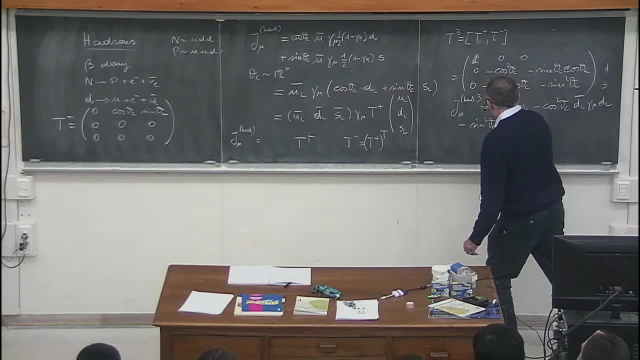 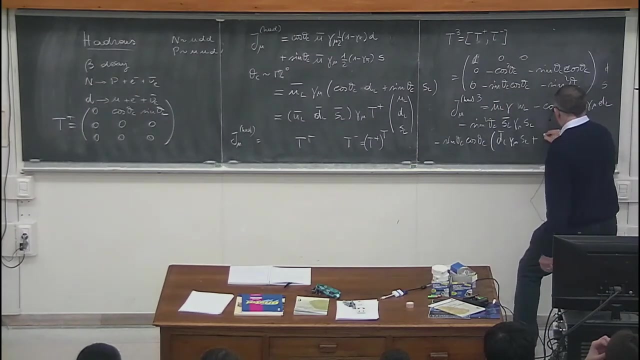 T73, T74, T74, T74, T75, T78, T78, T79, T79, T80, T80, T80, T81, T82, T82, T83, T83, T84, T84, T85, T85, T86, T87, T88, T89, T90. 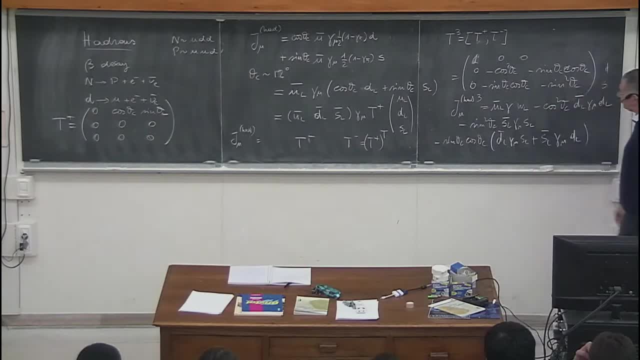 T91, T92, T92, T93, T94, T95, T96, T97, T97, T97, T97, T98, T98, T90, T90, T10, TE, T Ан, T90, T90, T90, T91, T22, T23, T24, T25. 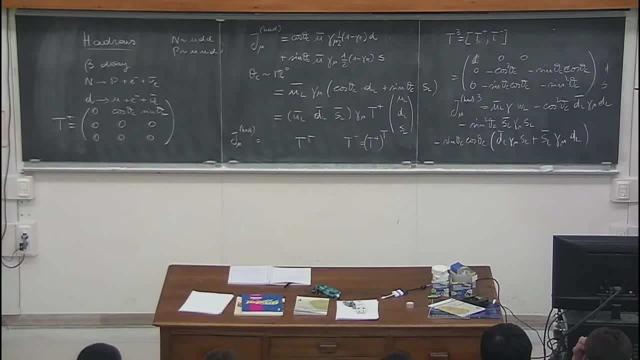 T28, T29, T31, T32, T34, T46, T37, T47, T48, T49, T21. I will tell you in a moment. Let me just complete the argument. You find that T plus minus T3 commutator is again proportional to T plus minus. so the algebra is closed. In that sense we are done. We have no more currents in the game. 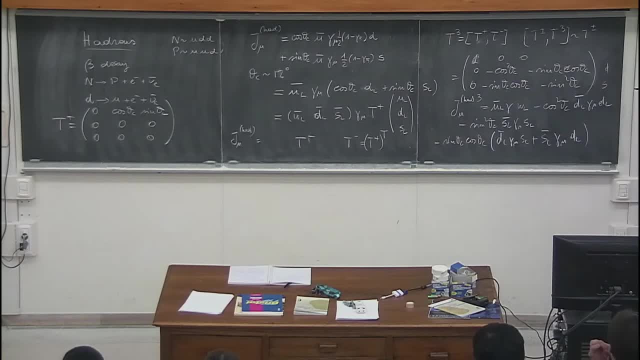 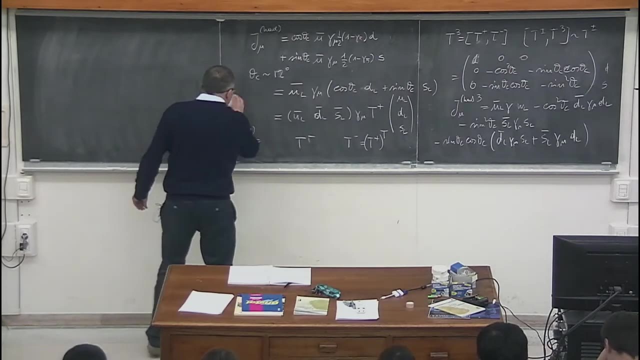 Let me tell you why flavor-changing neutral currents are not to be included in the theory. Well, the point is very simple. They are phenomenologically excluded. It is very well known that flavor-changing neutral current effects are very much suppressed with respect to flavor-changing charge current. 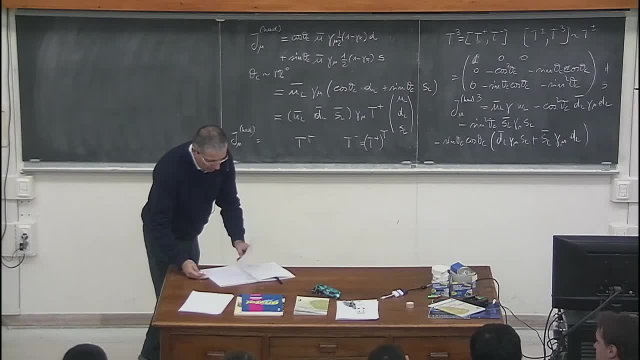 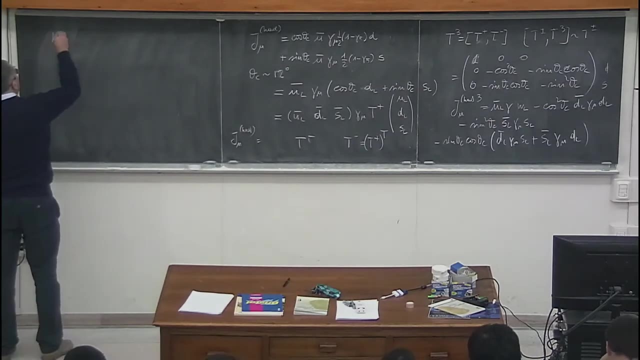 And a typical example is the decay of K3.. If you consider, for example, the meson K plus, which has a quark model composition, U S bar, The K plus meson is formed out of an up quark and a strange anti-quark, which means that it has charge plus one and strangeness plus one. 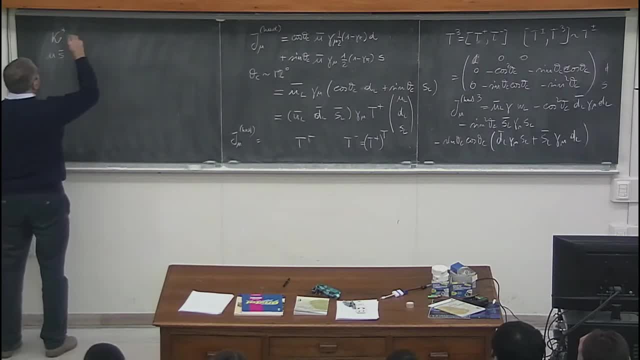 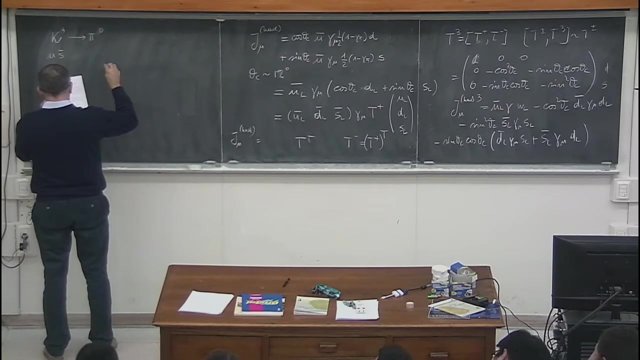 And among the decay modes of the K plus there is a beta decay. The K plus can decay into a neutral pion plus. sorry, into a charge. No, it was correct. Neutral pion E plus plus an electron neutrino. 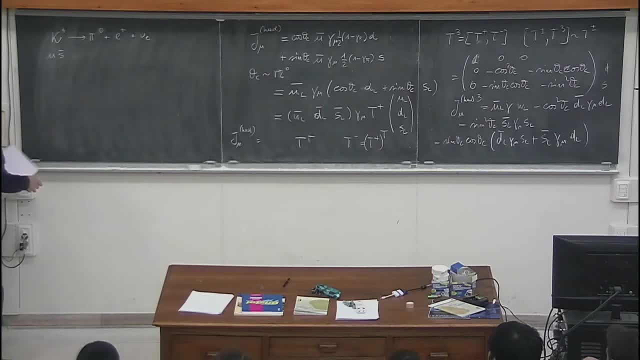 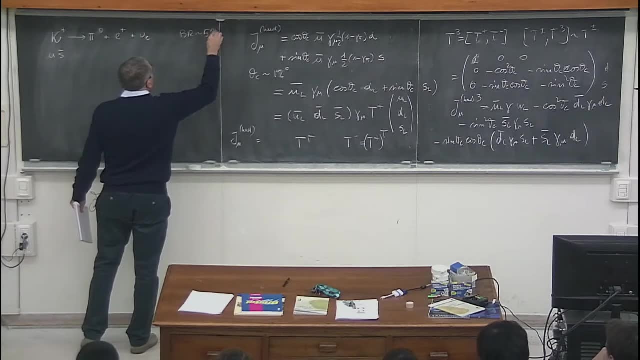 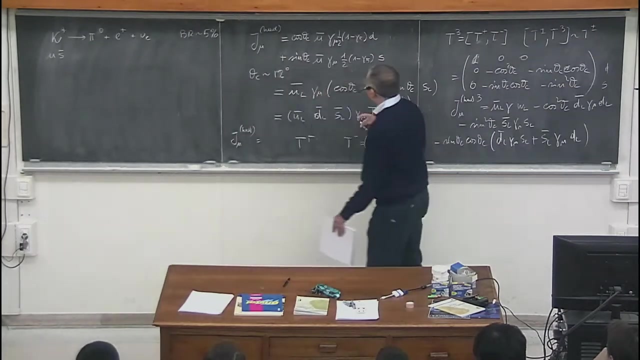 This is an allowed decay mode. The branching ratio is around 5%, so it is sizable, And this decay is clearly mediated by. I have to replace the S, sorry, the up quark. Just a second. Yeah, this is a piece I need. 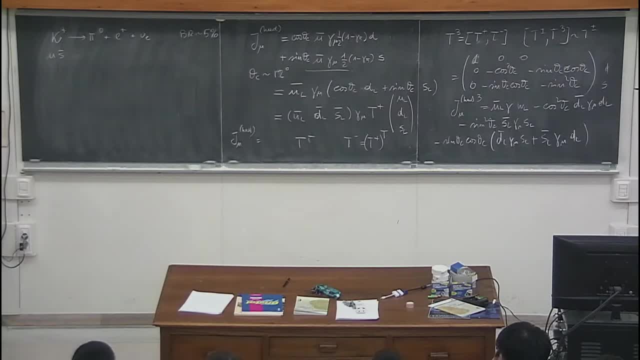 I have to replace the S bar quark by a U quark, So what I need is a. I need a term like U bar gamma mu, one half one minus gamma five S, or rather it's a mission conjugate, And this carries away sine theta Kb. 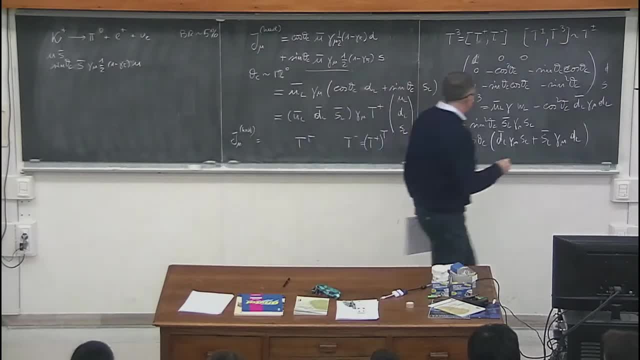 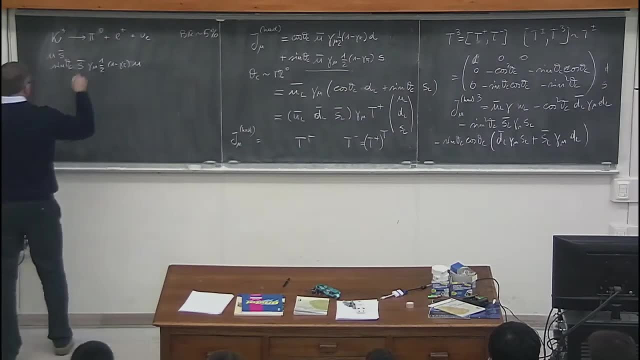 But if I have a term like this in the Haddon current, I can imagine that the same, the decay of the same particle, can take place like this. And this decay process is given by the replacement of the S bar quark By a D quark, because the pi plus is U D bar. 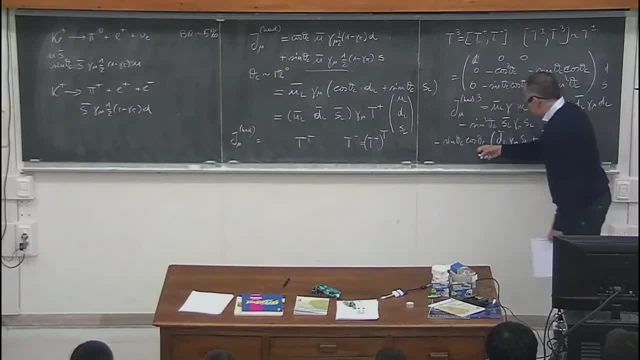 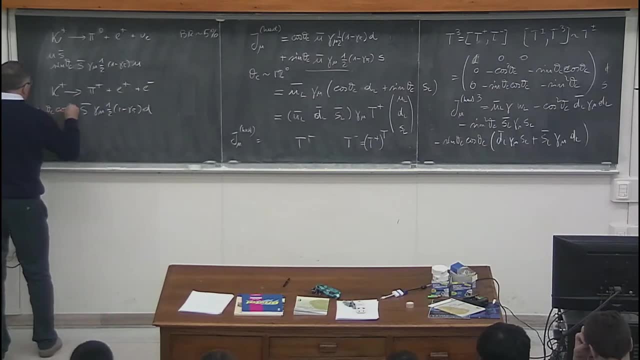 And the weight for this is sine theta Kb, cosine theta Kb And the leptonic part of the Lagrangian density is essentially the same. The only difference is that here you have a charged lepton, Here you have neutral Neutral lepton, but this makes essentially no difference. 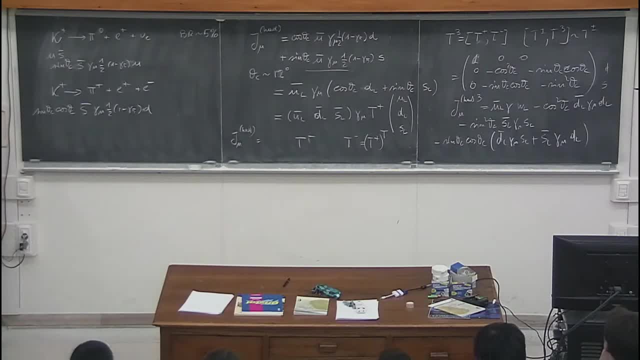 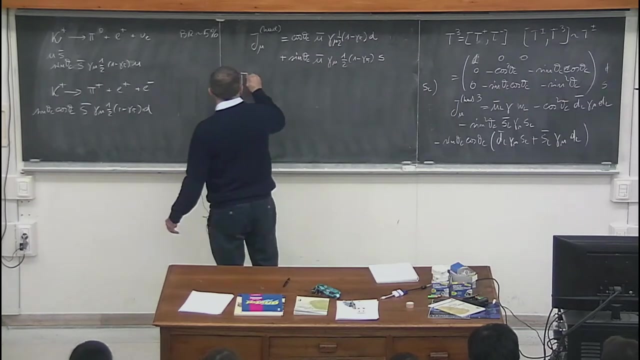 because the mass of the electron is very small compared to the mass of the K meson, which is around 500 GeV. So if you have this flavor-changing neutral current term around, what you would predict is that the ratio between the width for the decay process. 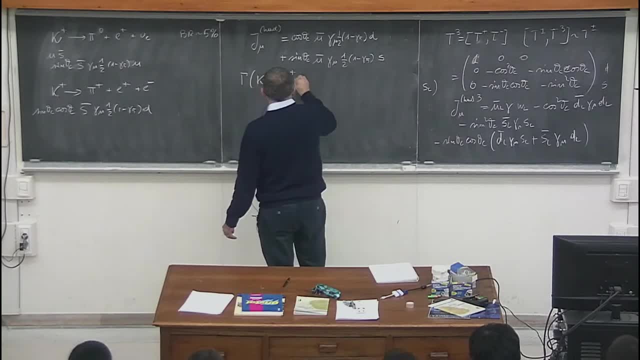 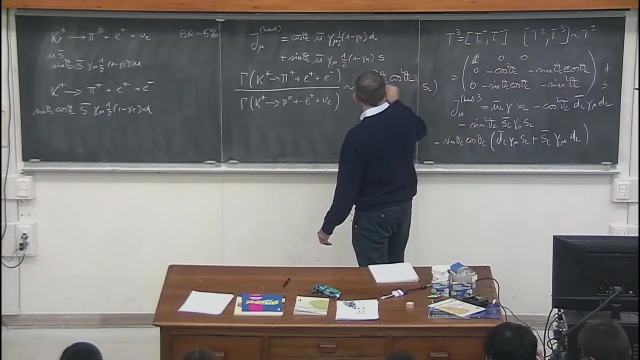 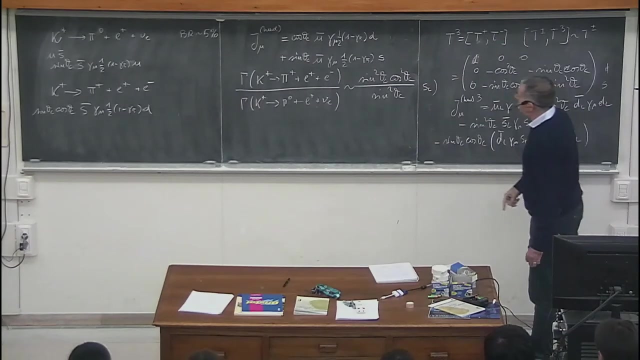 that's pi plus plus E plus plus E minus, divided by the width for K plus into pi zero. E plus neutrino should be of the order of the square E plus neutrino of sine square theta cabibbo cos square theta cabibbo. 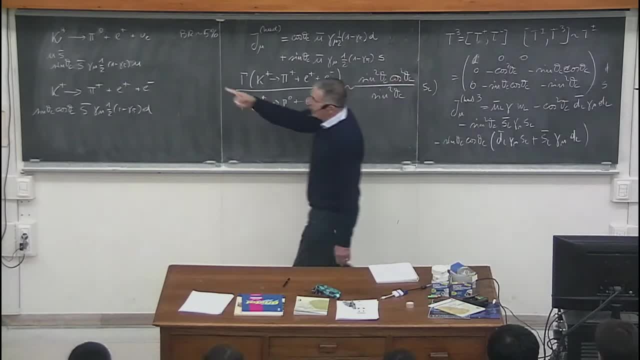 divided by sine square theta cabibbo. The square is because this is the amplitude and the weight is proportional to the square of the amplitude. All the rest is essentially the same: phase-space factors, matrix elements. There is essentially no difference. So this is what I expect. 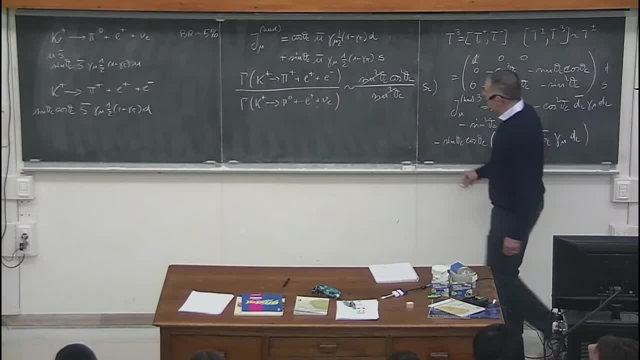 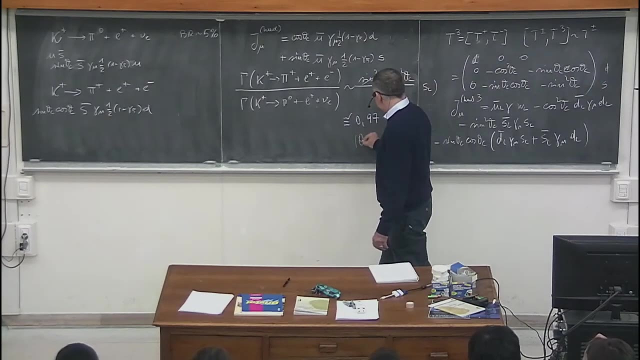 And since theta cabibbo is a small angle, this is close to one. something like this. this is what I expect from this construction. What I measure is 10 to minus 5.. This flavor-changing, neutral, current process. you see that in the Hadron sector. 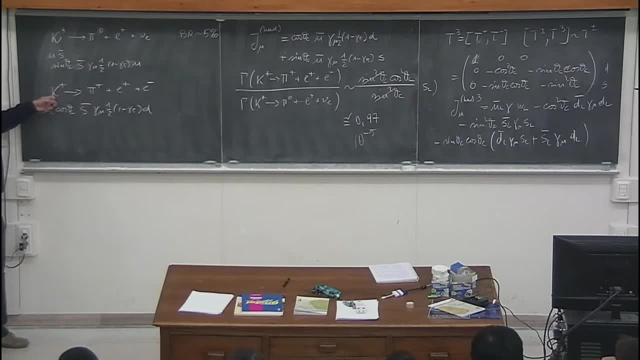 there is no charge change but the flavor changes. So this is flavor-changing neutral current process. It is measured, It has a very small branching ratio and the ratio between the two is of order 10 to minus 5.. So this is an example of the suppression. 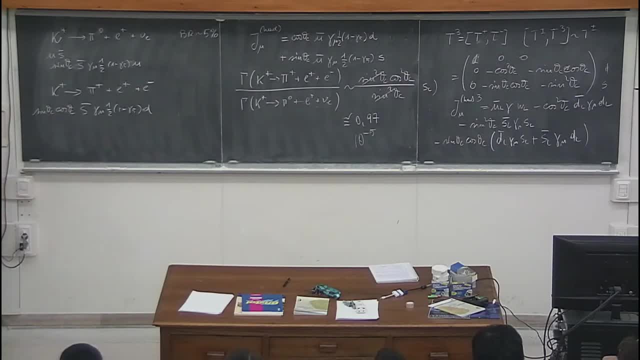 of flavor-changing neutral current effects with respect to flavor-changing charge current effects like this one. So this is, This must be suppressed somehow. What we did is not correct And there is a very well-known solution which I want to show you. 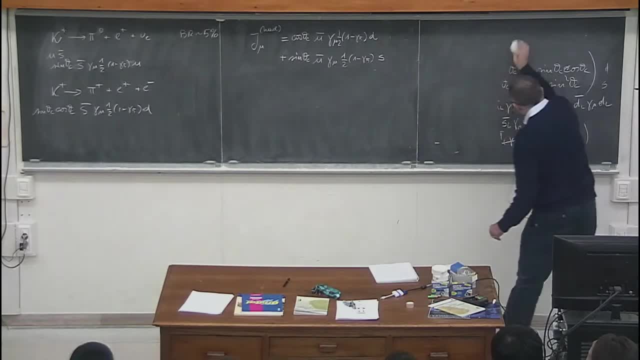 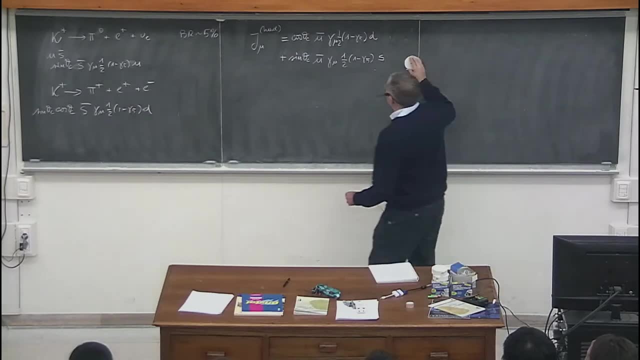 So this doesn't work. Let me write this term here on the same line: plus sine theta: cabibbo u bar gamma mu: 1 half 1 minus gamma 5. The S quark? The solution was proposed by Glashow again. 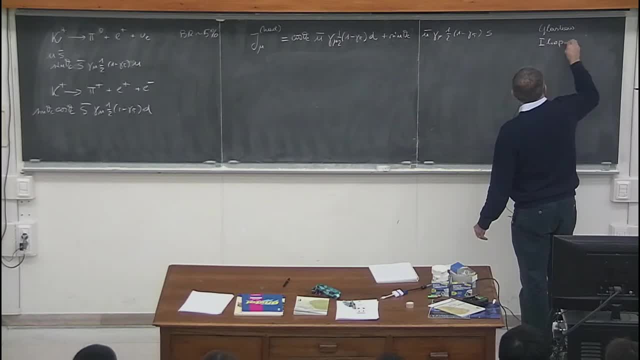 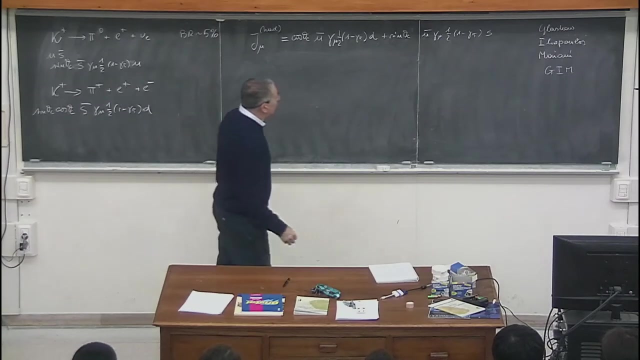 Gianni Liopoulos and Luciano Maiani, And what I'm going to tell you about is usually referred to as the GIM mechanism of suppression of flavor-changing neutral current, And the idea is the following: These three guys suggested that there is a fourth quark. 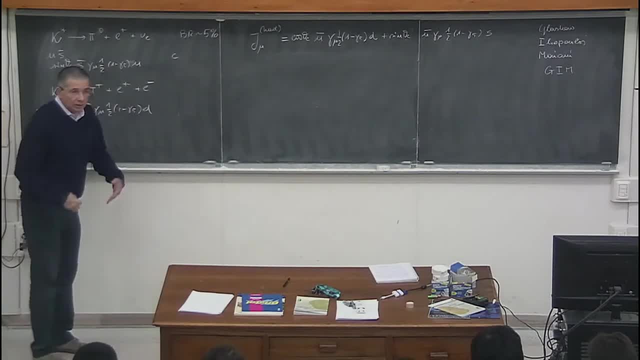 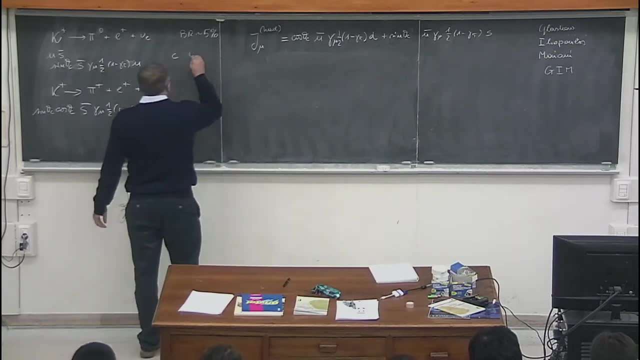 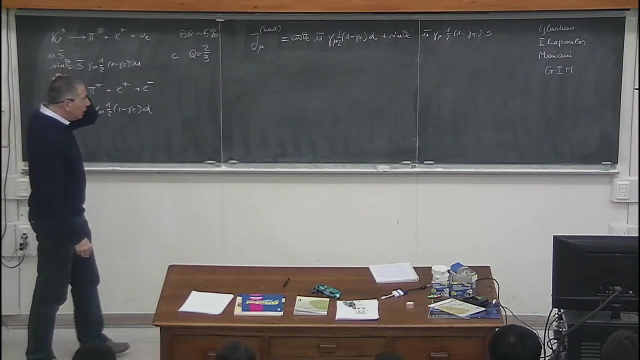 which they call a charm quark. There is a new flavor to be included in the game And this new flavor has The same electric charge as the up quark. It is similar to the up quark And they assumed that the interaction of the C quark 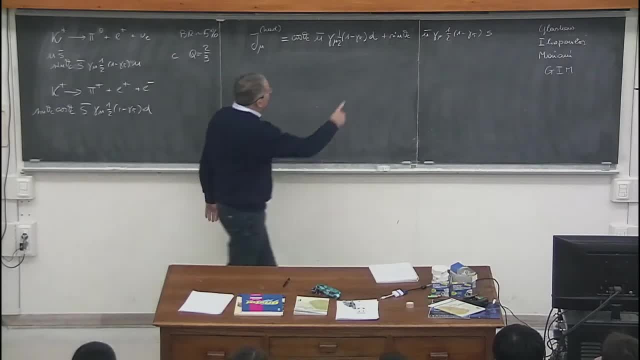 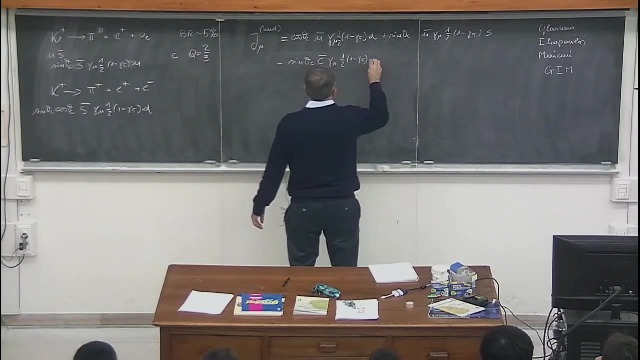 of this newly introduced C quark with DNS is like this: Minus sine theta cabibbo c bar gamma mu 1 half minus gamma 5 d. Plus cosine theta cabibbo c bar gamma mu 1 half 1 minus gamma 5 S. 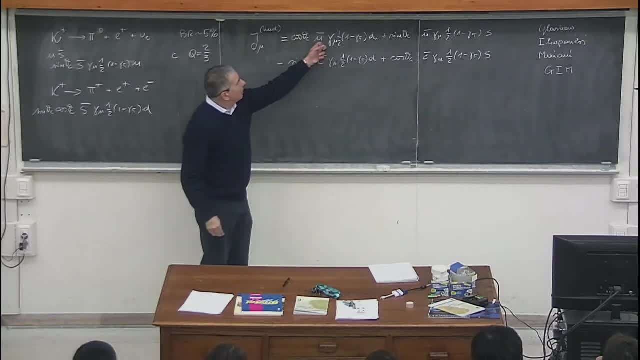 So, while the up quark is mainly coupled to D and weakly coupled to S, the opposite is true for the charm quark: It is only slightly coupled to the down quark and it is strongly coupled to S. There is no sign. 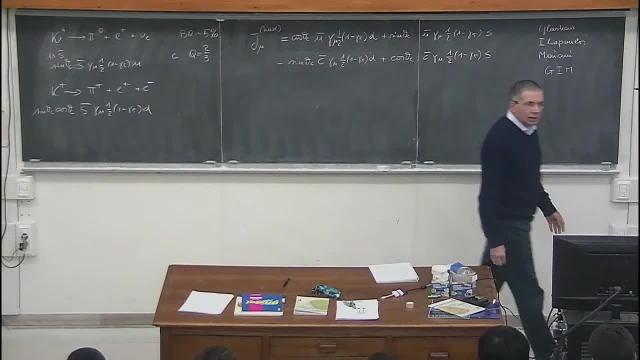 We are talking about mid-70s, 1973, 74. There was no sign, There was no need to introduce a new family of hadrons phenomenologically, But they just used the usual trick. They just assumed that the charm quark is so heavy. 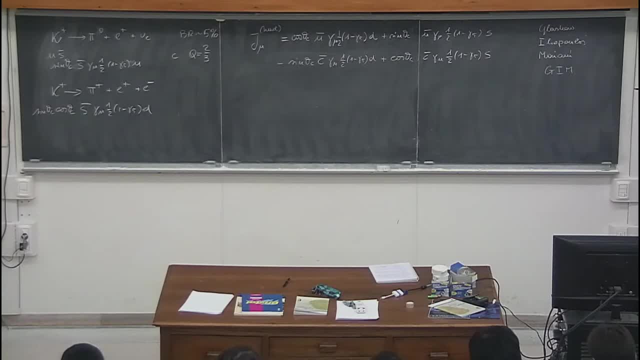 that present-day experiments in 1974 were not able to produce charm hadrons. So there is no problem, You just push Towards high masses what you don't see, But still the charm quark is there, they said. And it is coupled like this: 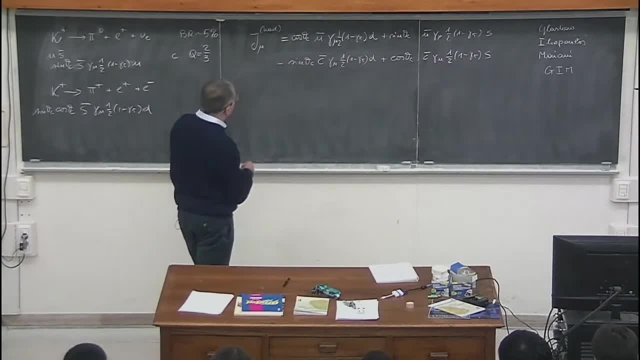 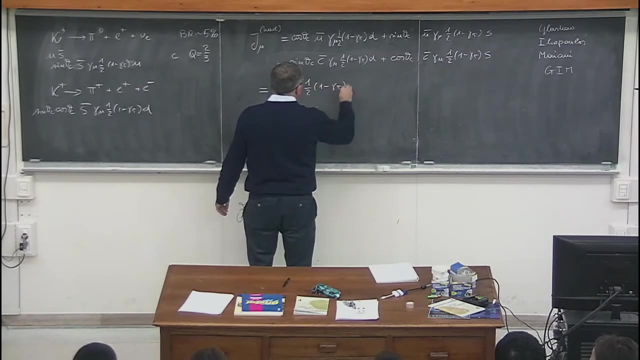 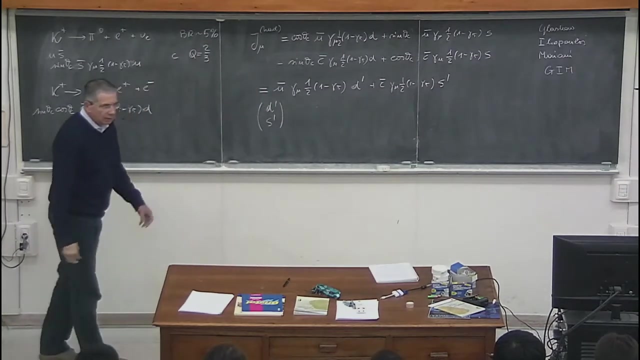 And this current here can be written in the following form: U bar gamma mu 1 half minus 1 minus gamma 5 d D prime plus C bar gamma mu 1 half 1 minus gamma 5 S prime. Well, D prime and S prime are not the original flavor quark fields. 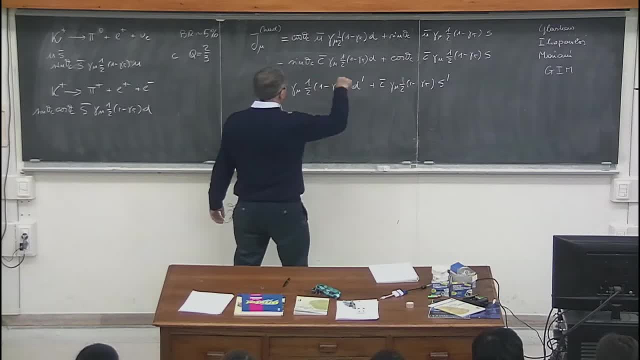 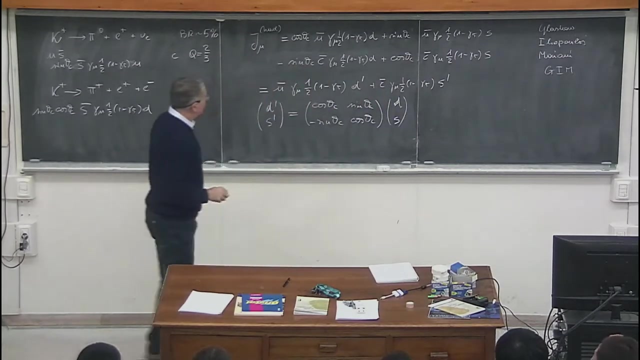 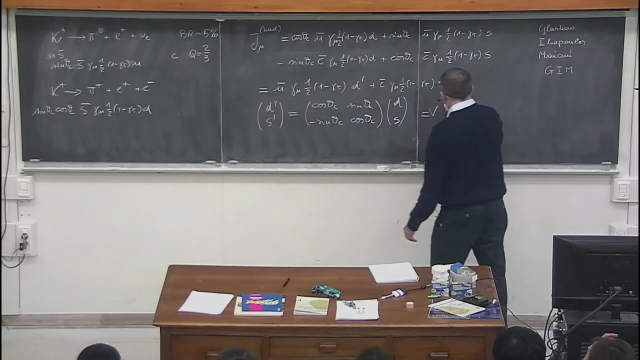 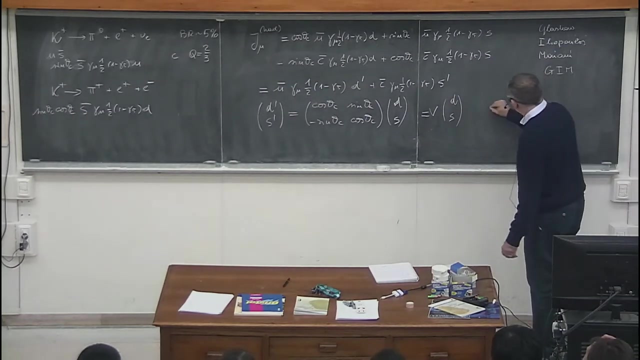 but are rotated with respect to them by a matrix which is again a rotation. So let's write the general reaction matrix. So if I do that, let me call this matrix V. This matrix V has the property of being an orthogonal matrix. 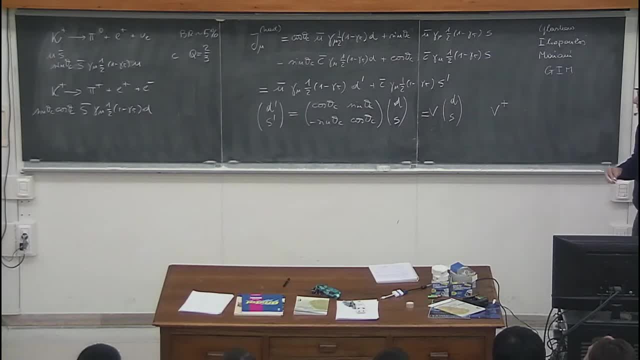 and if it were a complex matrix, it would be unitary. And if I do that, you immediately see that we are again in the same position as we were in the case of leptons, because this can be written like this: u-bar left, d-prime left, gamma, mu tau plus u-left, d-prime left plus c-bar left. 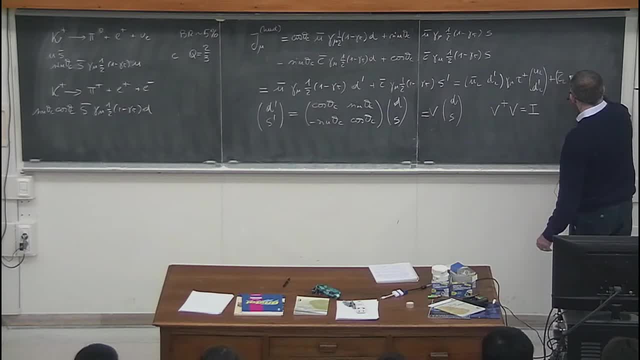 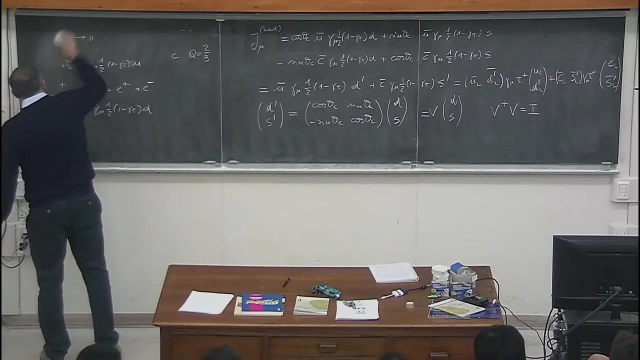 sorry, not enough here. c-bar left and s-prime bar left, gamma mu tau plus c-bar left, s-bar prime left. Sorry, Bar missing. Is that correct? No bar here. Okay, Why is this a solution to the neutral, flavor-changing neutral current problem? 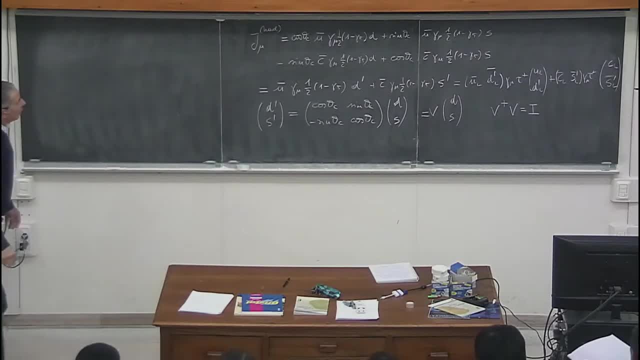 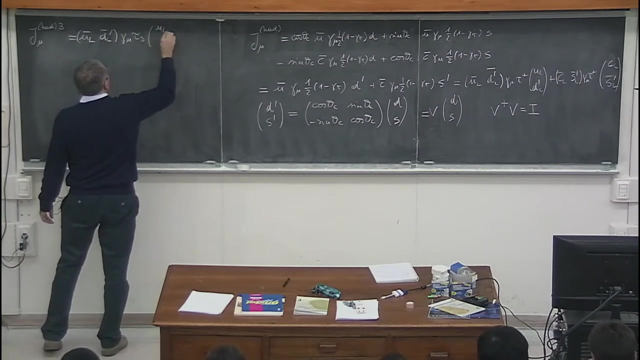 The reason is very easy. If I now compute j mu, hadronic 3, this is diagonal in u-d-prime and s-d-prime, so this is given by u-bar, u-bar, left, d-bar, left-prime, gamma mu, tau 3, u-left, d-left-prime. 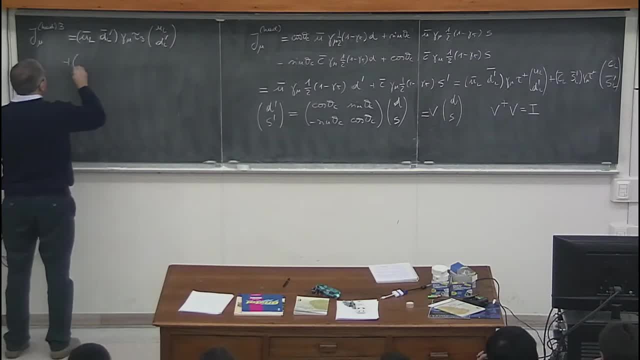 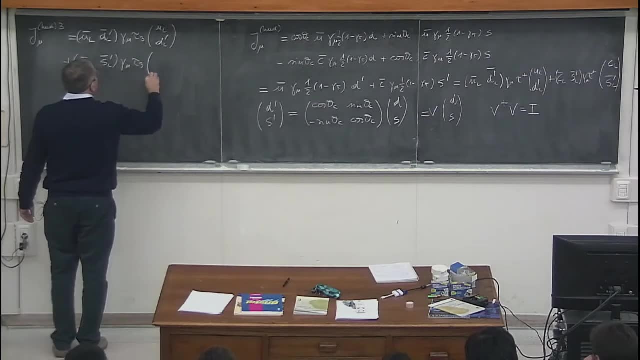 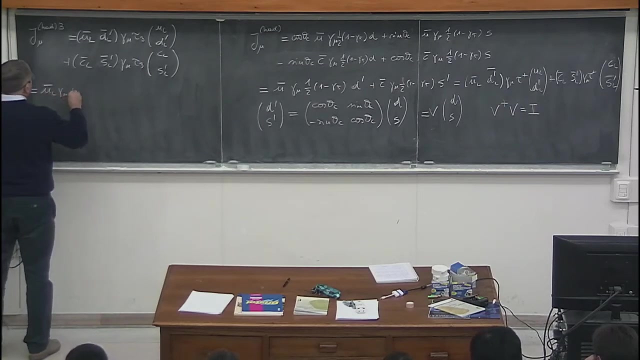 plus c-bar left, s-bar prime left, gamma mu, tau 3, c-left s-prime left, Which means u-bar left, gamma mu, u-left plus c-bar left, gamma mu, c-left. These are the terms corresponding to the first to the 1-1 entries of tau 3, in both terms. 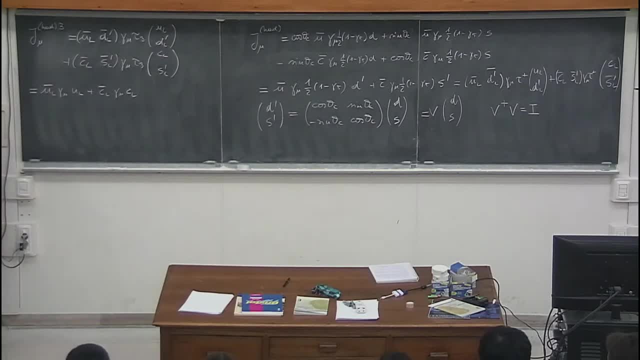 They are diagonal in the up quarks. Then you have terms with a minus sign in front, because the second entry of tau 3 has a minus sign. Yes, The negative is. the negative can be used to explain: like: no prime, no prime. 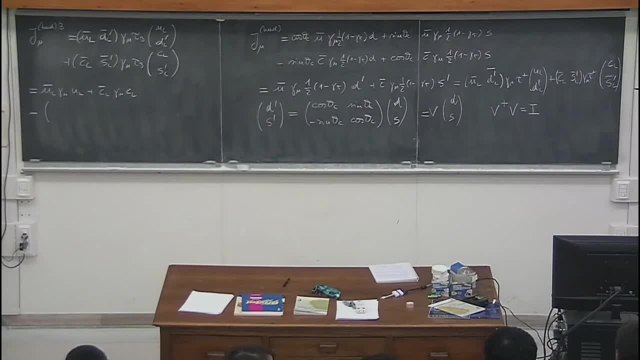 Yes, But now, why do I look at the video in this way? I mean, by the way, maybe it's because it's prime here. What's wrong with that? I mean, Let me finish, but maybe this answers your questions. 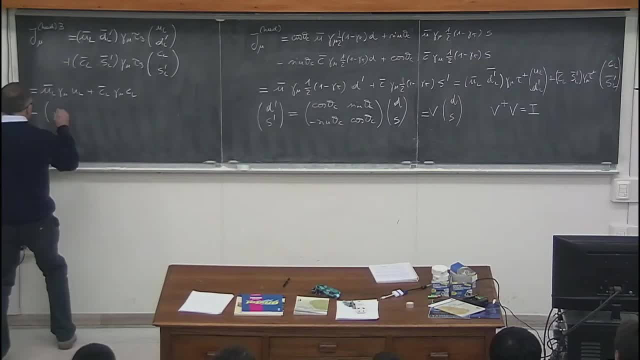 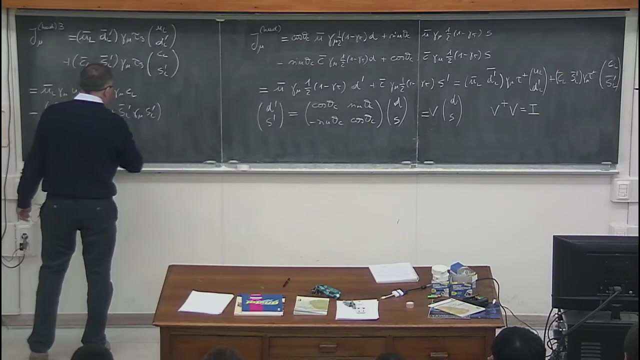 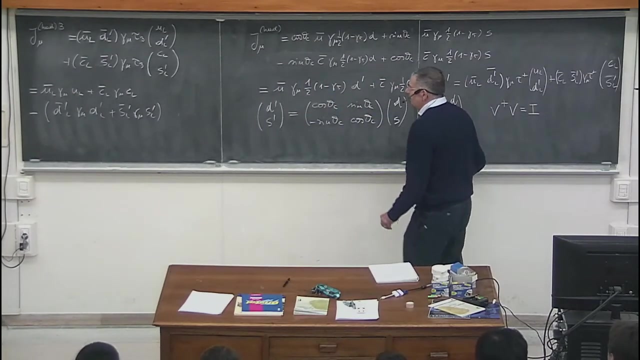 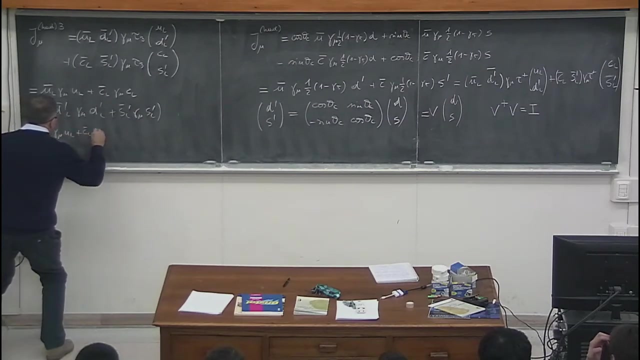 The second term here corresponds to down quark, so d prime left gamma, mu d prime left Plus s bar left prime gamma mu s left prime. But he doesn't like primes, so I get rid of primes. And right here This doesn't have primes, so it's fine. 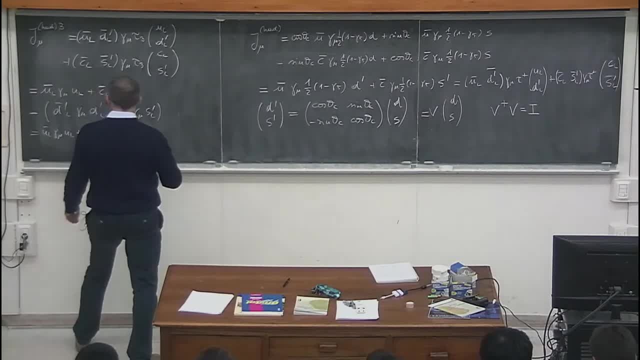 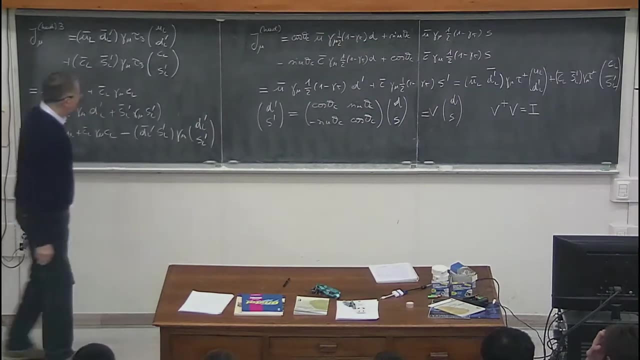 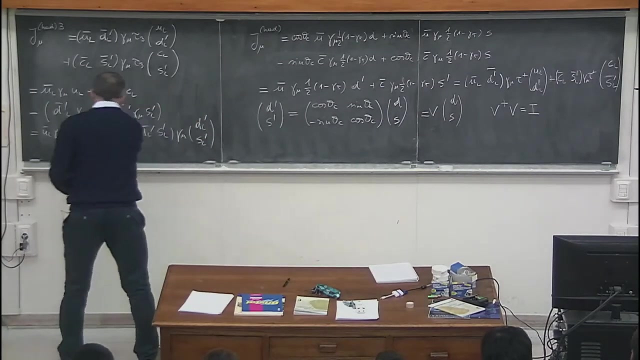 And this I can write like this: Minus d bar left, prime s left, prime gamma. mu d left, prime s left, prime. Okay, Just scalar product. This times this plus, this times this. But now I use This definition, This definition here: 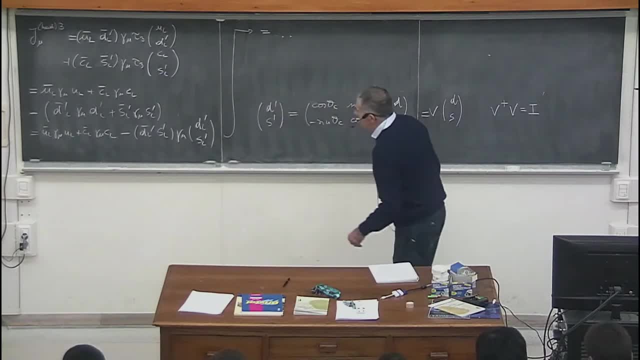 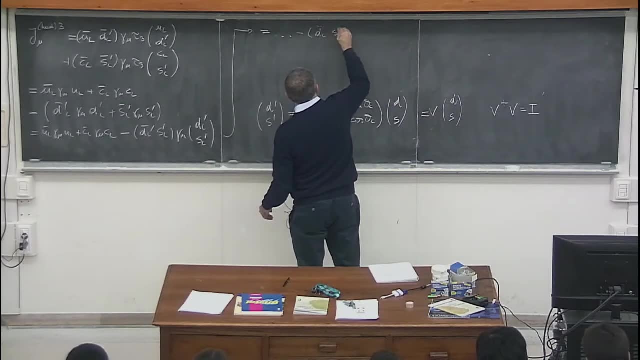 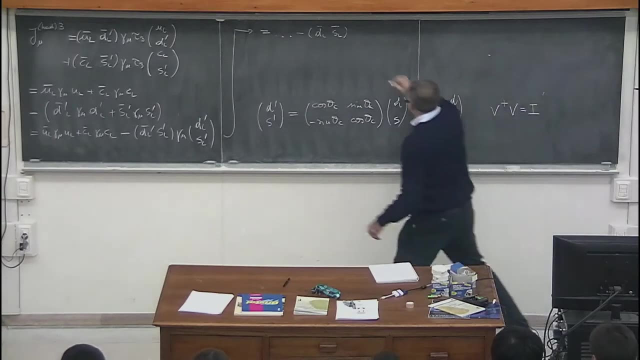 And I get- Let me omit the first two terms, which are already okay- Minus d bar left s bar left, Without primes v Permission conjugate Gamma mu v d left s left. But I choose, Actually, Luciano Maiani chose for me v to be an orthogonal matrix, a unitary matrix. 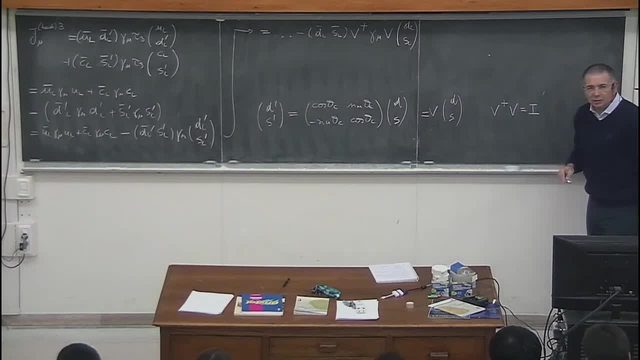 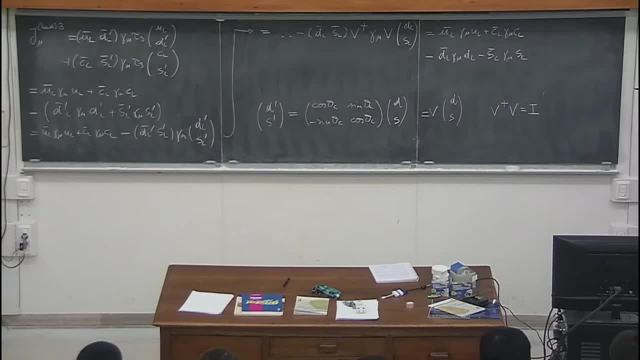 Okay, Is that what you were asking? So there is no trace of the mixing between the two down quarks in the neutral current because of the fact that we chose cleverly the structure of couplings of the charm quark. We don't see it, so we can do whatever we want. 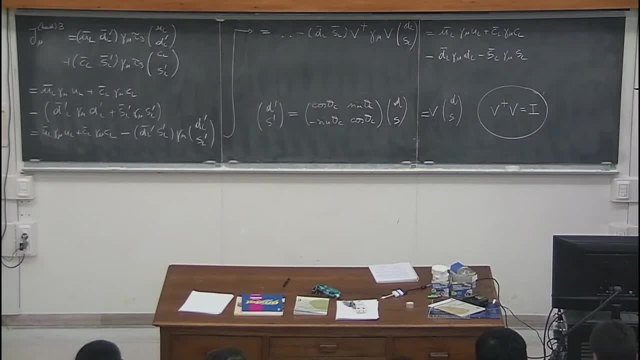 So this is the GIM mechanism, which requires the introduction of an as yet unobserved particle, the charm quark, but for the rest it's okay. It suppresses flavor-changing neutral current at the tree level. So this is what Glashow, Iliopoulos and Maiani suggested. 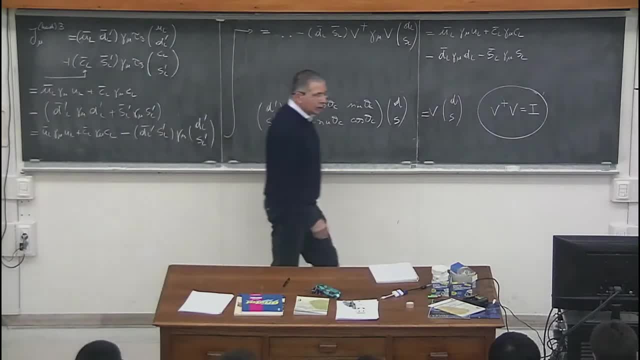 And in fact the charm quark was observed very soon. What was first observed is the resonance C bar C, which is called The J-ipsi particle in the J-A equal to one state is a vector particle. It was produced in E plus E minus collisions at MIT and at SLAC. 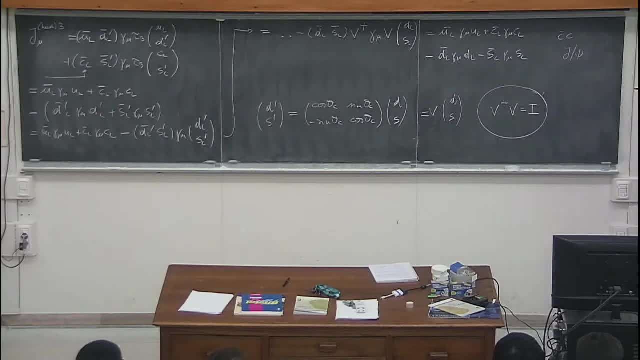 and immediately after that also in Frascati, here in Italy. This particle has a mass. the mass of the J-ipsi is around 3 GV. 3 GV is actually an enormous number For the scale of energies available at that time. 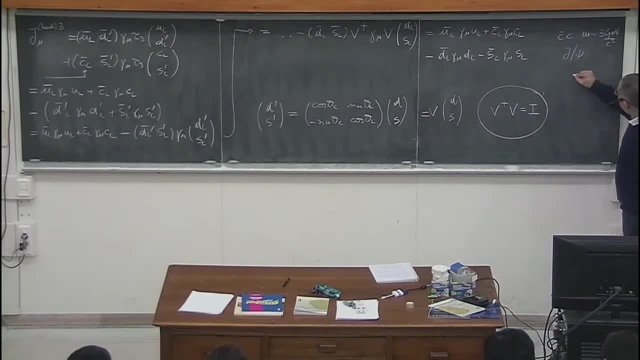 And this is related to the fact that the charm quark has a mass of over 1.5, 1.3 GV, which was indeed much larger than the masses of up-and-down quarks and also much larger than the mass of the strange quark. 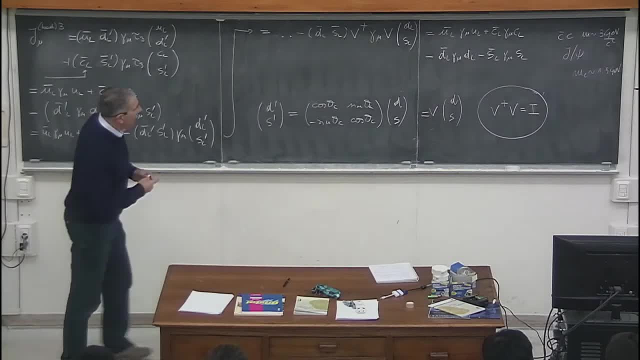 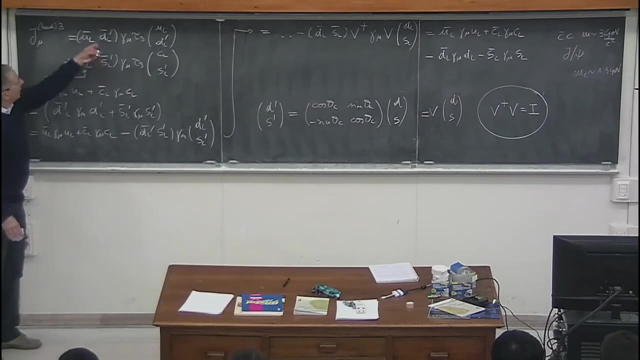 Anyway, we will talk about flavor again later in much more detail, but I just wanted to show you this historical path which led to the idea that quarks must come in doublets, and mixing between different doublets is not only possible but also required by phenomenology. 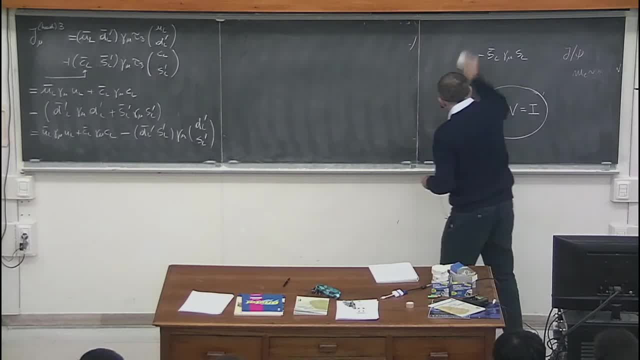 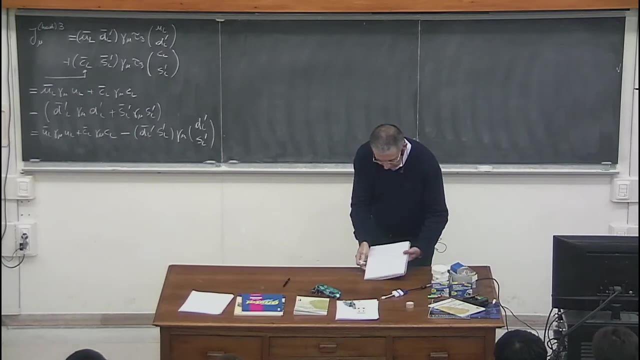 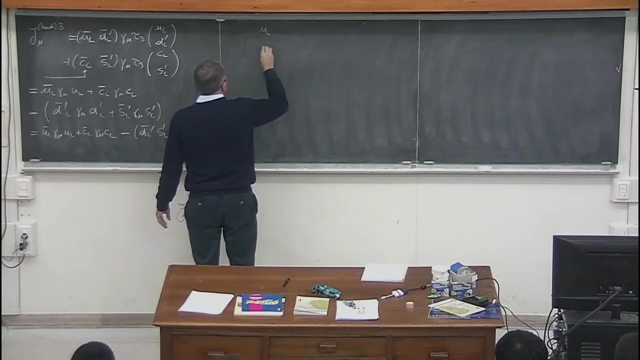 So we have nothing else to do. essentially, We have a structure which is very similar to the structure of leptons. There is a doublet of leptens. There is a doublet of left-handed d-quarks in the first generation. 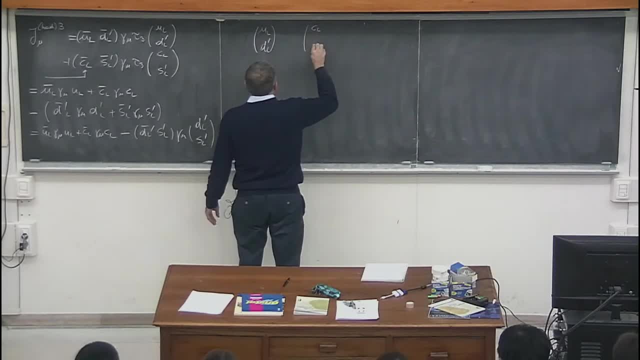 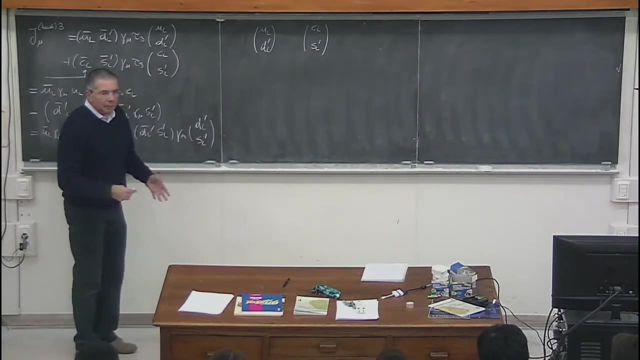 There is a doublet of left-handed quarks in the second generation, And the structure can be replicated as many times as we like, provided that the down component of this doublet are mixed by means of a unitary matrix which I call P. 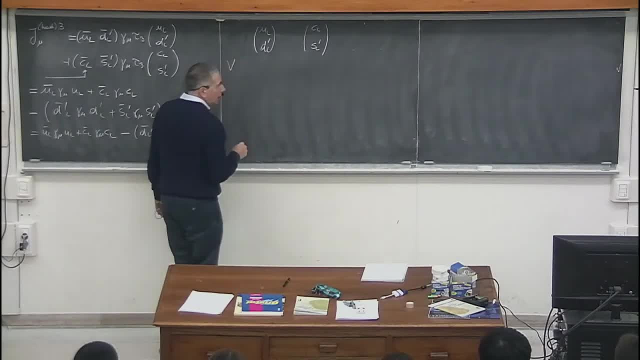 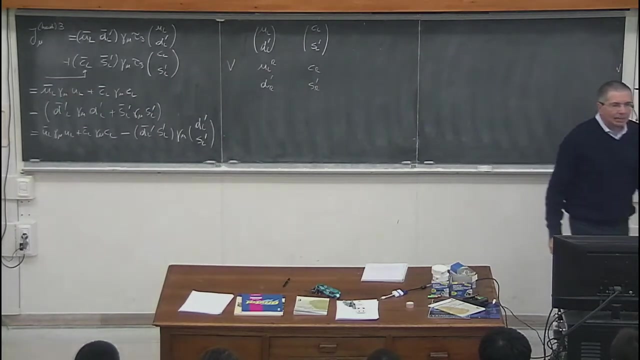 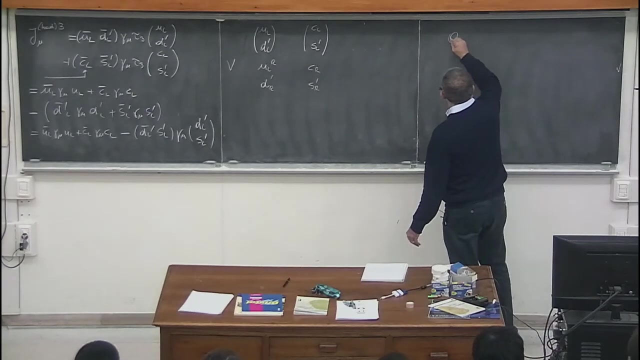 And the right-handed components are again placed into singlets of S-U-2.. And the hypercharged quantum number. if we repeat exactly the same argument which we worked out in the case of leptons, we would end up with a relation which is the same. 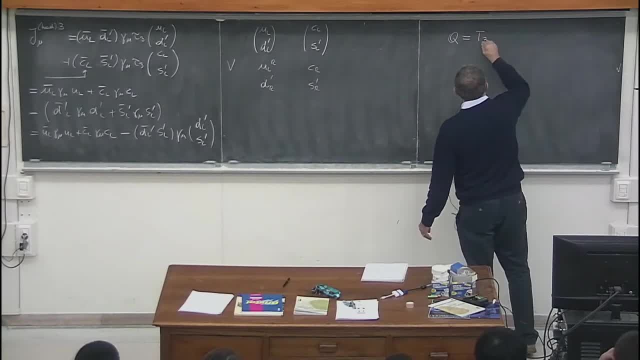 that we get for leptons. Q equals T3 plus the hypercharge divided by 2.. Or, if you like, hypercharge to Q minus T3.. The difference here is that down-type quarks- now Sorry, Up-type quarks- do not have zero hypercharges. 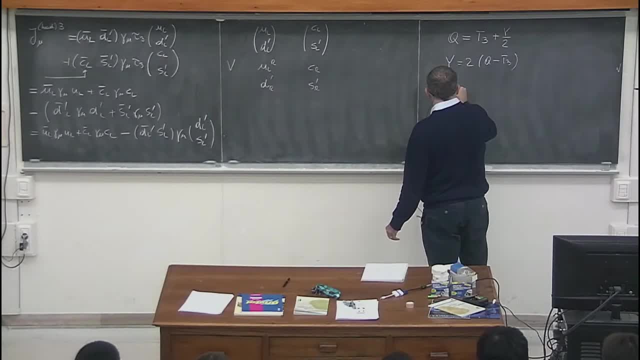 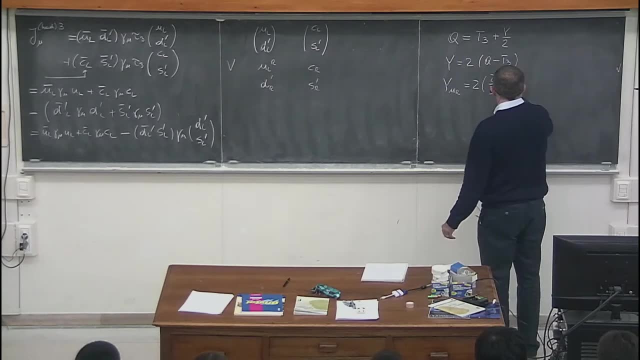 The hypercharge of, for example, U-R is twice 2-3rd minus zero. The zero here is because right-handed particles are singlets of S-U-2. And this is different from zero, which is a difference with respect to the case of leptons. 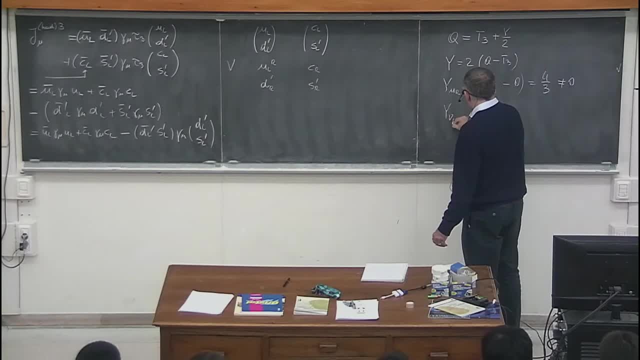 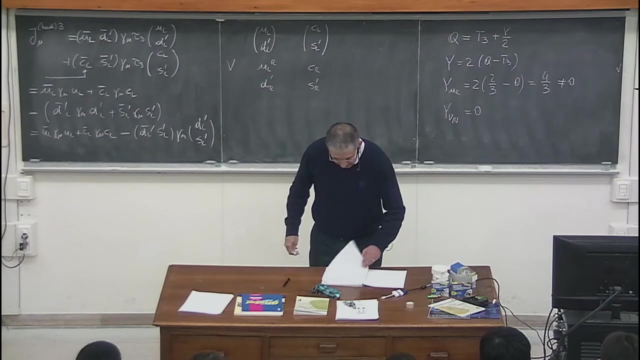 where the hypercharge of right-handed neutrinos is zero, And this will lead to differences in the case of hadrons, which we will discuss in great detail later. I think this is all I wanted to say about the massless structure of hadrons. 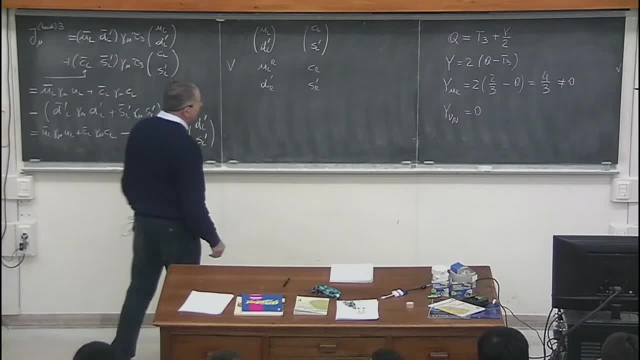 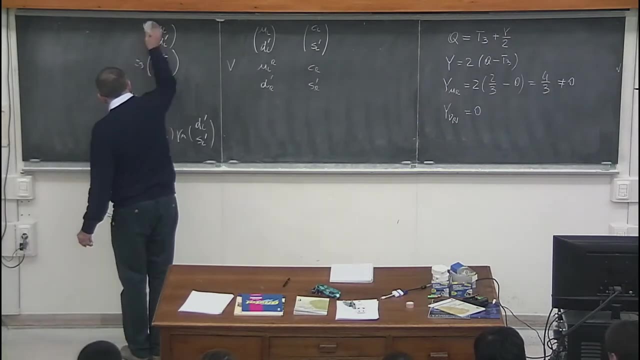 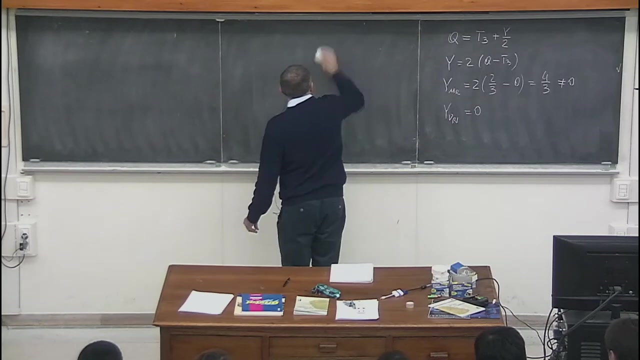 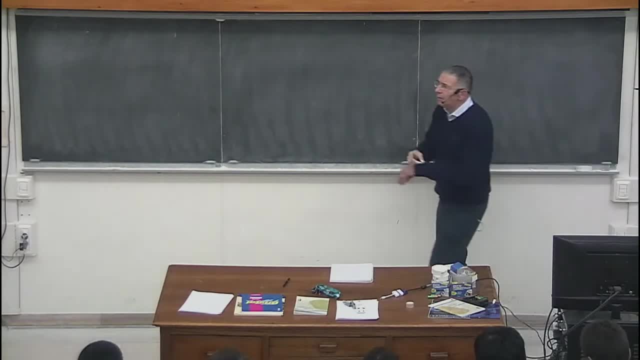 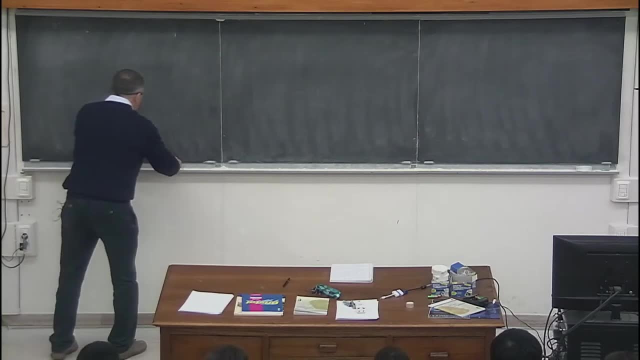 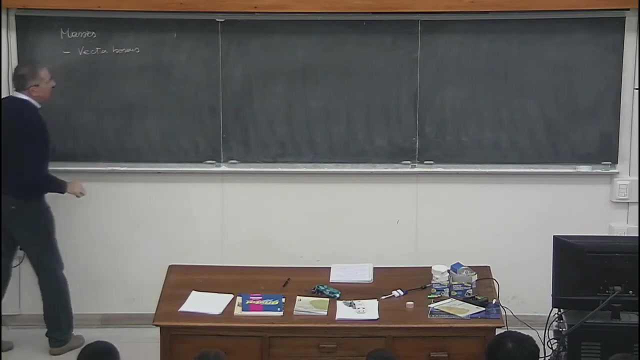 Thank you. Let me just introduce the problem and then probably we make a stop for five-ten minutes And then we come back to the lecture. The problem is the following: There is a problem with vector bosons and, as you already know, 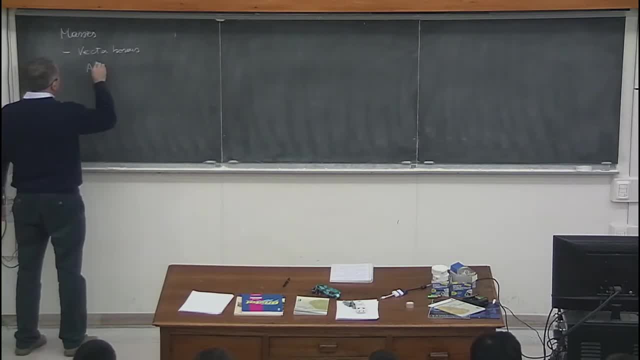 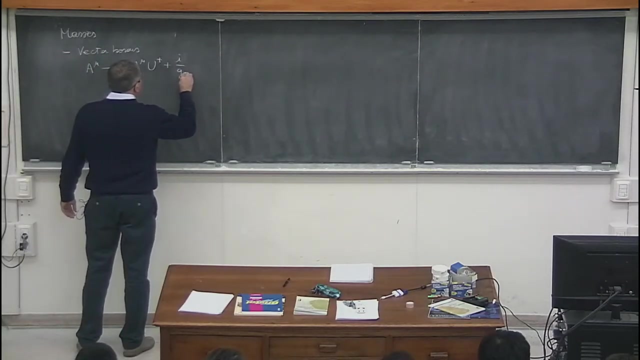 in the Young-Mills construction Vector bosons are transformed under the action of the gauge group like this: u a mu u dagger, where u is a matrix belonging to the gauge group plus i over g? u d mu u dagger. 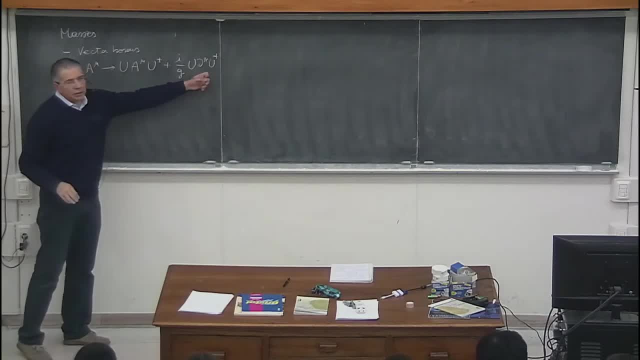 And this second term is generally non-zero because u is assumed to be a local transformation. in the case of gauge theories, And if you have a situation in which vector fields transform like this, it is clear that mass terms m, square, a, mu, a, mu. 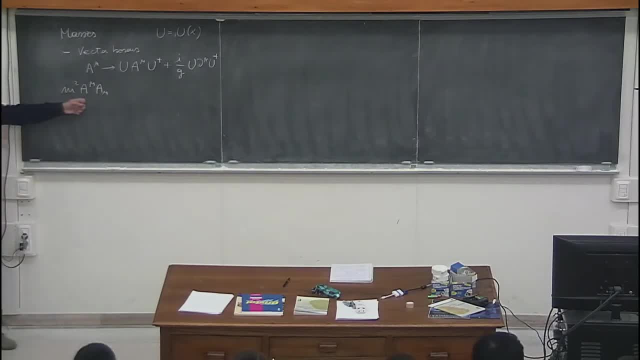 what we call a mass term in quantum field theory is a bilinear term in the Lagrangian, which does not contain derivatives. So this is the only mass term we can build out of a vector field which is dimension four and Lorentz invariant. 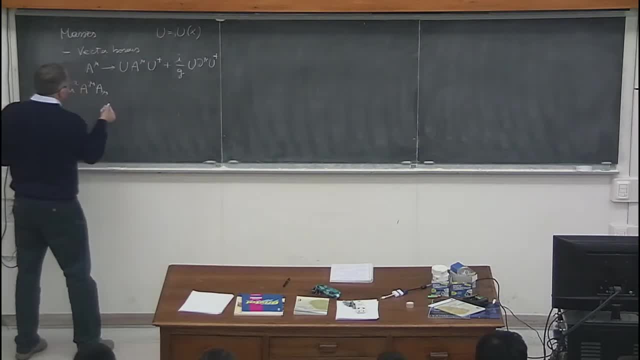 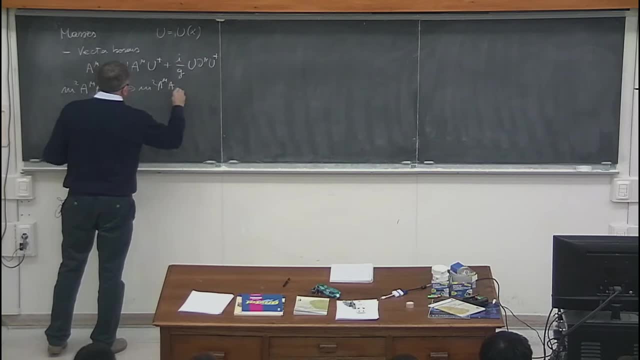 So m square a mu. a mu is not invariant. clearly, it transforms itself, plus something. this is easily seen in the Abelian case, where a mu from this transformation lose becomes a mu into a mu, plus the divergence of a scalar function. 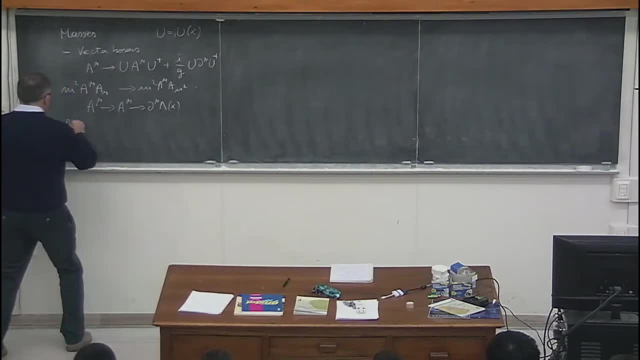 the parameter of the transformation, which means that A mu A mu goes into A mu A mu plus twice A mu d mu. lambda plus terms of order, lambda squared. So a mass term is forbidden by gauge invariance. There is no way out. 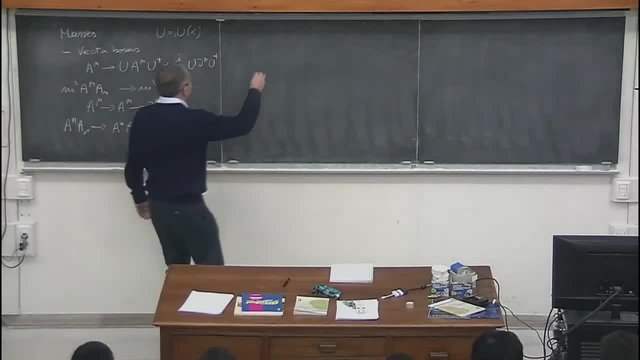 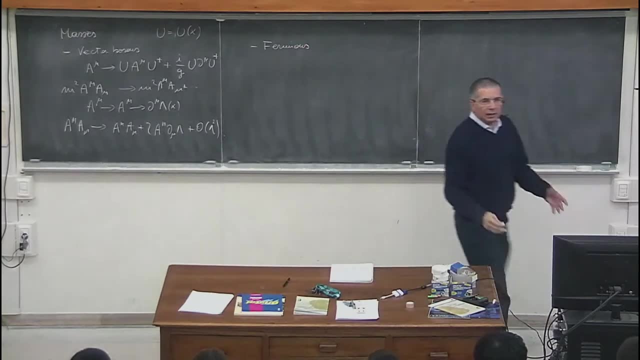 But there is a problem also with fermions in the case of the standard model, Because the standard model, the theory we are constructing together, is what is usually called a chiral theory. A chiral theory is a theory based on an invariance property. 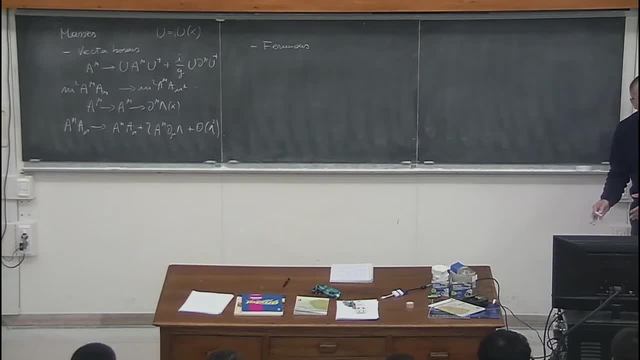 which treats in a different way left-handed component and right-handed component of a Dirac field. So in this case, So a mass term for a fermion, which is usually written like this: a Dirac mass term, not talking about Majorana mass term for the moment. 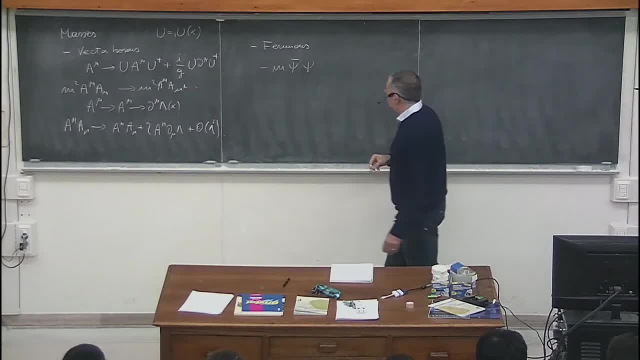 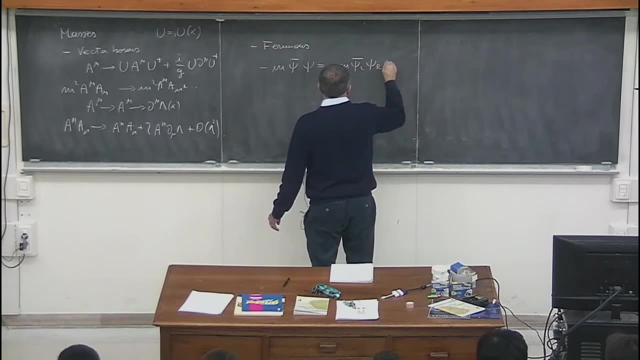 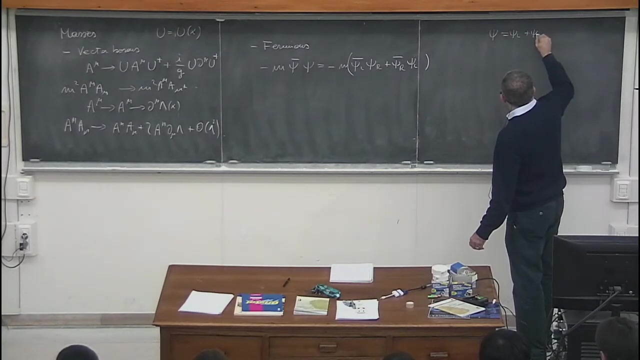 Dirac mass term is like this for a given fermion, psi, which can be written like minus n times this combination, This combination: if you decompose psi into the sum psi left plus psi right, then you easily discover that the diagonal terms are zero. 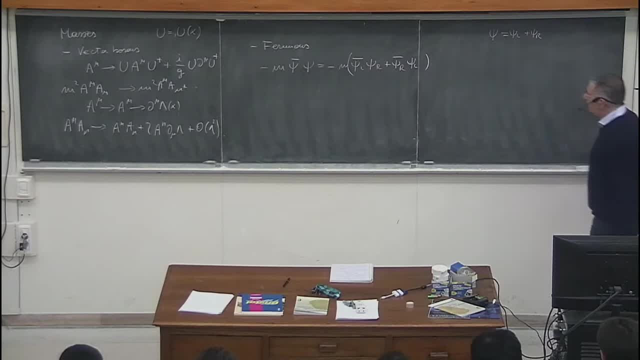 because of properties of gamma 5.. So you are only left with the mixing, the term which makes the right component and the left component of the Dirac field. And if you have a chiral theory, a chiral theory is one which transforms. 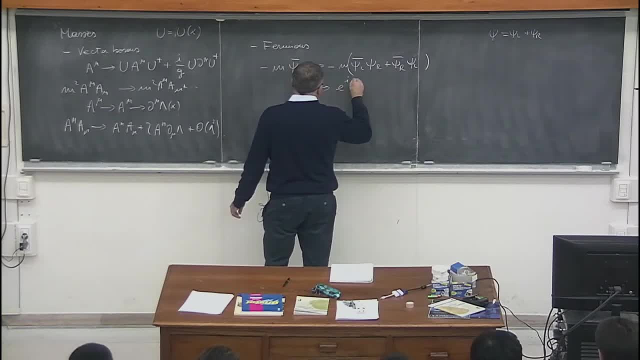 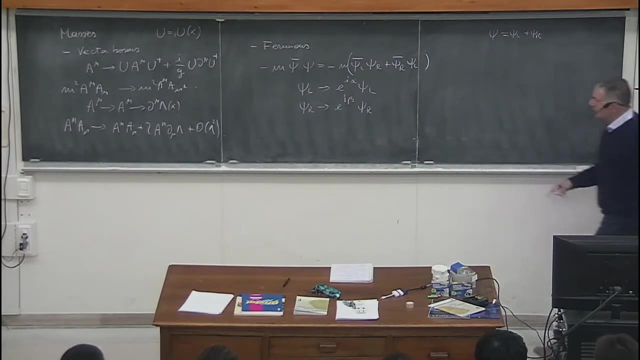 for example, the left-handed component into itself times a phase and the right-handed component into itself times a different phase, which, in the special case of the standard model, is zero. These are singlets under the action of SU and this is not invariant. 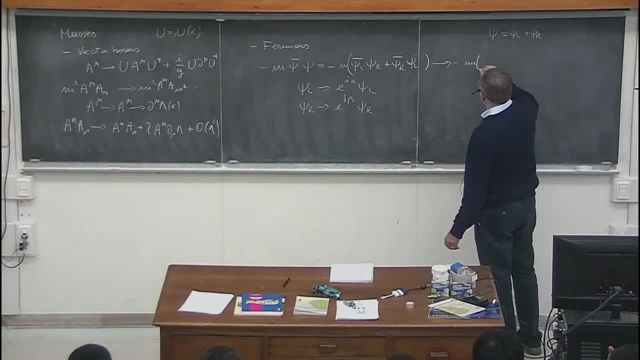 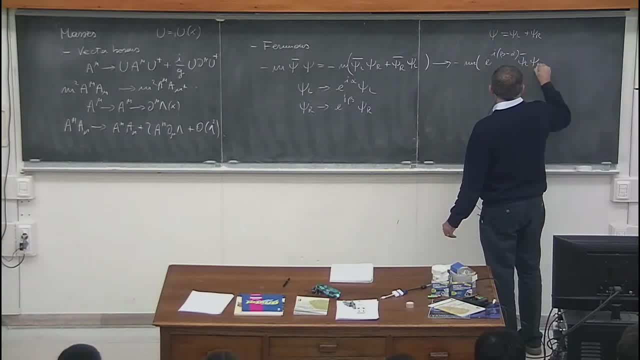 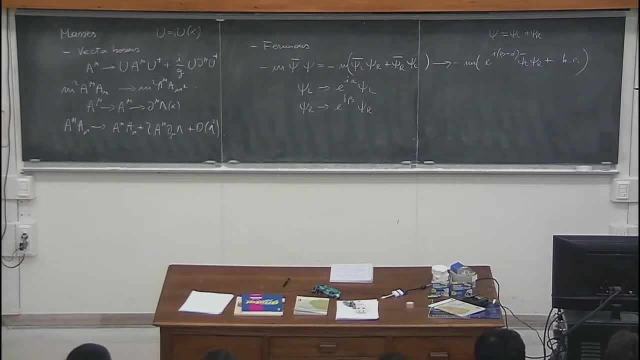 So in the case of the chiral theory also, fermion masses are forbidden. But we know we need both. We need mass for the vector bosons because the weak interactions are short range, and we obviously need masses for the electron, for the muon, for the up quark, for the top quark. 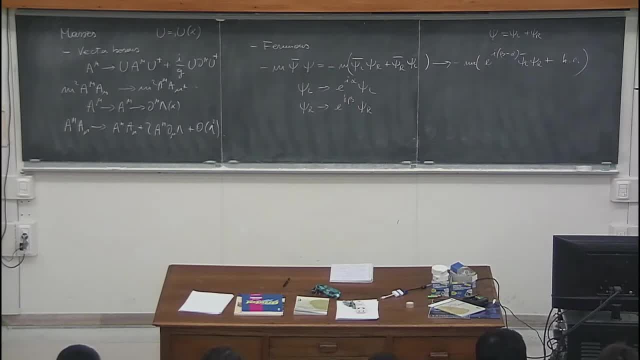 We need a very heavy mass. So we have to find out the way out of this problem, and the way out is something you heard about a little bit yesterday, but I will talk about that in much more detail. So we stop for a while maybe. 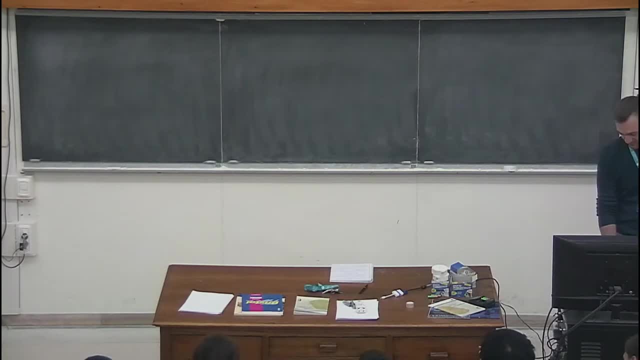 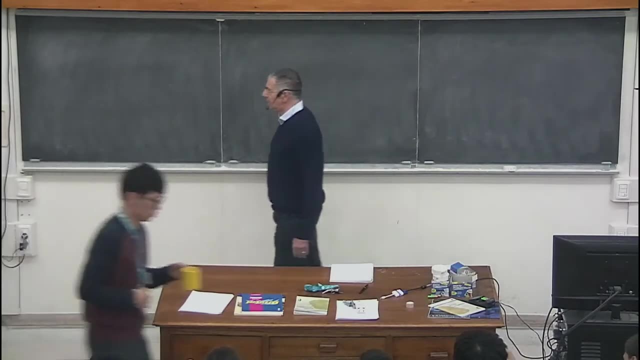 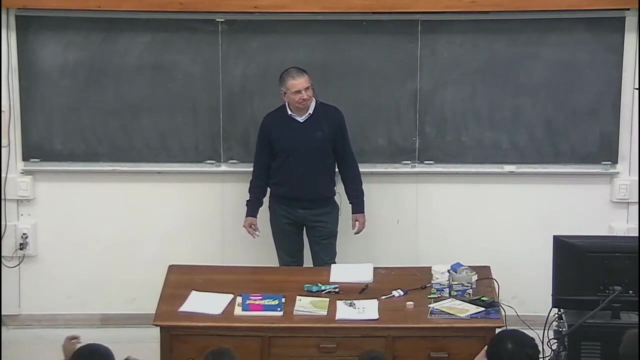 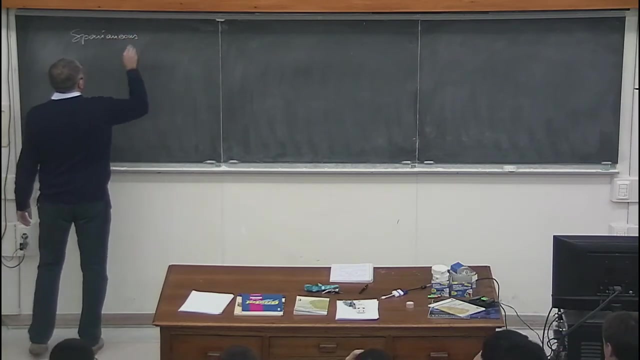 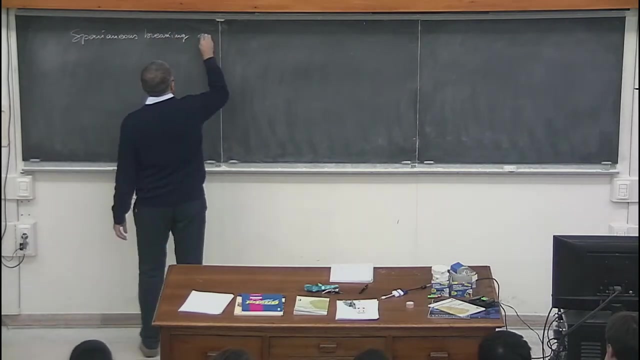 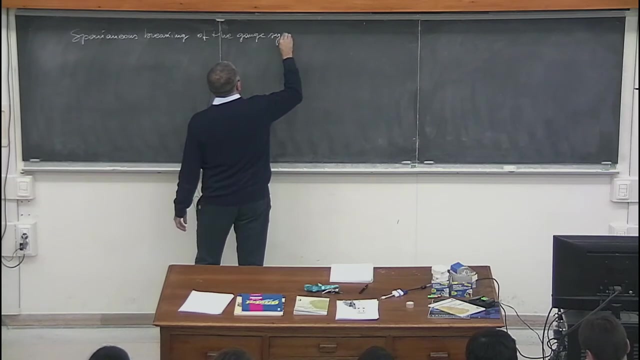 and we start in 10 minutes with this problem. Okay, Wait for the last arrivals. Okay, What we need is spontaneous breaking of the gauge symmetry, Which is an unfortunate name. as you probably already know, The gauge symmetry is not actually broken. 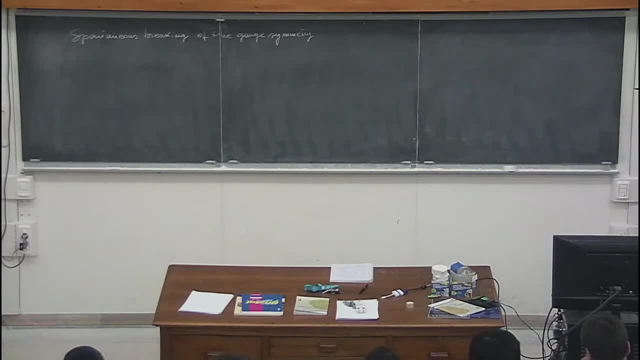 We don't want to break the gauge symmetry, because gauge symmetry is what guarantees that the theory is unitary and renormalizable. so this is not what we want And in fact we will not break the symmetry, We will just realize it in a slightly different way. 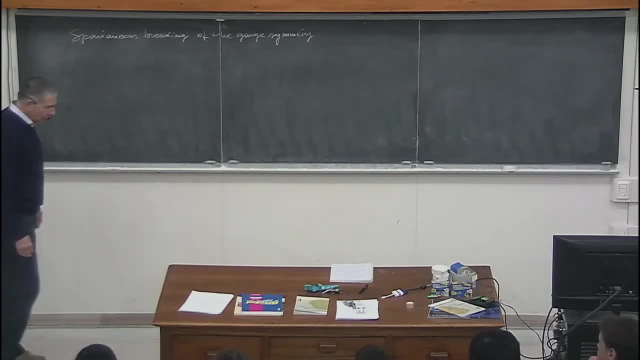 I will show you how the spontaneous breaking of the gauge symmetry mechanism works in a simple case. Then we will extend it to the standard model. The extension is rather straightforward, And the simple case which I will talk about is what is usually called scalar QED. 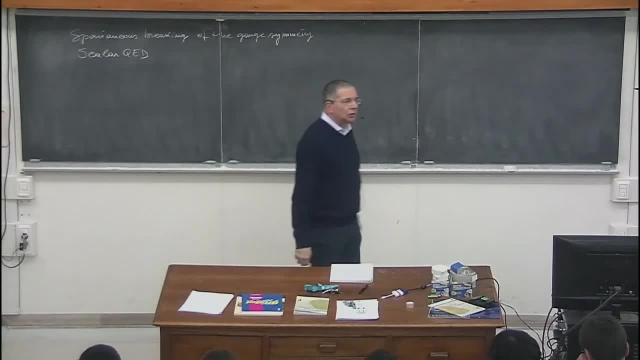 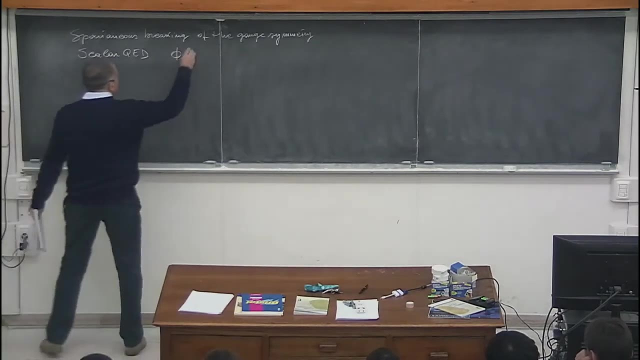 Scalar QED is quantum electrodynamics for one single charged, complex scalar field. Why a scalar field? We will see in a moment. So what is scalar QED is very simple. I have a charged scalar field, phi of x, And the Lagrangian density is: 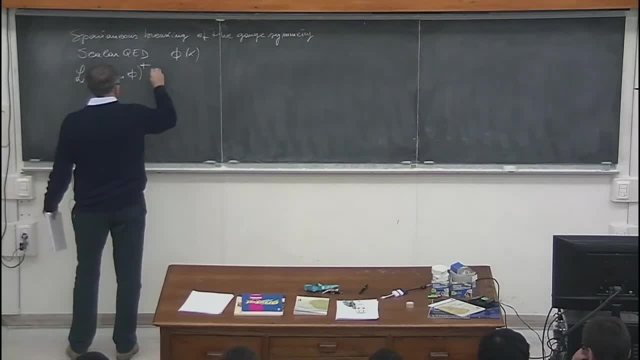 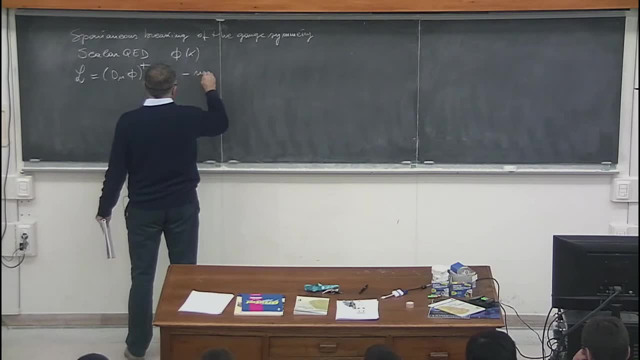 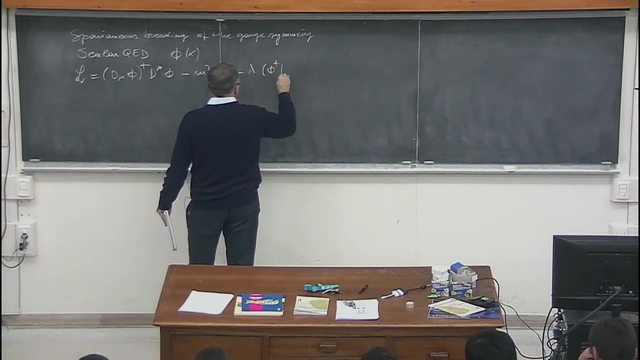 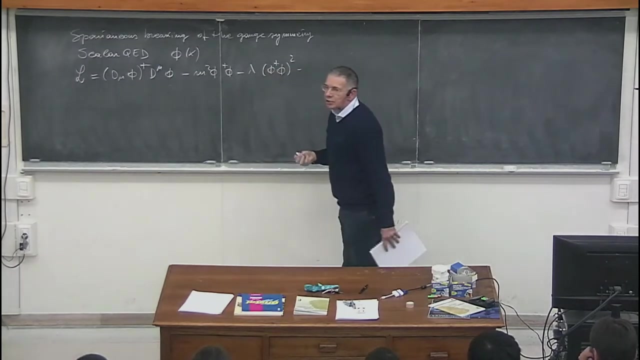 d mu phi Hermitian conjugate: d mu phi Minus. m squared phi dagger phi minus. lambda phi dagger phi squared Minus. let me use Feynman gauge. In the Feynman gauge the free field Lagrangian for the electromagnetic field is minus one half d mu a nu. d mu a nu. 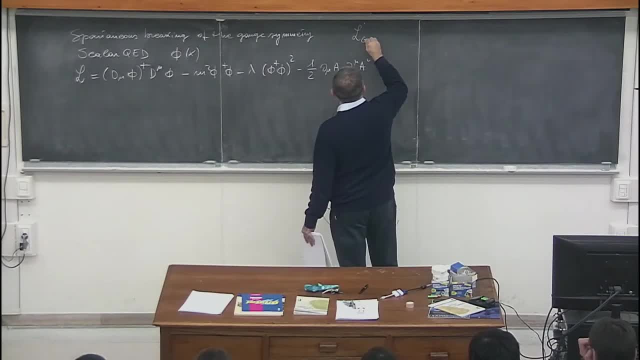 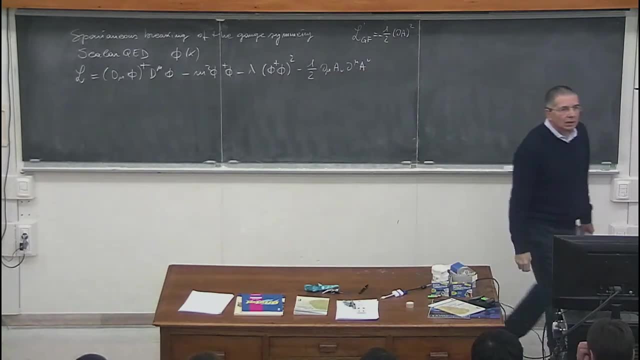 The Feynman gauge means that the gauge fixing term is equal to minus one half d mu a mu squared. I would take a few lectures to tell you something about gauge fixing. I assume you more or less know what it means. But with this gauge fixing, Lagrangian density. 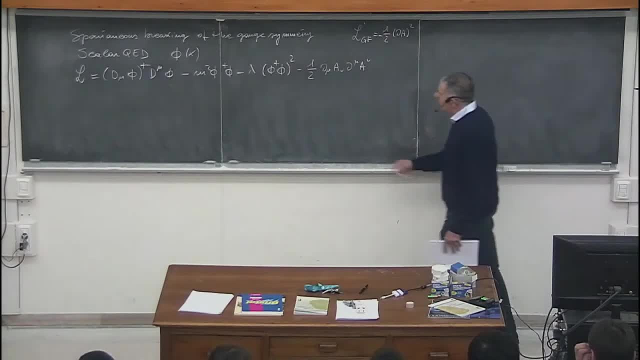 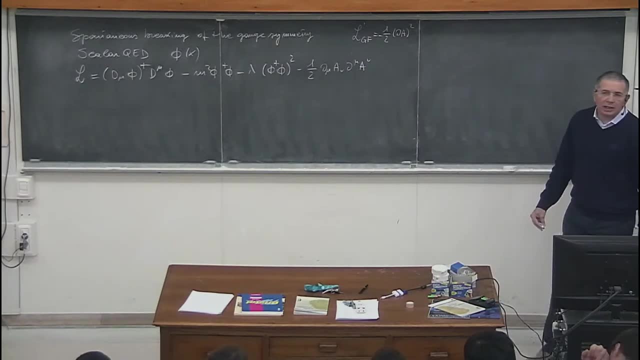 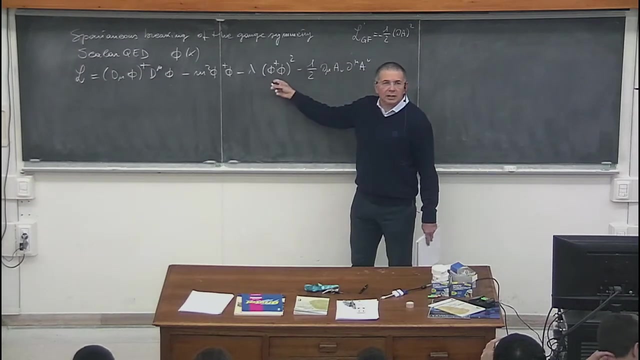 for scalar QEDs like this. we have a scalar potential here, which means terms in the Lagrangian density which do not contain derivatives of the scalar field, And these terms contain up to the fourth power of the field, again by the criterion of renormalizability. 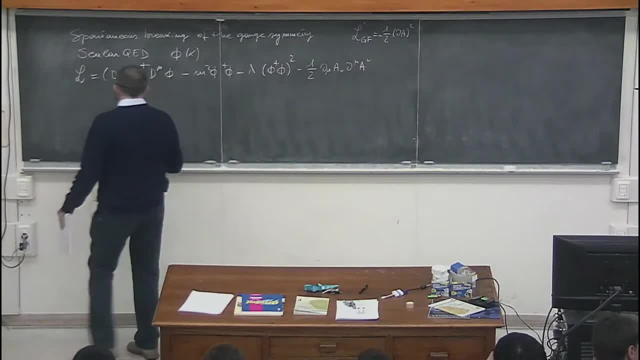 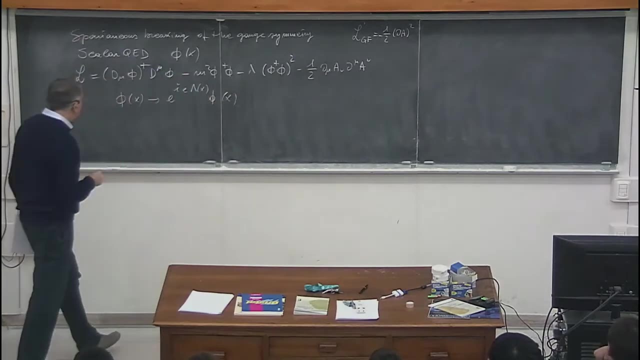 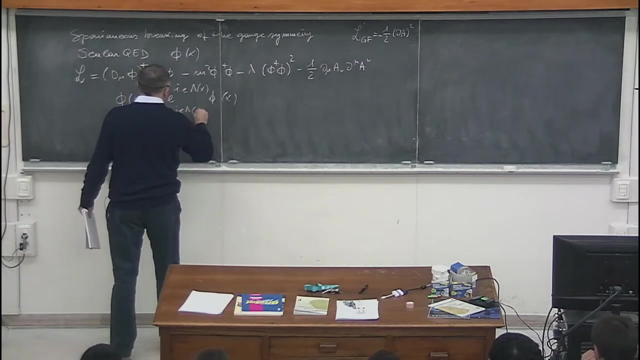 And this Lagrangian density is invariant under the transformation. phi of x goes to e to i e lambda of x. phi of x, where lambda is a real function, sp by dagger e to minus, i lambda. phi of x And a nu to a. mu plus d mu lambda is our usual gauge transformation. 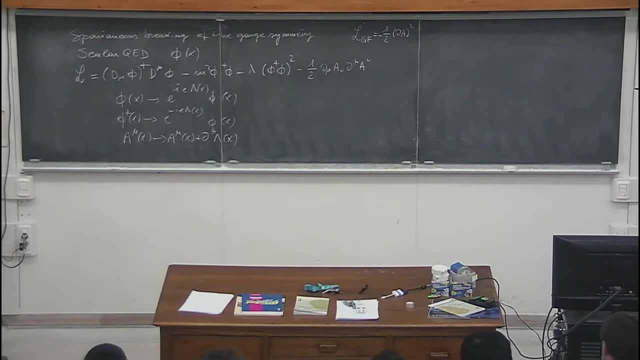 you are familiar with, since classical physics actually Provided the covariant derivative is less than or equal to sheep's height. the covariant derivative here is defined like this: d mu phi. equal ordinary derivatives minus Ie a mu phi. This is what is called scalar QED. There are 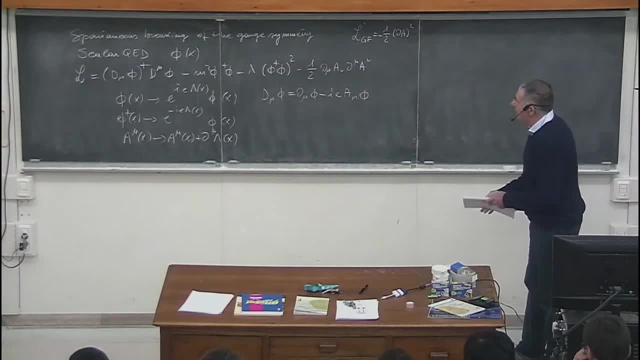 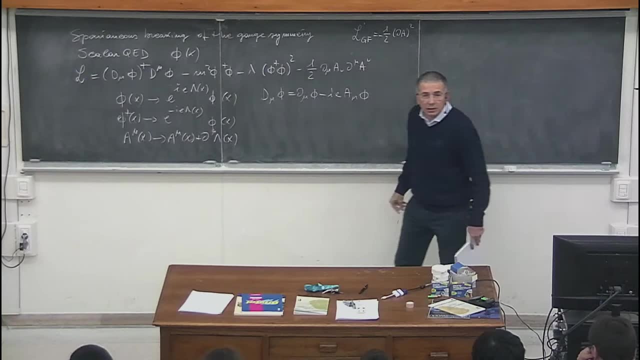 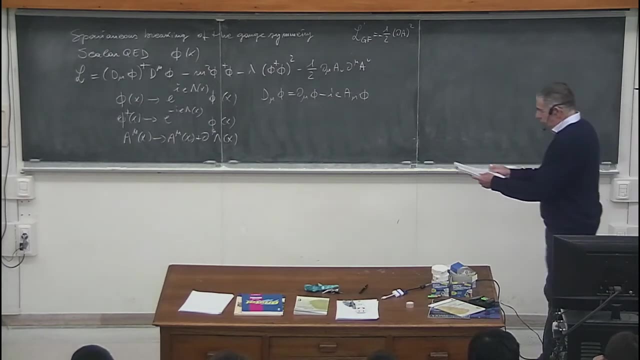 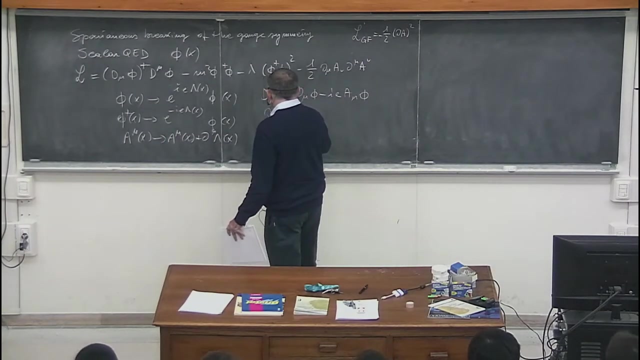 equations of motion for the fields phi. Actually, scalar QED is more complicated than usual QED because there is one more coupling constant, The coupling constant of the scalar field itself. The equations of motion are something like d mu v square plus m square phi. 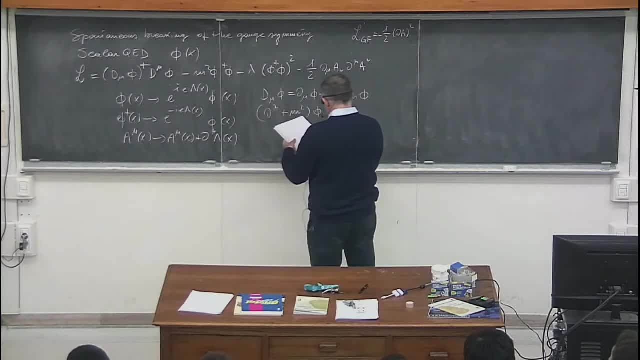 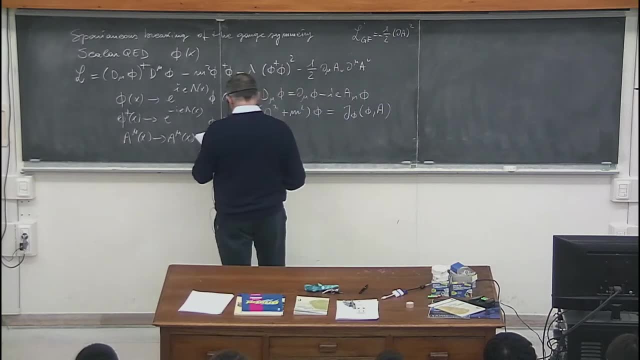 equal to five, which I call jphi. jphi is a fundamental därum, so this is like linear Rib-L included in the circular ant conducive. Add gegen Đ function of Phi and a and d square a mu. this is the miracle of the final gauge. 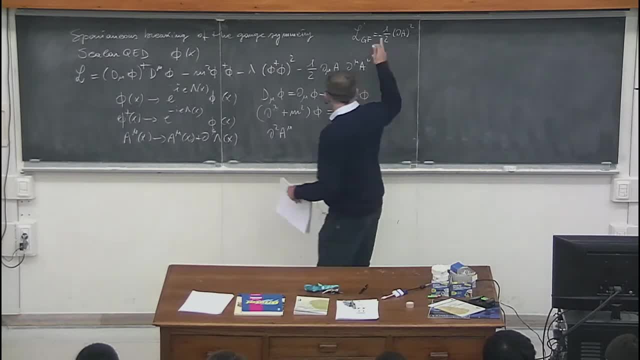 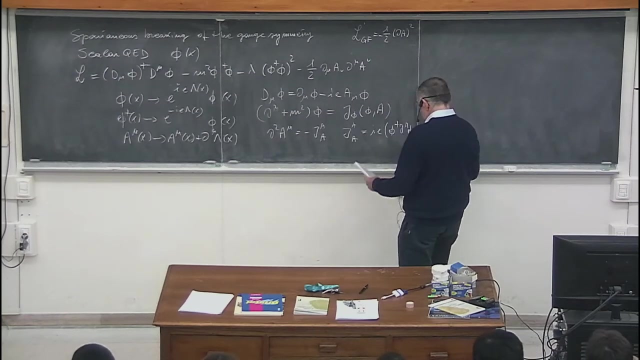 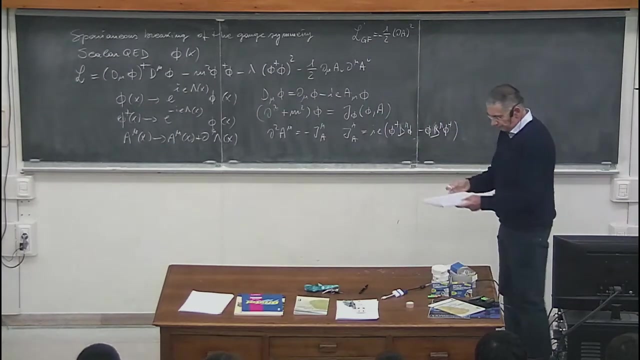 that is, there would be another term here which disappears with this gauge. fixing this square is equal to minus J mu a, and J mu a is the usual current for scalar charge. scalar field: i e phi dagger mu Phi minus Phi phi dagger d mu. covariant derivative. the gauge symmetry you are used to is said in this case to be: 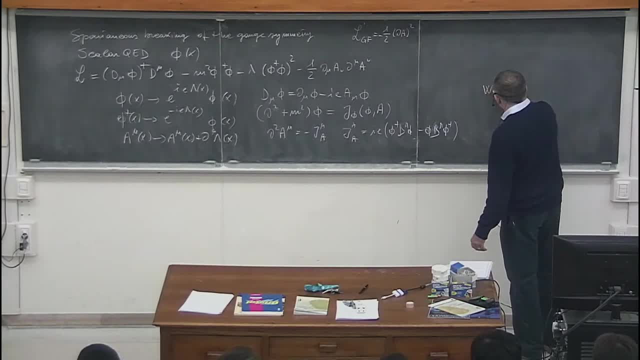 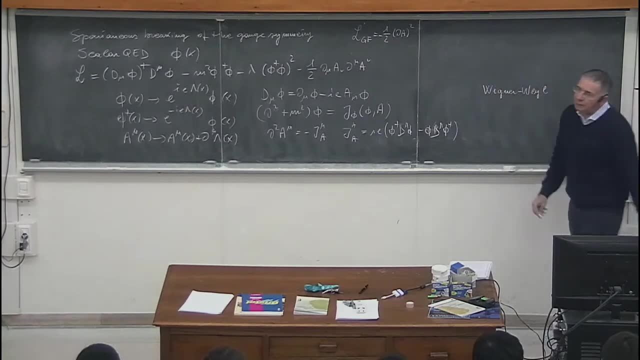 realized in the way way of Wigner vials. this is a Wigner vial realization of the gauge symmetry and the fact, the important fact, is that the zero field configuration is mapped into itself. the field configuration we correspond to Phi, equal to zero, everywhere and at any time. 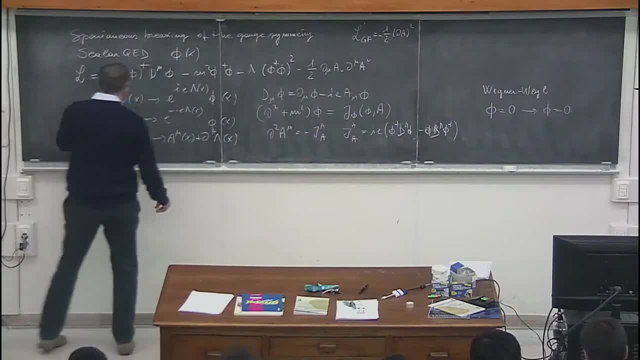 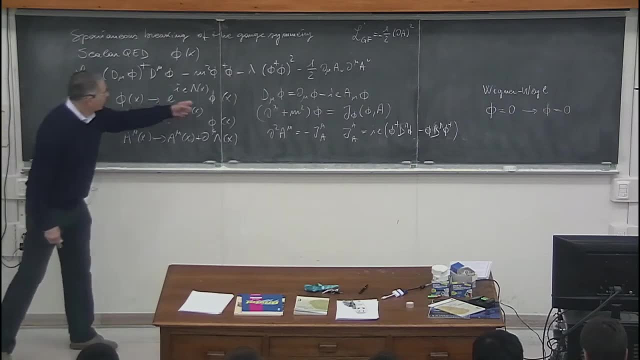 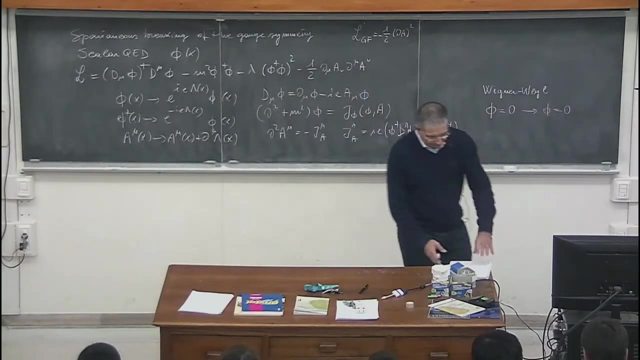 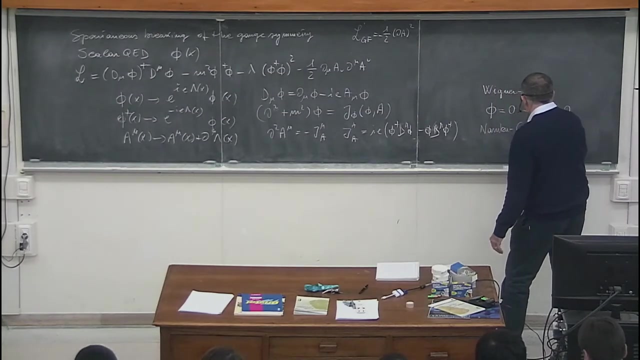 is mapped, is transformed into the same configuration, Phi equal to zero by the gauge transformation is homogeneous in Phi. so Phi equal to zero goes to Phi equal to zero. there is a different way to realize the gauge transformation in this case and the different called the Nambu Goldstone way. the Nambu Goldstone realization of the gauge. 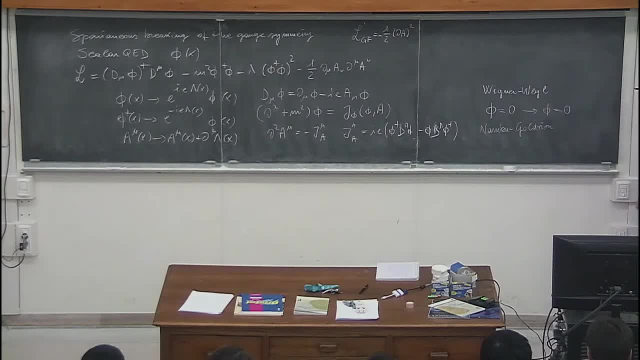 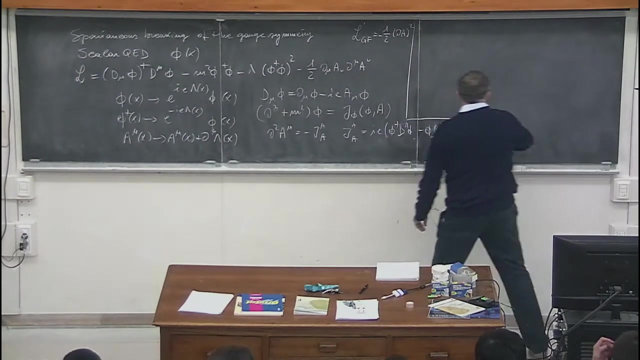 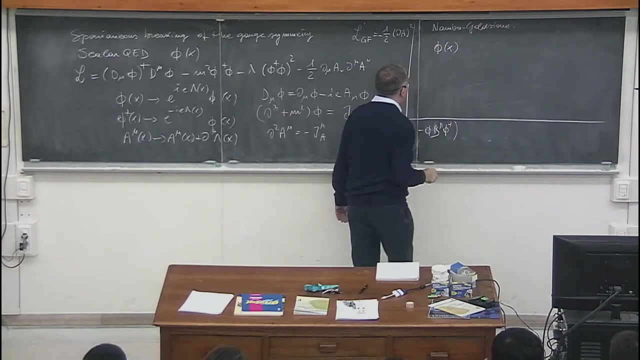 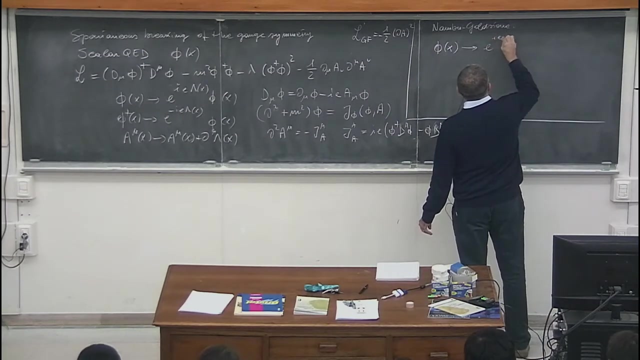 symmetry which doesn't share this property And the Nambu Goldstone realization of the gauge. symmetry is defined as follows: I define the transformed scalar field, phi, like this: e to i, e lambda of x times phi plus a constant which I call v, divided by a root of 2.. 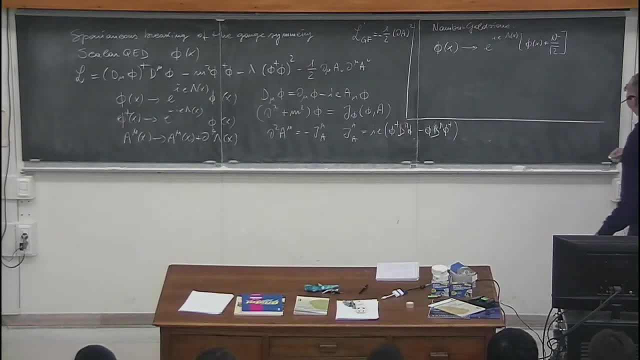 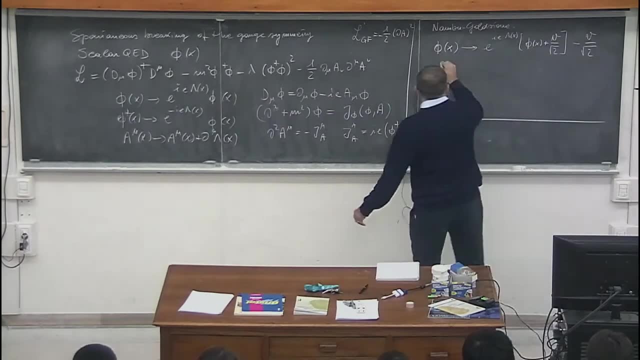 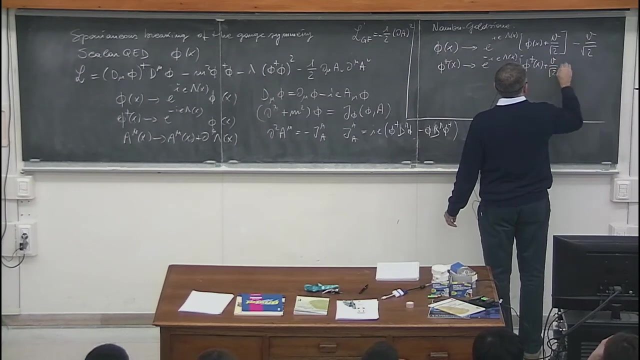 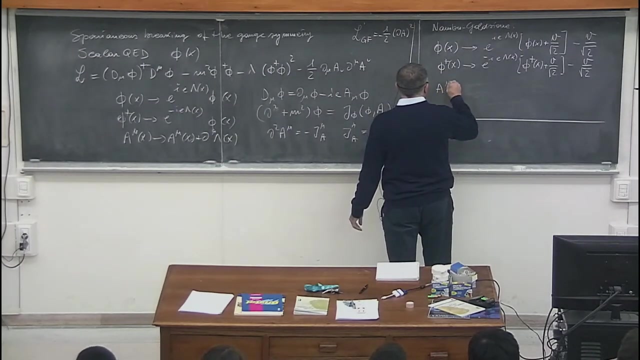 minus v over root of 2.. Of course, phi dagger goes to e. This is a real constant And the transformation of the vector field is unchanged. I will show you in a moment that it is possible to write down a Lagrangian which is invariant. 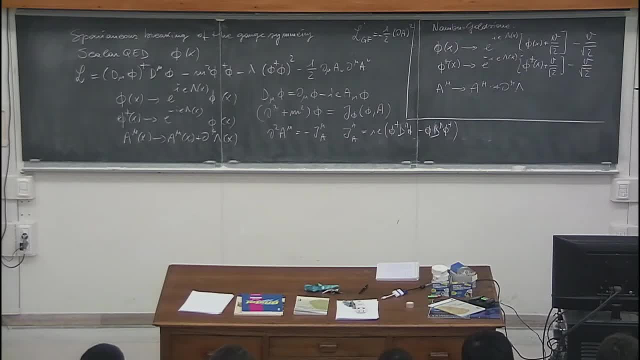 under this set of transformations. Let me just observe that, first of all, these kind of transformations do not leave phi equal to zero equal to phi. do not map phi equal to zero into phi equal to zero. If I said here zero, you get something different from zero in general. 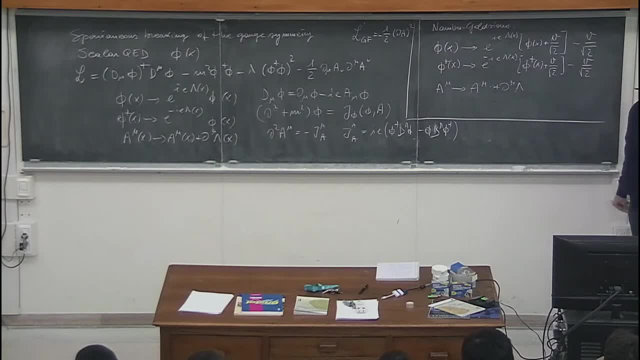 And the second important observation is that v, the real constant, v, is now a new fundamental constant in our Lagrangian density. So such a transformation is only possible, it is only possible to define Nambu Goldstone transformation for a scalar field, because phi, because v has the same transformation. 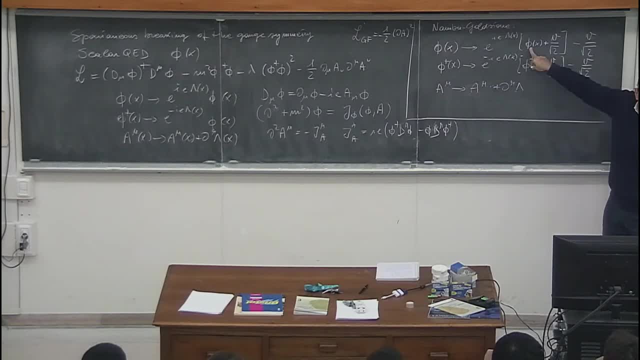 properties as the field phi under Lorentz transformation. So in other words, phi has the same transformation properties as the field phi under Lorentz transformation. So we don't want constants that transform upon Lorentz transformations. So this is only possible with scalar fields. 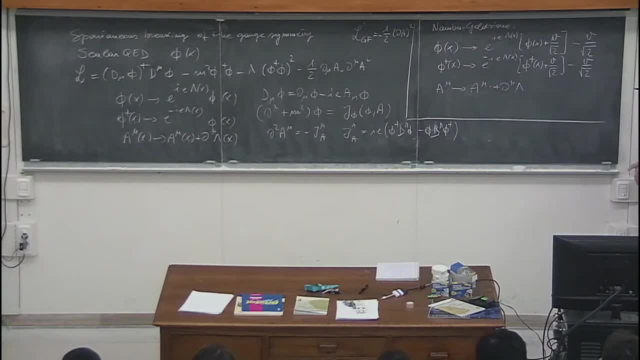 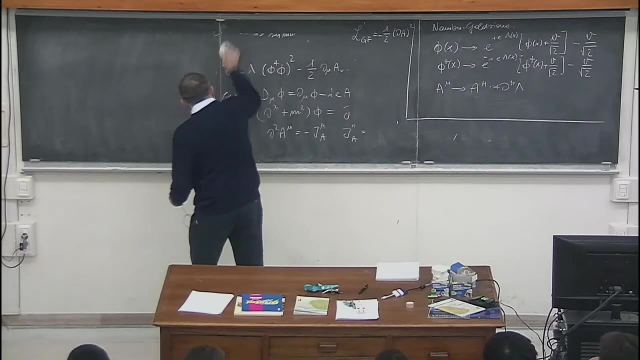 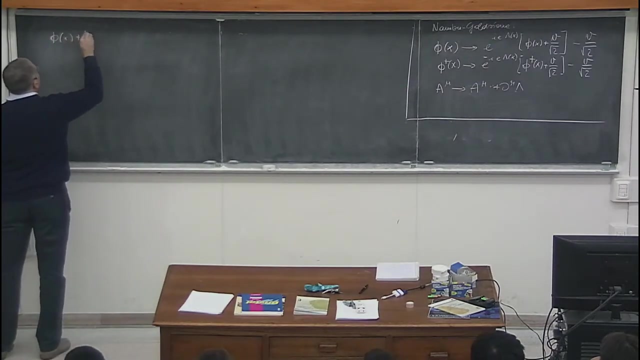 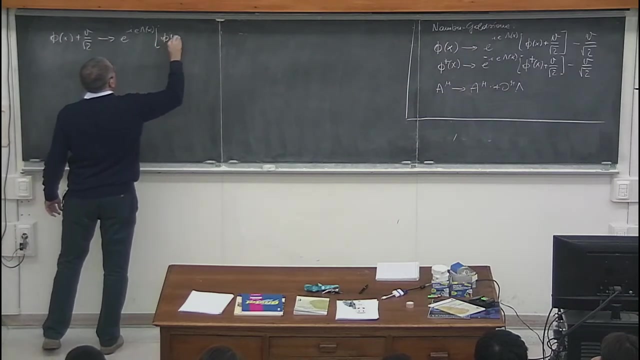 Okay, how do I build an invariant Lagrangian? And if I assume that the gauge transformations are like this, it is quite easy. It is especially easy if I rewrite the transformation law for phi of x in this way, If I write it like this: 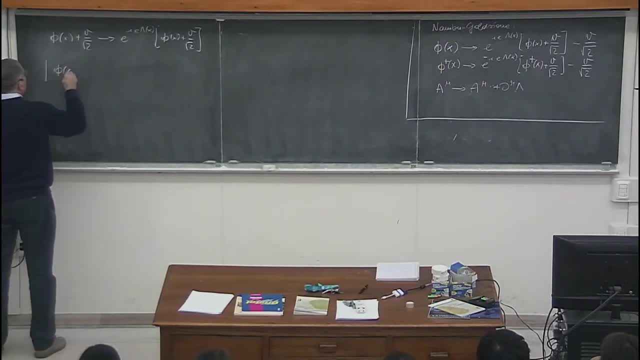 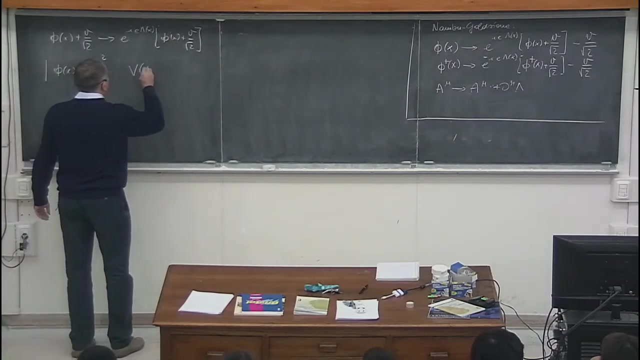 It is obvious that Phi, Phi Plus v over root of two module square is invariant upon this kind of transformation. This transforms by multiplication by a phase and a phase is square, mod is one. So this is invariant. So the scalar potential which I can build, with the constraints that it is invariant upon this, 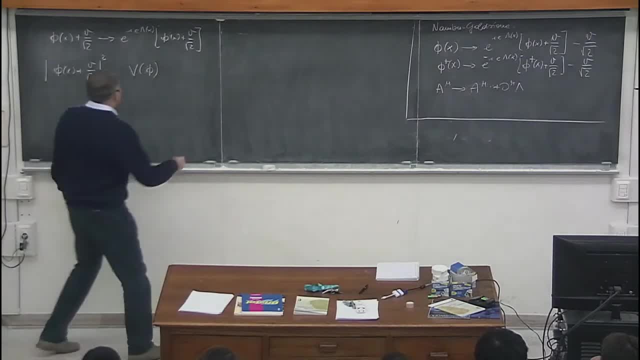 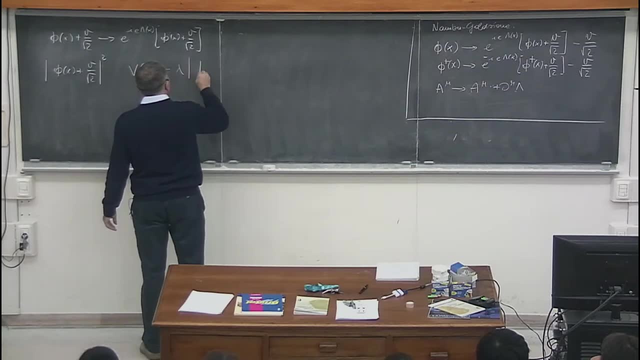 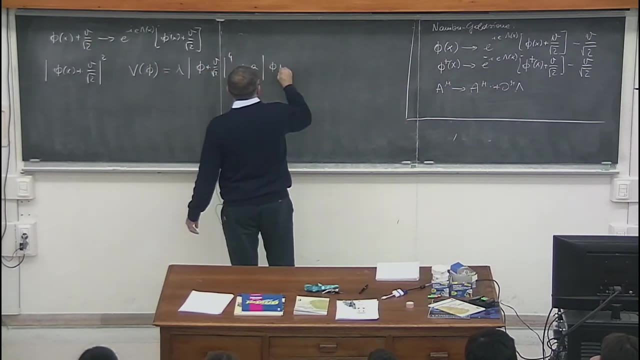 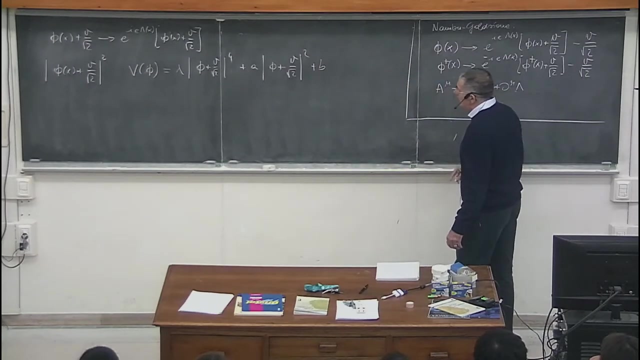 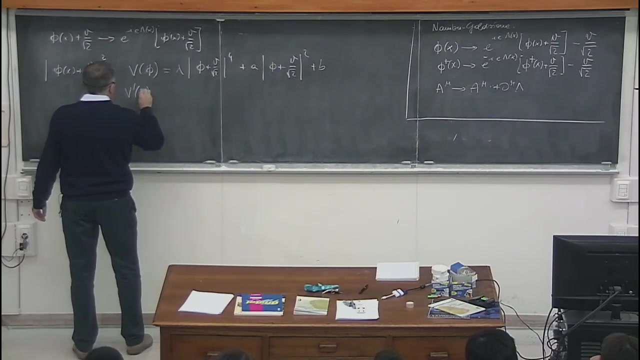 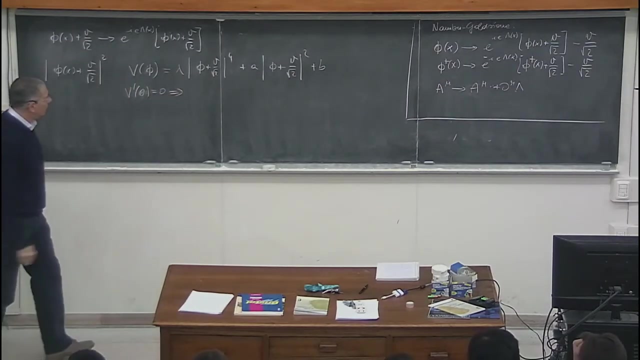 kind of transformation, and it is renormalizable- turns out to be a quadratic function of this quantity. so I can write it like this: And b is irrelevant, of course. and if I further require that the potential has a minimum when phi equal to zero, then you can work out a little bit and discover that the potential 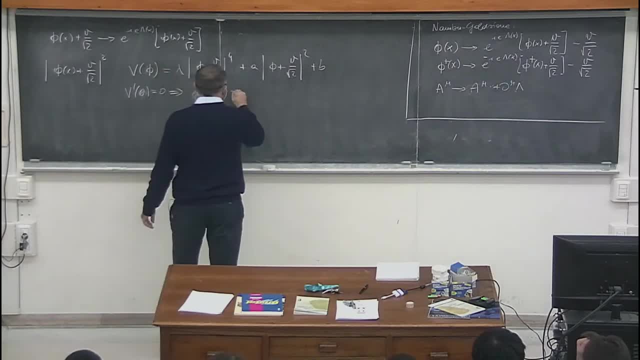 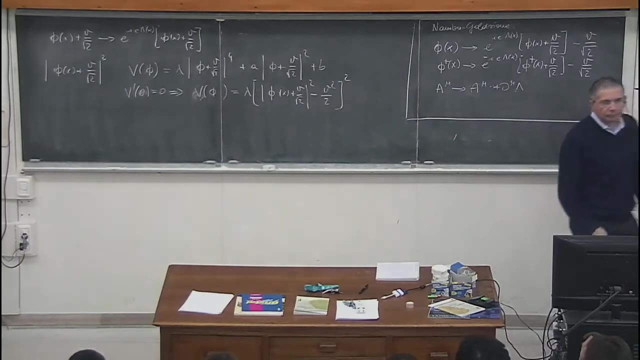 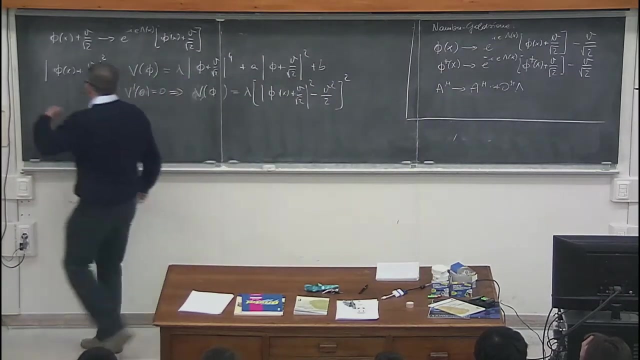 has a unique form up to an additive constant which is lambda phi of x plus b Plus v over root of two square minus v square over two to the second power. This scalar potential is uniquely determined by these two requirements: the requirement of renormalization. the three requirements gauge invariance with respect to the Nambu-Golston. 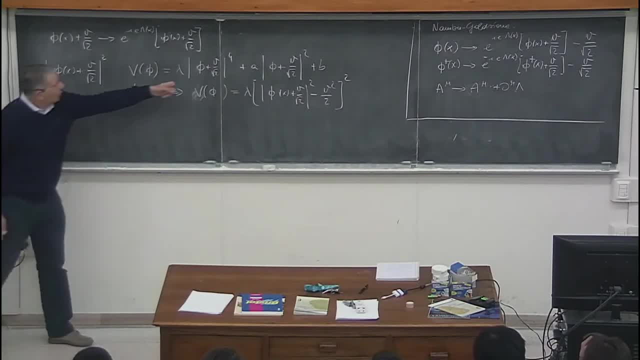 transformations no more than four powers of the field And n minimum at the origin. So this is the scalar potential. I need a covariant derivative and the covariant derivative is easy to work out. I define d mu of phi plus v over root of two as d mu phi plus v over root of two. 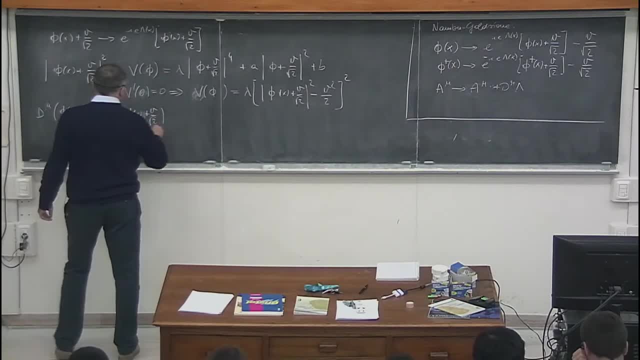 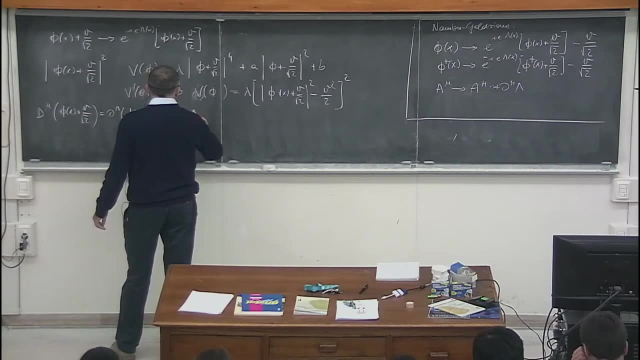 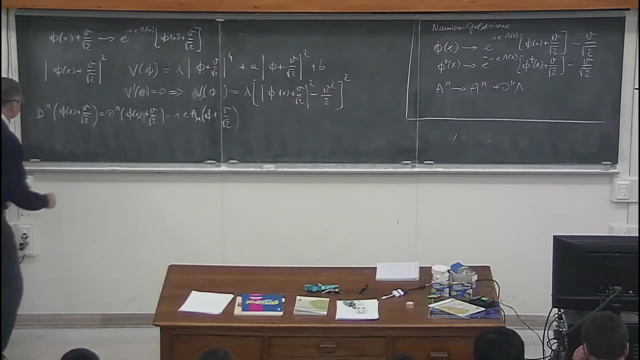 This is irrelevant because the derivative acting on a constant gives zero minus. i cubed E A mu phi plus V over root of 2.. This is again covariant in the sense that D? mu phi plus V over root of 2 transforms as: 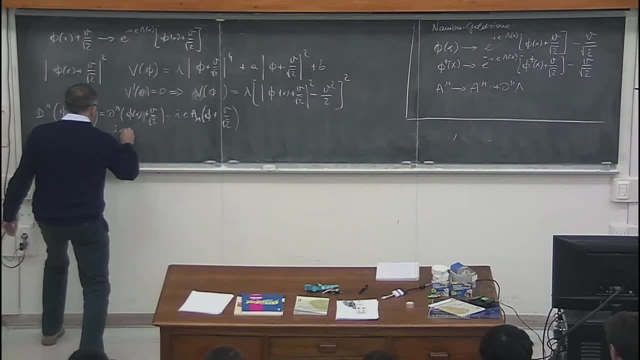 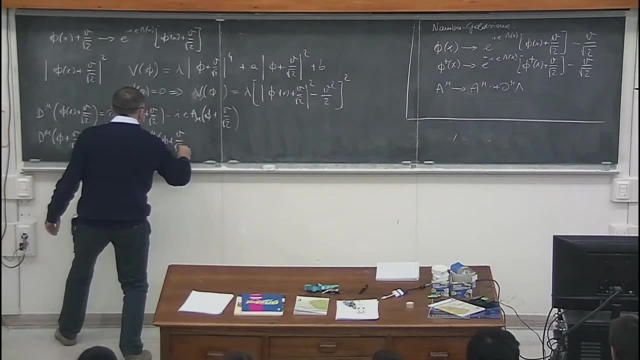 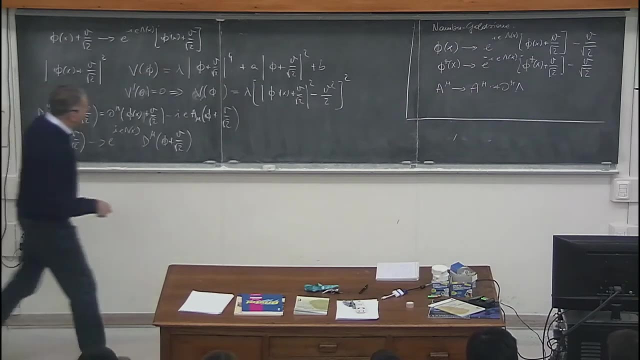 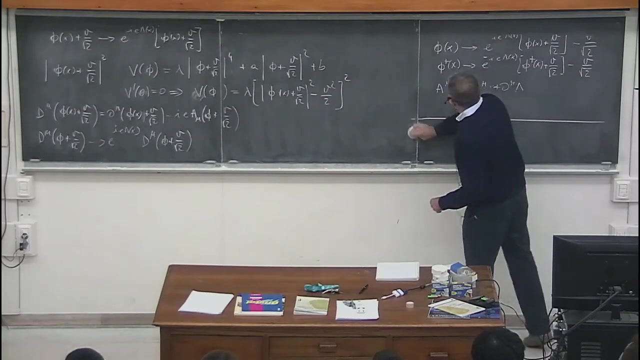 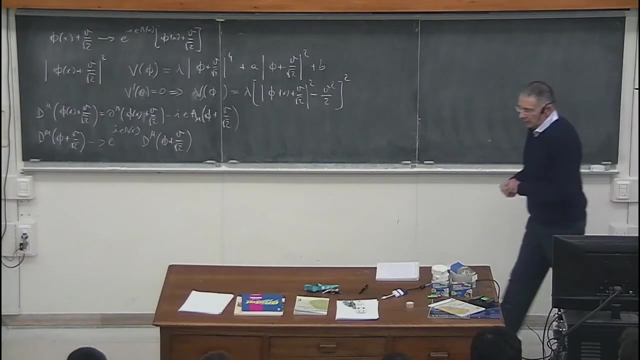 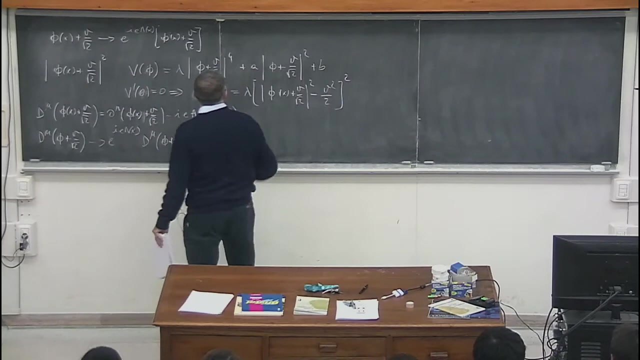 the field. This is easy to check. So scalar QED with the Nambu-Golston realization of the gauge symmetry is here. I can erase immediately written: Oh, gauge fixing. The gauge fixing term here is: it is convenient to choose a slightly different gauge fixing term which is 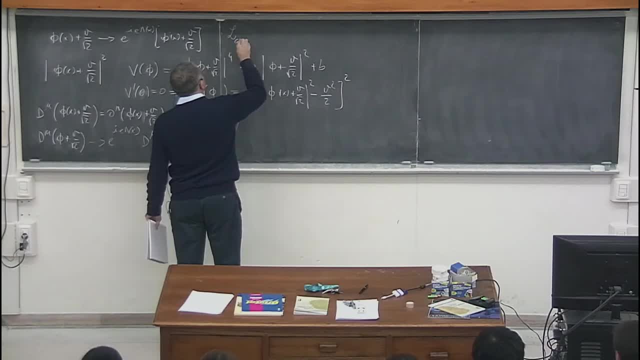 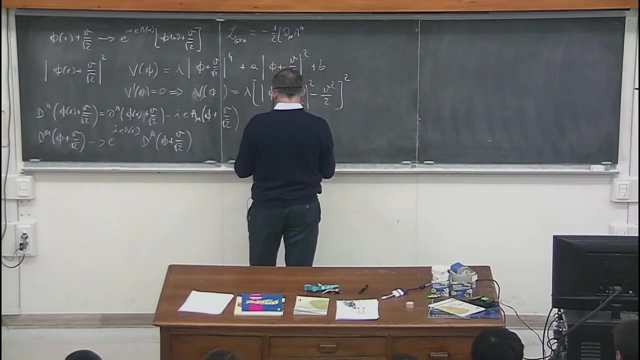 called the Feynman-Toft gauge fixing, And the Feynman-Toft gauge fixing is like this: It's minus one half. Instead of D mu A mu square, I have D mu A mu plus something, and something is proportional to the imaginary part of phi. 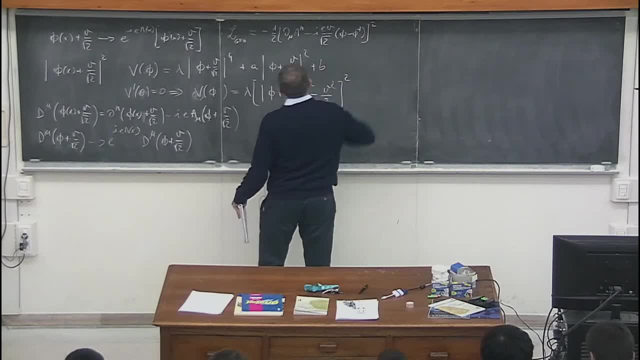 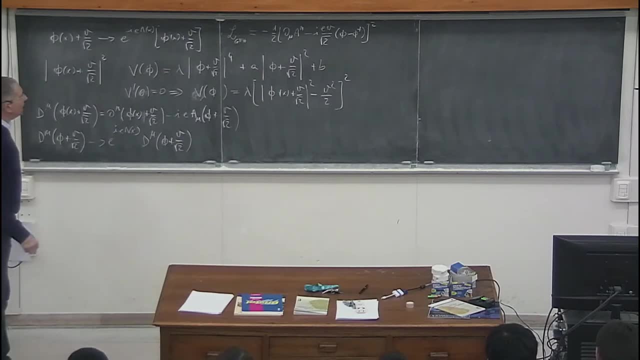 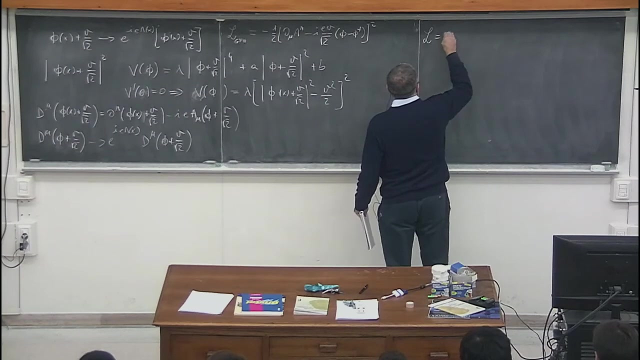 And this term is just the general type of system I have leave. in this case The gauge fixing is arbitrary, so I can choose whatever I like And we will see in a moment why this gauge fixing term is more convenient in this case. So Lagrangian density is: 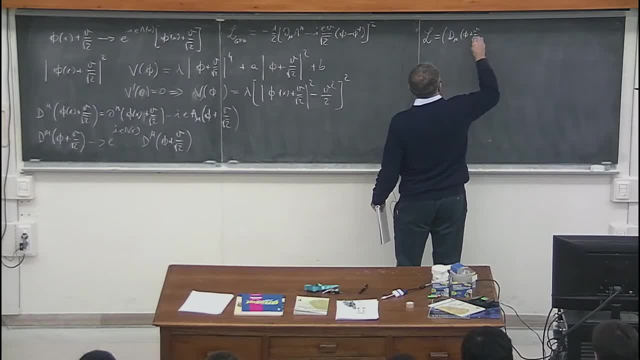 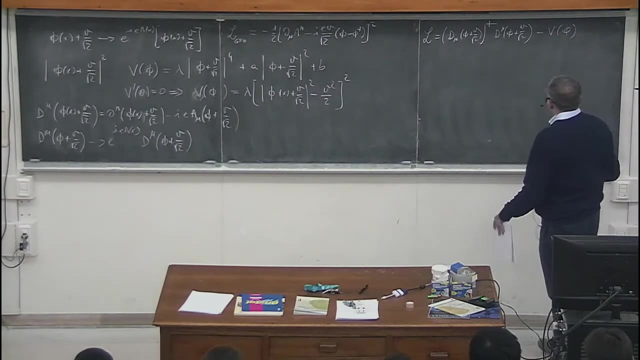 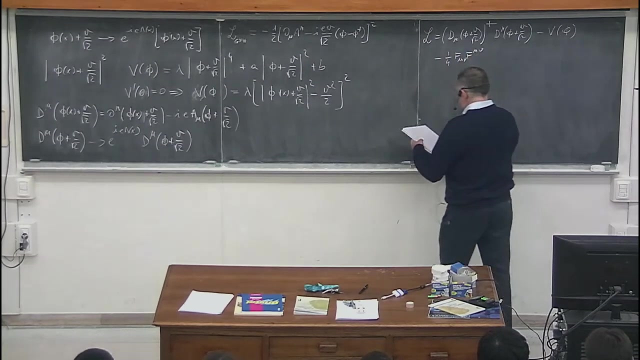 D mu phi plus V over root of 2 plus Einspannpryred power: 0.6 O8·Bv. root of two. Hermitian conjugate: d mu phi plus v over root of two, minus the scalar potential which is written down there explicitly, minus one-fourth f mu nu, f mu nu plus gauge. 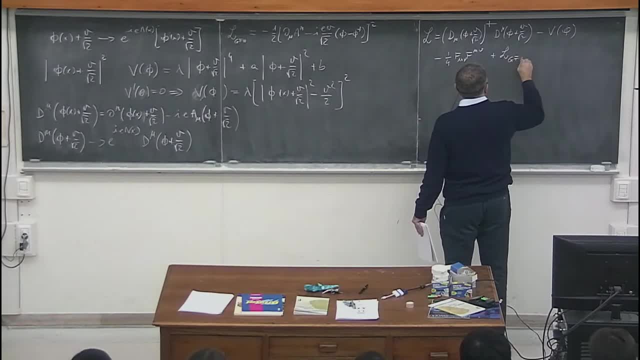 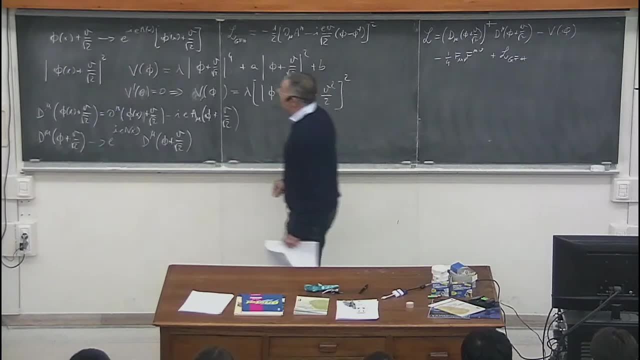 fixing term. This is scalar QED with this definition of the transformation of phi under the gauge group. Why do I like it so much? Well, first of all, let me observe that the Lagrangian is still renormalizable. It is non-negative. 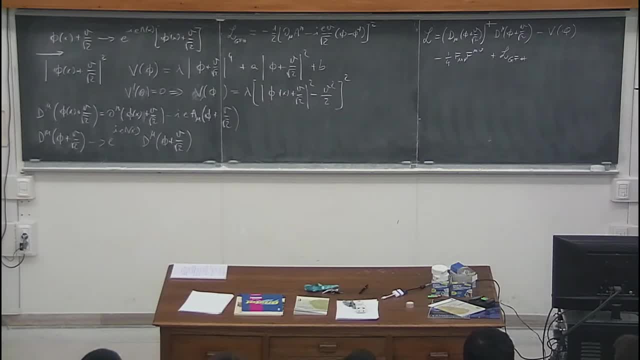 It still gives rise to a unitary S-matrix because the gauge symmetry is still there. I have just defined it in a slightly different way, but it is still a gauge symmetry. so nothing has changed. We haven't destroyed the good properties of ordinary scalar QED. 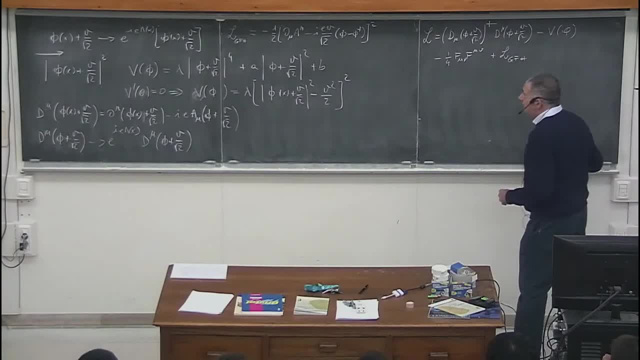 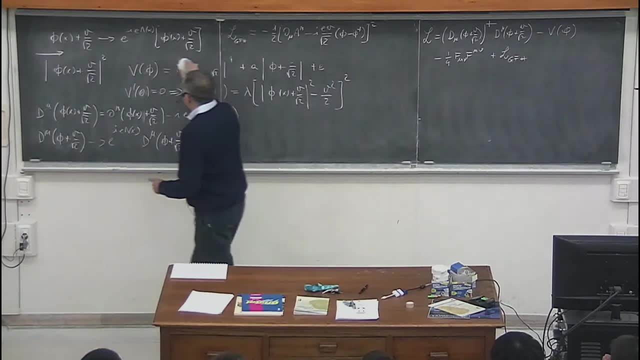 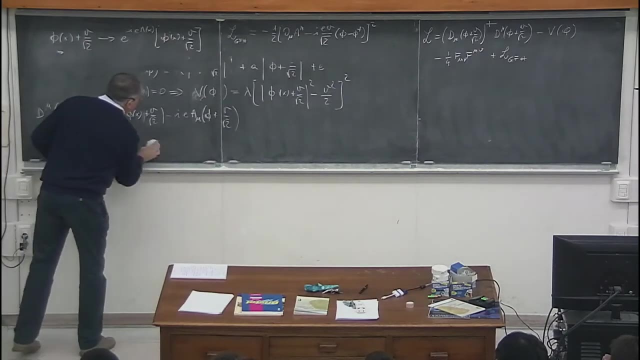 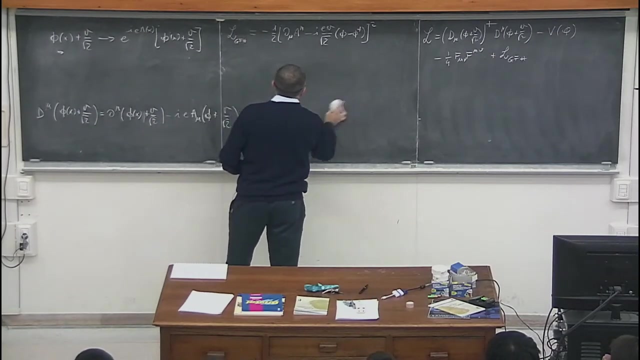 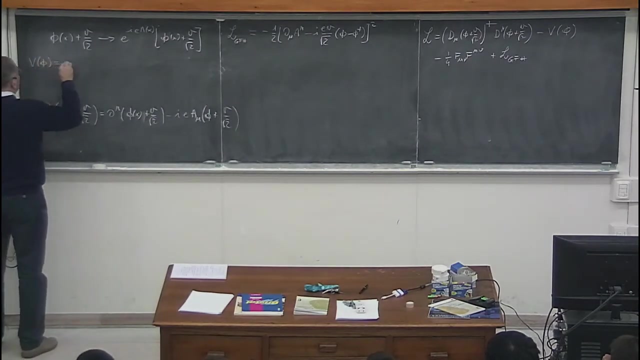 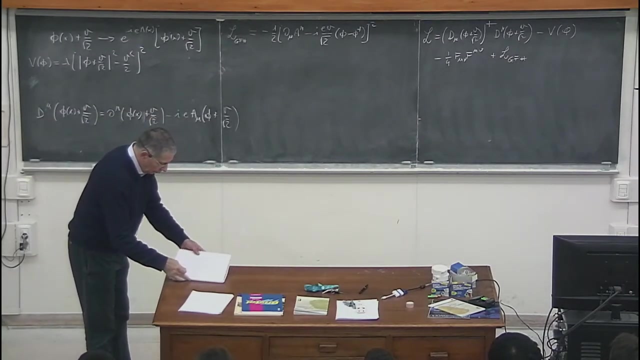 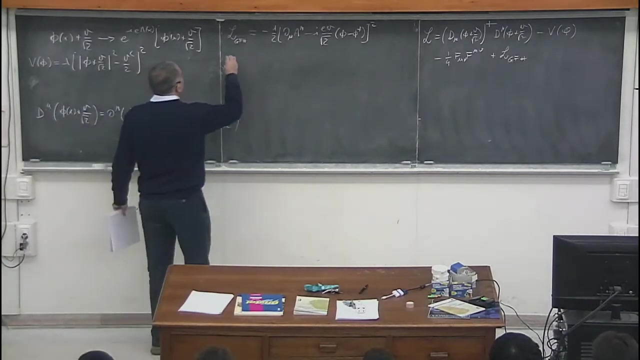 I need the scalar potential and I need the covariant derivative. So let me write the scalar potential here And the covariant derivative is written there. I write it here. so I have some. Let me first collect in a The number of the quadratic terms that are in the fields. 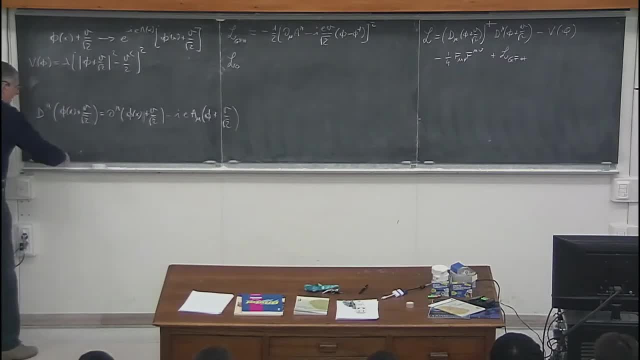 The quadratic part of the Lagrangian is important because it is the part which allows us to determine the shape of the propagators. It's the free propagating part. So what is L0?? L0 has quadratic terms which come from the scalar potential, from the square of the covariant. 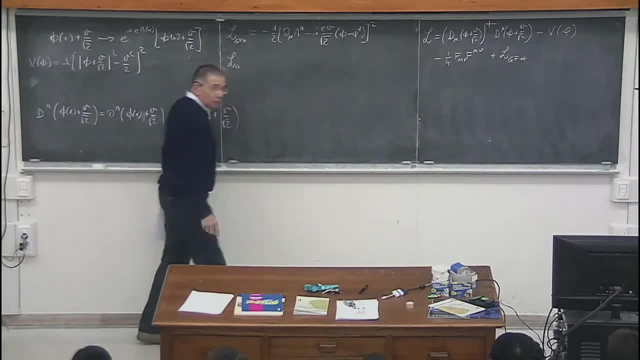 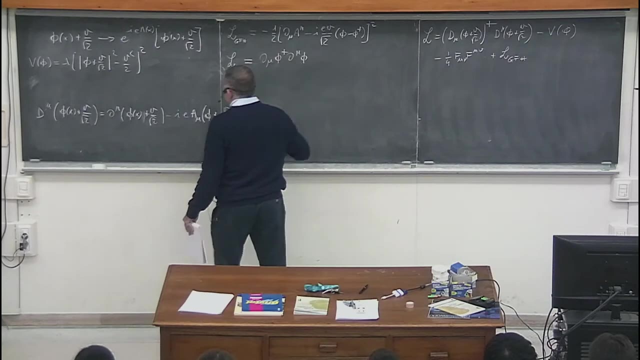 derivative, and also from the gauge fixing term, which is also quadratic in the fields. So I have to collect them all. this is just a matter of algebra. What do I get? I get a kinetic term for the complex scalar field. this comes from the ordinary derivative. 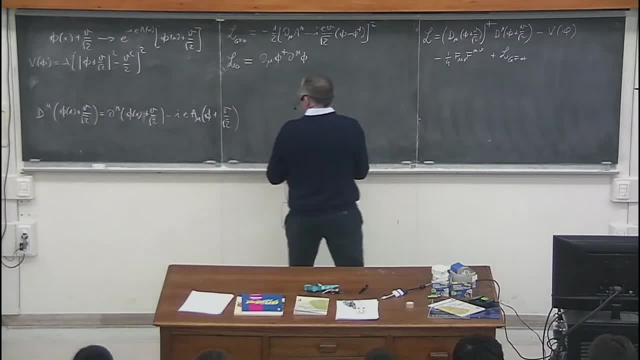 of the mu. Then I have a mixed an interference term between the derivative of the scalar field and the field, a mu, from the square covariant derivative term. and this is plus i e v over root of 2 a mu, d mu phi minus phi dagger. 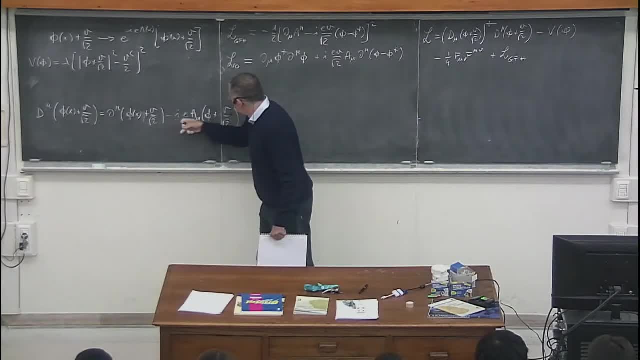 There is a phi minus phi dagger, because there is a minus i phi in the covariant derivative and a plus i phi dagger in the covariant derivative of the Hermitian conjugate. So what you get is this term here. Then there is a quadratic term from the square of this term here, a mu times v and this: 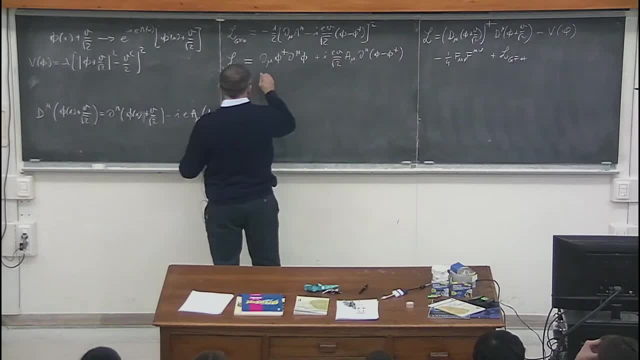 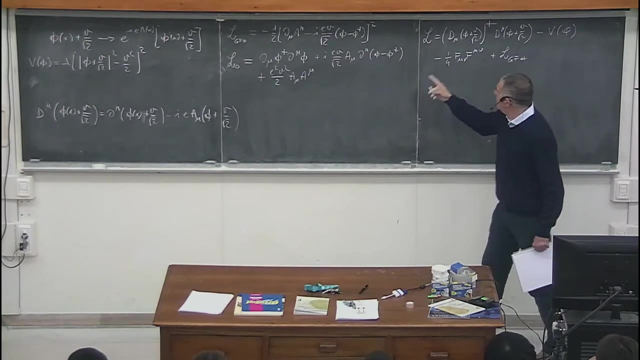 is- let me write it here- plus e square, v square divided by 2.. v over root of 2: a mu, a mu. The square of this term i e a mu. v over root of 2 is this term here, And this is a mass term for the vector boson. see a constant times: a mu, a mu. 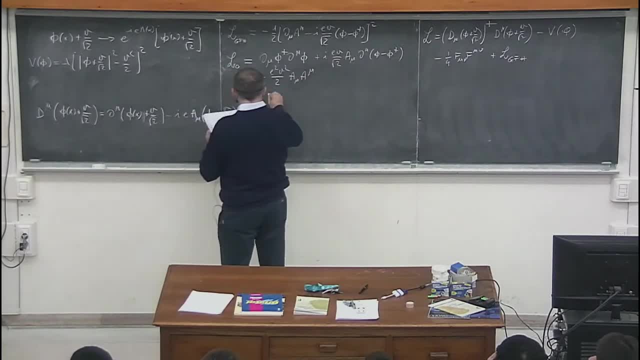 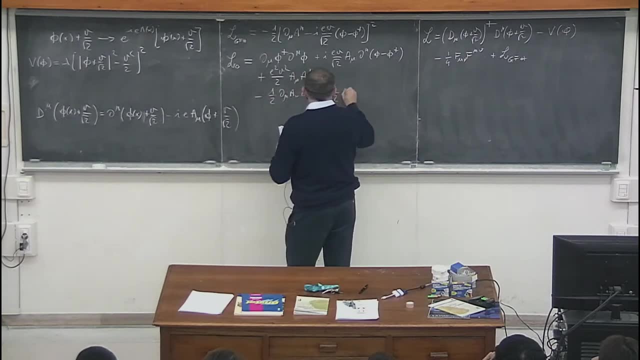 Then I have the derivatives of the vector field: one half d mu a mu, d mu a mu, minus one half d mu a mu. So I have a constant times a mu a mu, And there is another term proportional to the derivatives from the gauge fixing term. 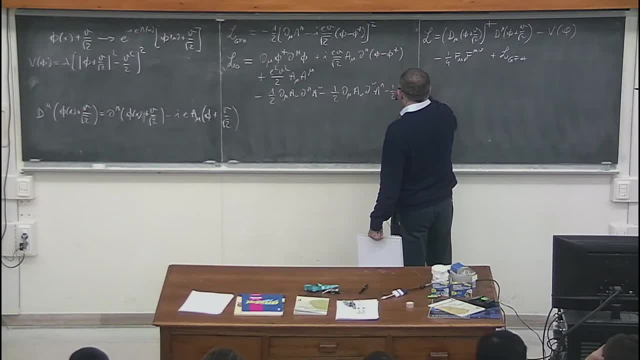 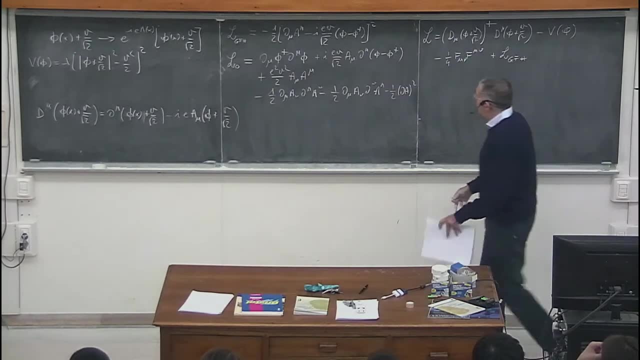 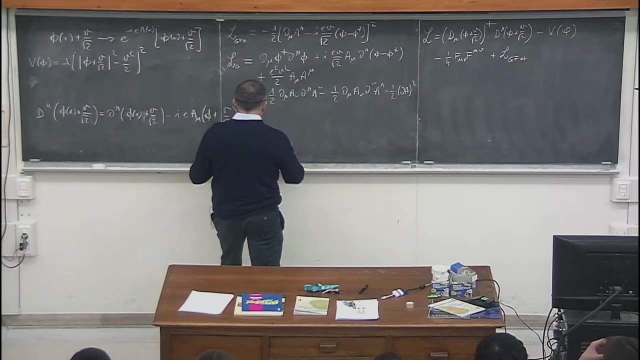 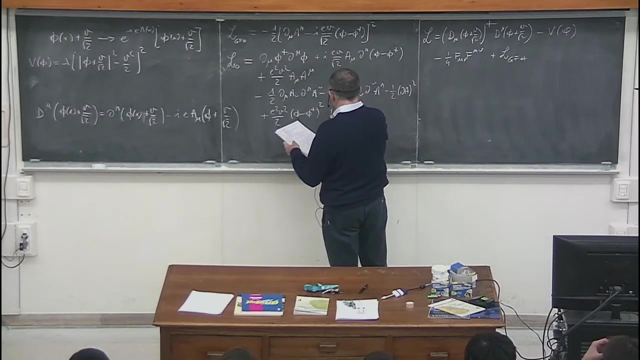 which is minus one half d a square. Then what do we have? We have a quadratic term here which is plus e square, v square divided by 2. phi minus phi dagger square. And finally, I have an interference term here which is plus i e v over root of 2 d mu a. 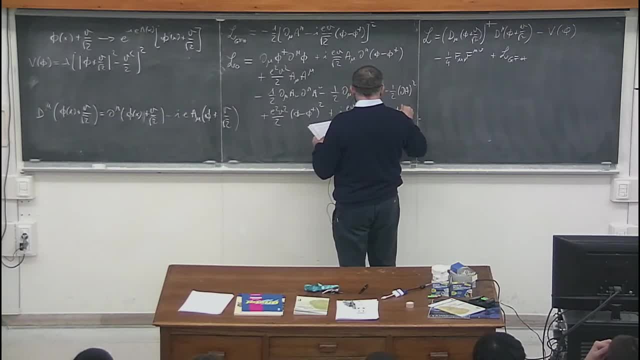 mu phi minus phi dagger. Very complicated, but I simply put it here. So what you get is this: This is the derivative of this term here. So what you get is this. So what you get is this: And this is the derivative of this term here. 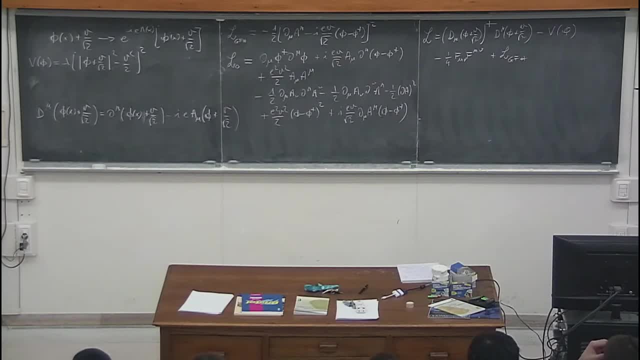 So let me verify it in a moment. So what happens here? The first interesting thing is that the sum of these 2 terms- the second term in f mu mu, f mu mu and the part of the gauge fixing term which depends only on the vector field, 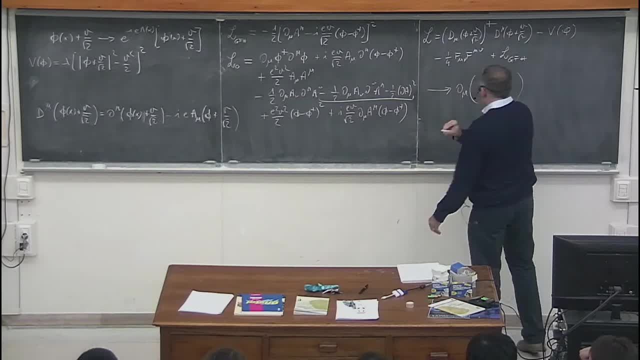 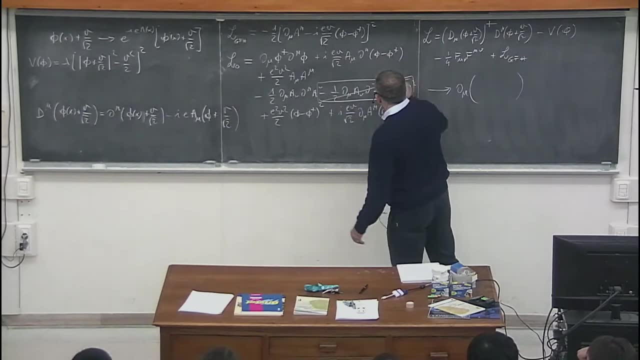 this is a total derivative. It's d mu of something. You can prove it very easily, So I can drop it altogether. So Total derivative has no effect on the equations of motion, on the stationarity of the action, so I can just forget about it. 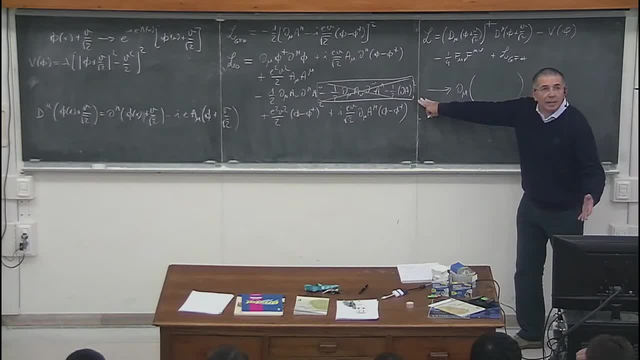 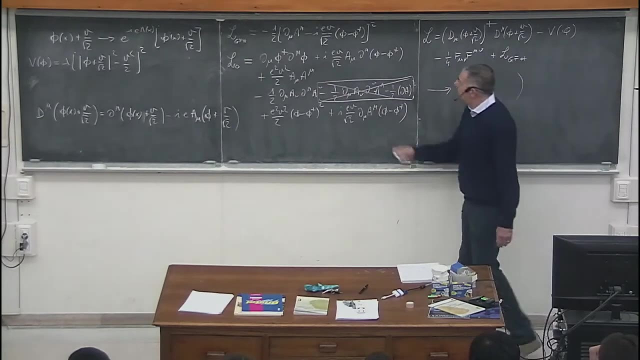 And this is exactly the same as in the case of the final gauge for standard QED, for ordinarily realized QED. Then look at these two terms. These two terms are particularly unpleasant because they are quadratic in the fields but they mix the vector field with the divergence of the scalar field. 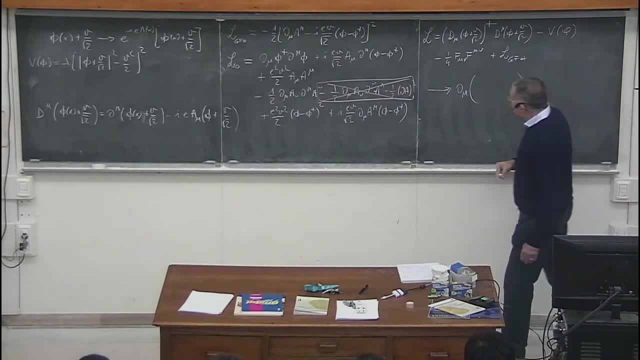 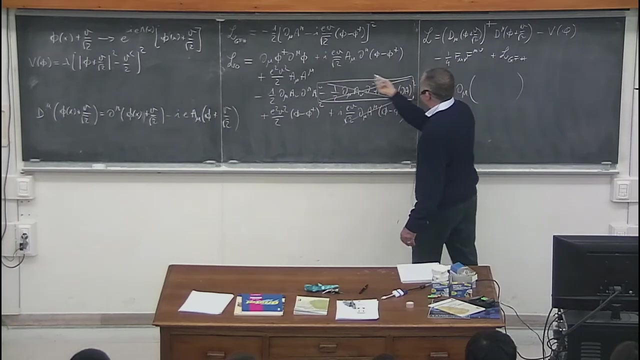 But if I perform a partial integration, for example in this term, and I assume that the fields vanish at infinity rapidly, then you have a minus sign here and the derivative is acting on phi minus dagger and these two terms cancel exactly. So I cancel this against this, and this explains why it is convenient to use this Toft gauge fixing term. 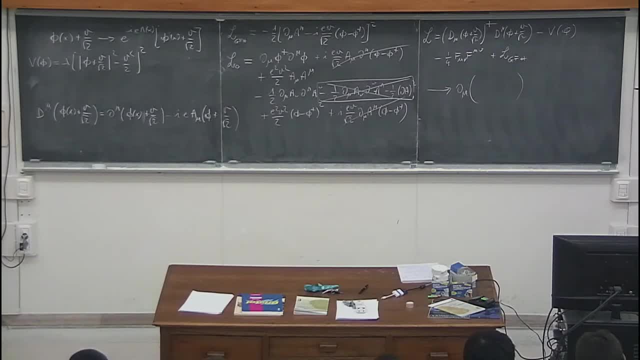 The Toft gauge fixing eliminates the mixing between a mu and the divergence of the imaginary part of phi. Oh, they cancel because they are exactly the same, except that here the derivative acts on a mu and here the derivative acts on phi minus. 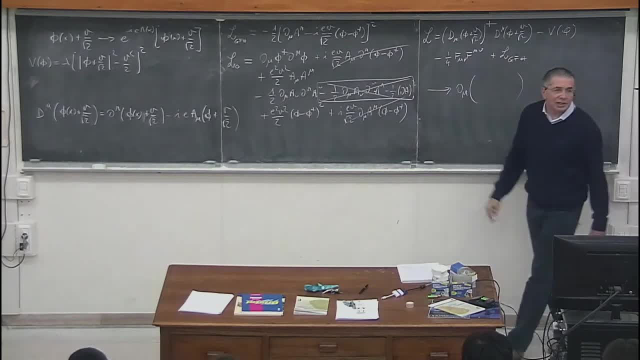 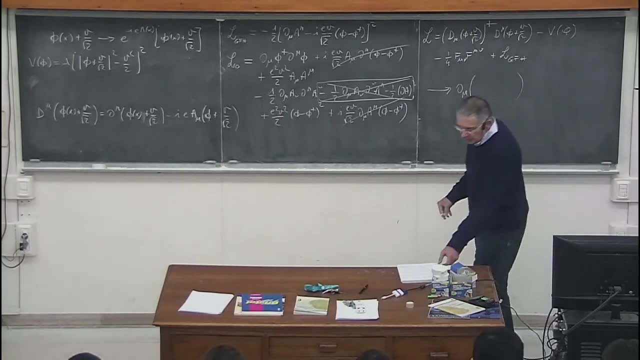 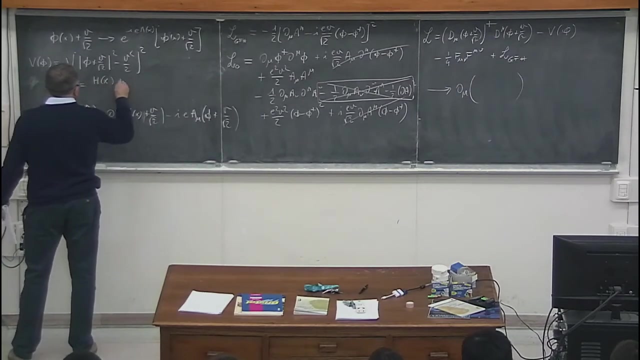 So I integrate by parts and the derivative is the same sign change and they cancel against each other. So this simplifies considerably and it is convenient to write phi in terms of a real part and an imaginary part, which I call respectively h of x and g of x. 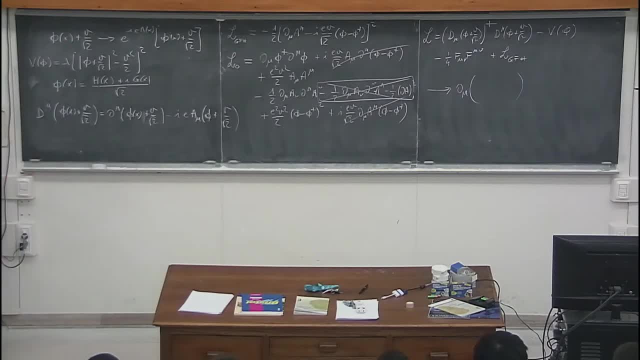 h stands for Higgs and g stands for Goldson, and this should remind you of something you already saw. So if I do that, this L0 becomes simply 1 half times d mu h, d mu h plus d mu g, d mu g, and this is this term. 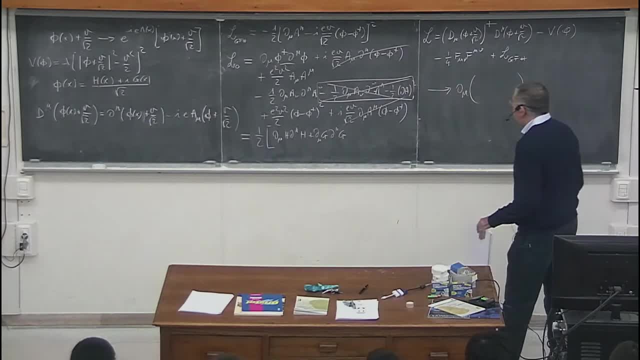 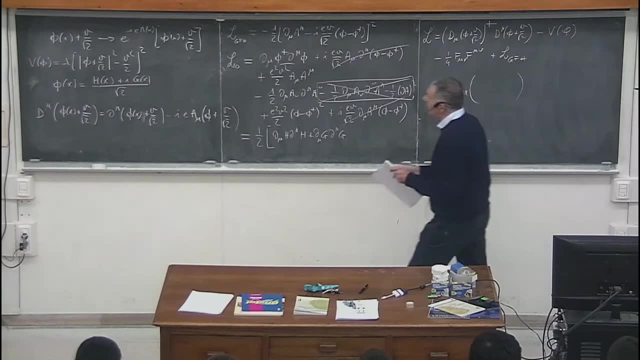 Then I have a quadratic term for. Sorry, I forgot to write down the quadratic term in the real part. There is a quadratic term for the real part from the scalar potential, which is: Where is it? My, my, minus, lambda, divided by 2, v squared phi plus phi, dagger squared. 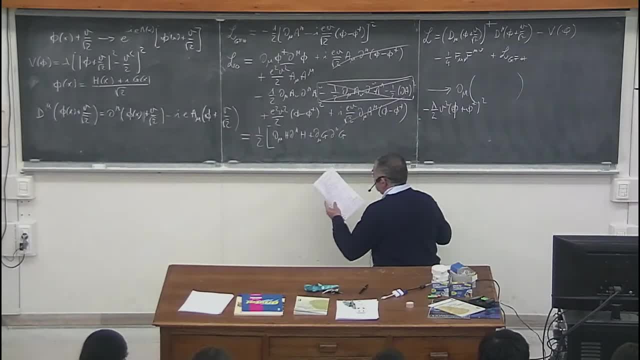 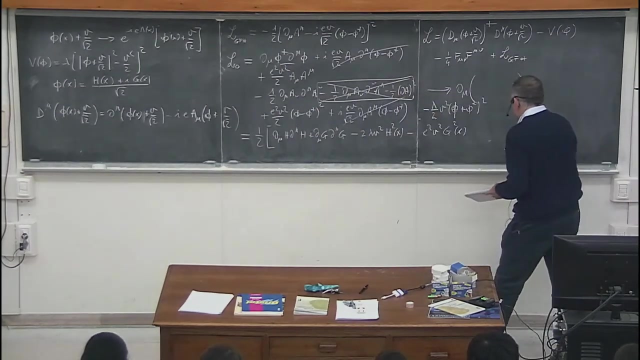 So there are kinetic terms for the two scalar fields. Then I have mass terms minus 2 lambda v squared. h of x squared. minus e squared v squared minus g of x squared. Then I have the derivative term for the vector field. 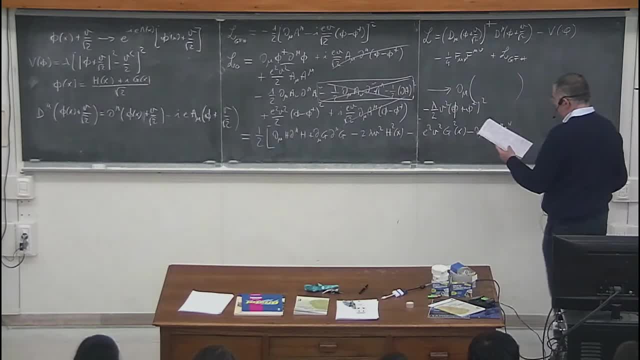 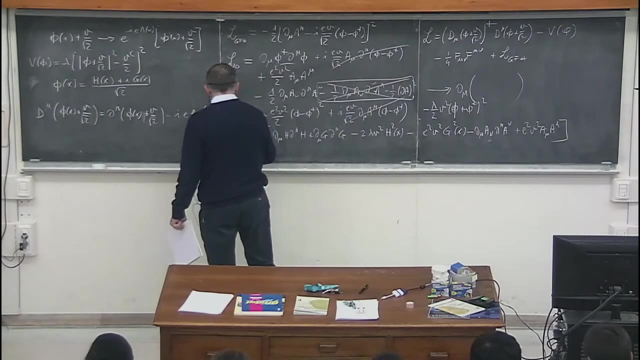 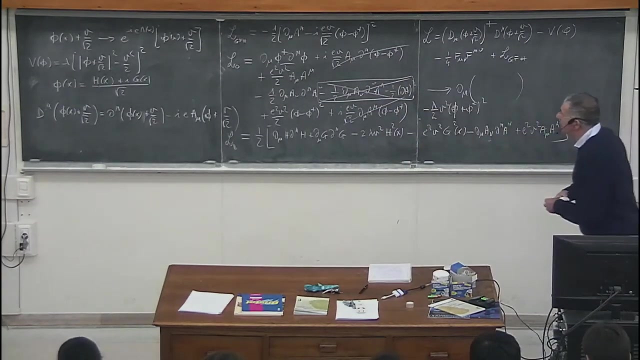 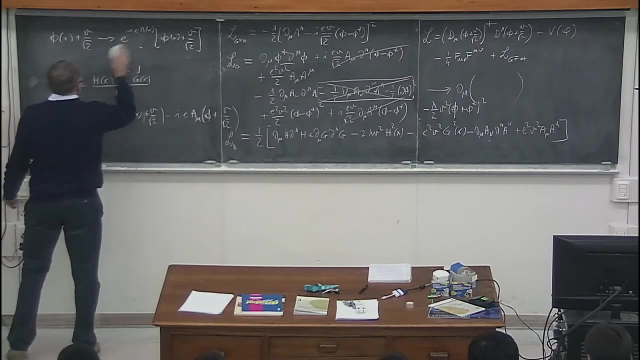 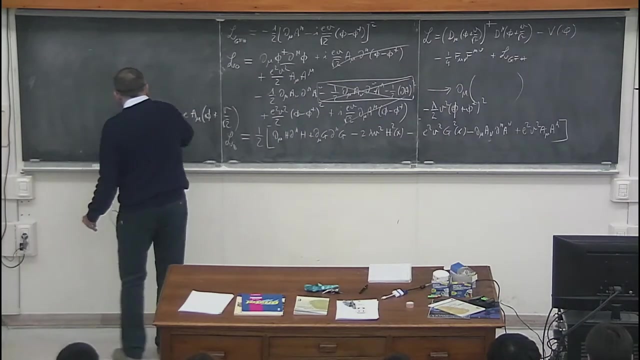 d mu a nu, d mu a nu. plus e, squared v, squared a mu a mu. This is L0.. I did nothing. I just defined the gauge transformation in a different way. So what are the propagators for this theory of quantization? 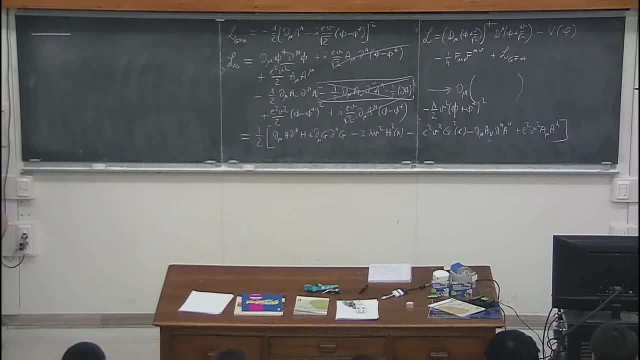 There is a. I use solid lines for the field. for the Higgs field, the real part of the scalar field and the corresponding propagator is minus 1 over k squared, minus 2 lambda v squared plus i epsilon. So the mass, the squared mass of the Higgs boson is related. 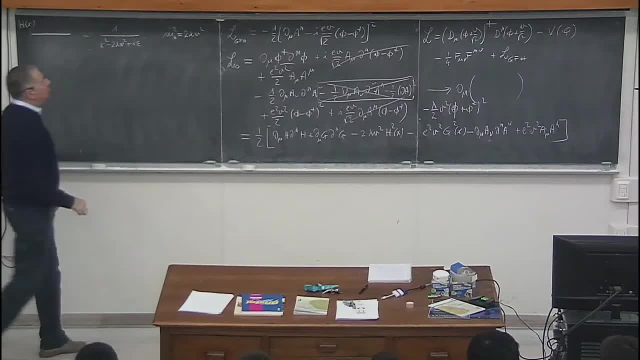 to the parameter which enters the definition of the field transformation, which of course has the dimension of a mass, because it has got the same dimension of the field, phi. Then let me use a dashed line for the Golston field. The Golston field is a scalar, real scalar, massive field. 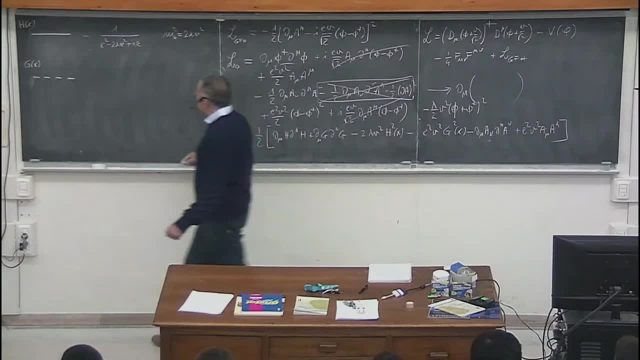 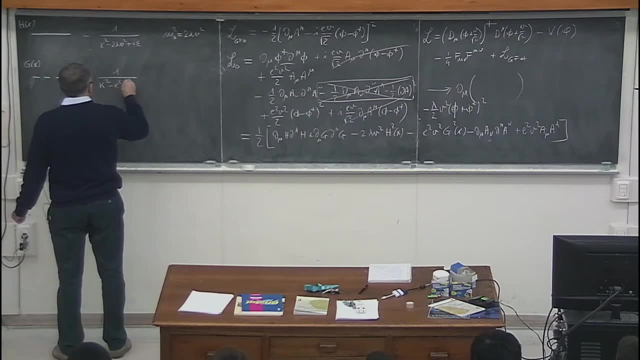 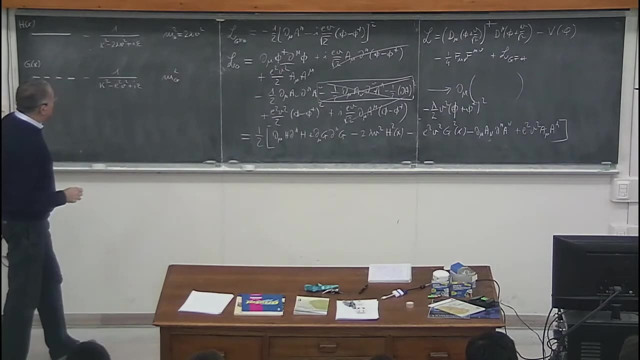 with mass e squared v squared, So the corresponding propagator is minus 1, over k squared minus e squared v squared plus i epsilon, which means that with this gauge fixing the mass of the Golston boson is e squared v squared. 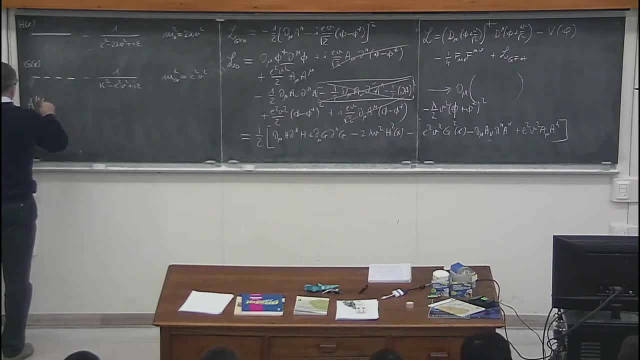 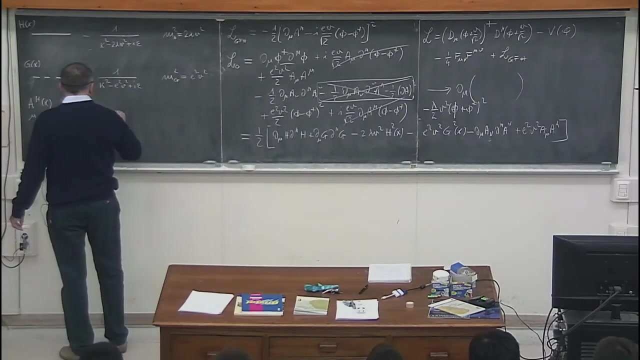 And then I have a vector for which I use, as usual, a wavy line which has Lorentz indices at the vertices, And the propagator for the vector boson is g, mu, nu, divided by k squared minus e squared plus i epsilon. 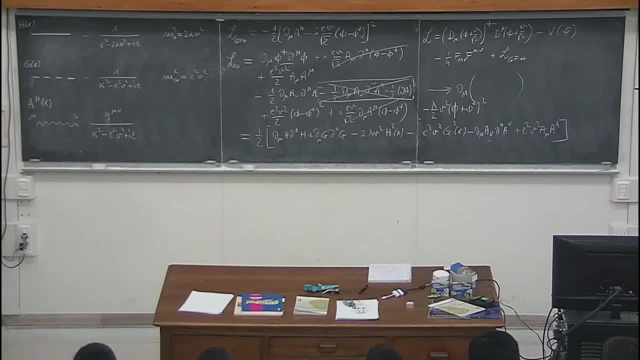 So the Golston boson is massive as a consequence of the fact that this is not a global symmetry. This is not the breaking of a global symmetry, but it is the breaking of a local symmetry And the Golston boson which would be massless. 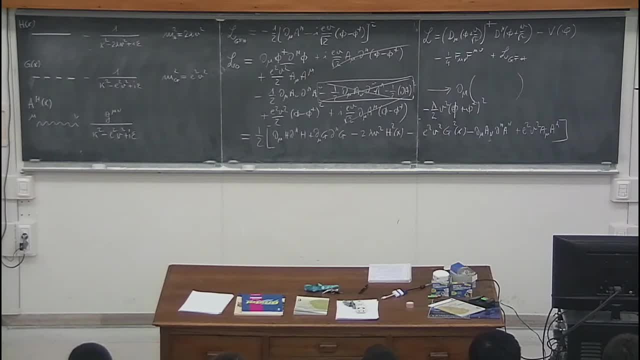 in the case of the spontaneous breaking of a global symmetry here has a mass. Actually, its mass depends on the gauge fixing terms, because the quadratic term appears here And we will see that actually, in the case of spontaneous breaking of the gauge symmetry, 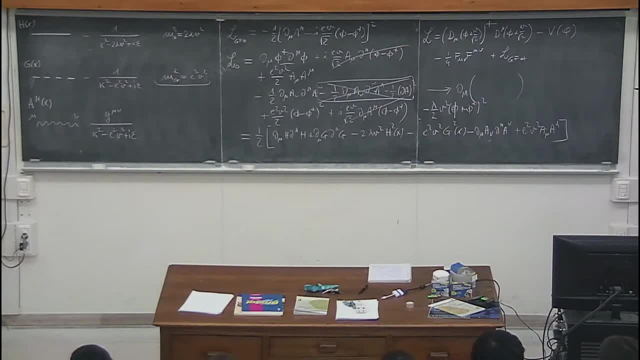 the Golston boson are unphysical degrees of freedom. We will get rid of them. So the situation is different. with respect to the case of global symmetries, which you have seen yesterday. Okay, am I forgetting something? I don't think so. 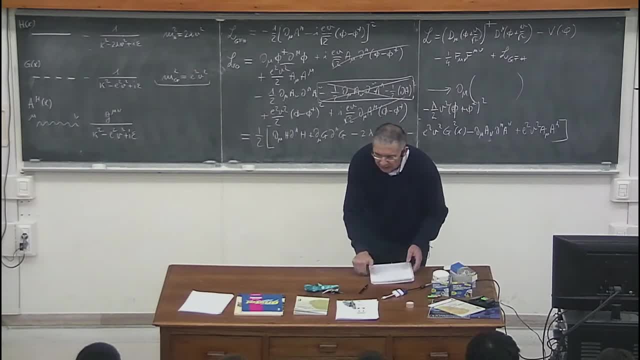 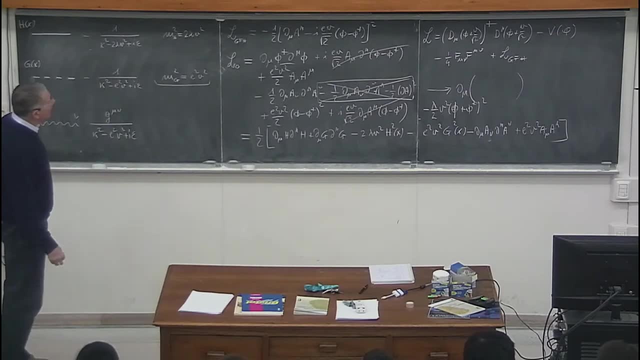 It's fine. So one of the problems I've listed at the end of the first part is now solved in principle If I introduce scalars in the theory and I realize the gauge symmetry in this Nambu-Golston way. 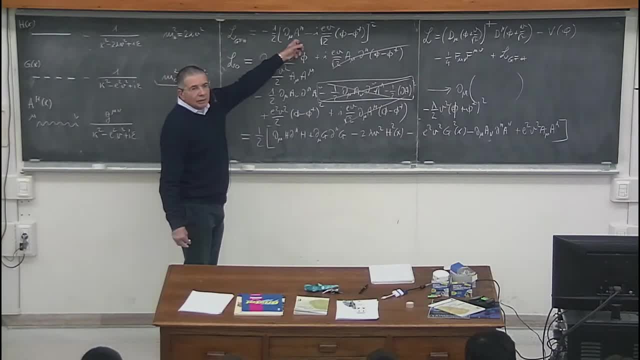 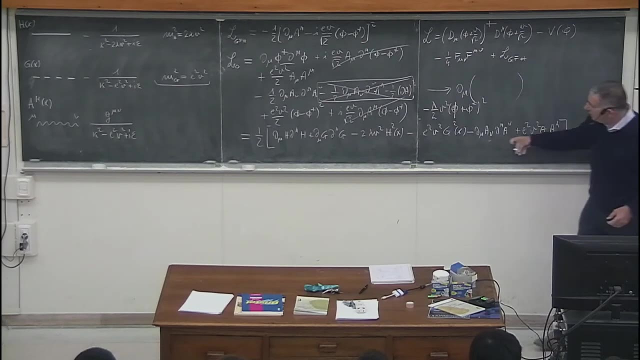 it so happens that a vector field, a gauge vector field, acquires a mass term which is now compatible with gauge symmetry, in the sense that it is not gauge invariant, but its gauge transformation is compensated by the transformation of other terms in the same Lagrangian. 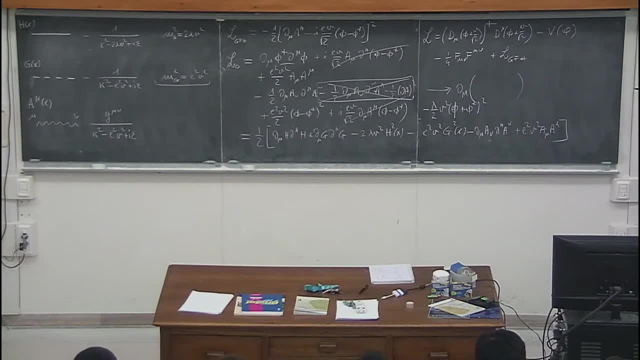 And the global thing is in fact invariant under the gauge transformation. So I have absorbed the variation of the mass terms into the variation of something else by means of this mechanism. We have half an hour so we can go on and write down the interaction terms. 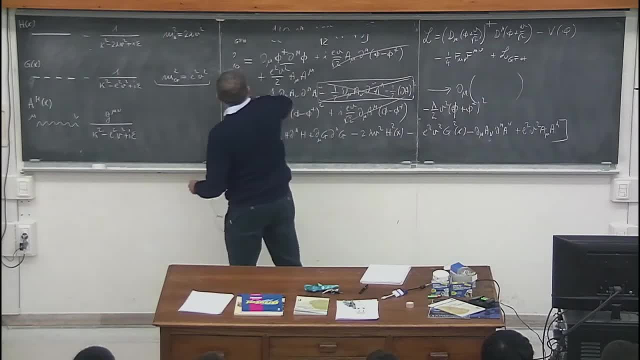 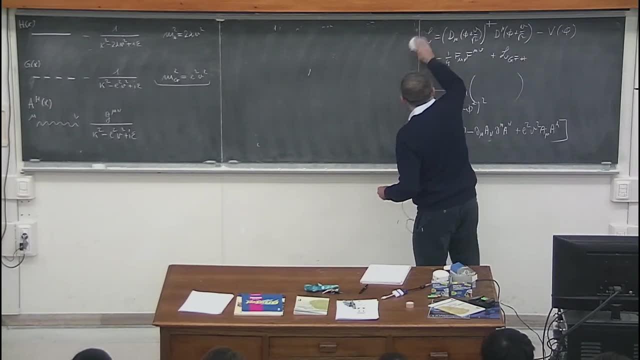 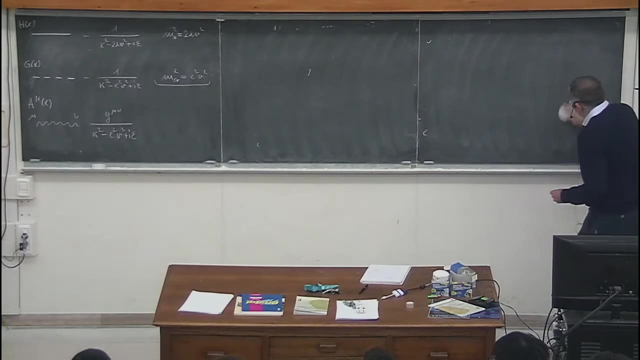 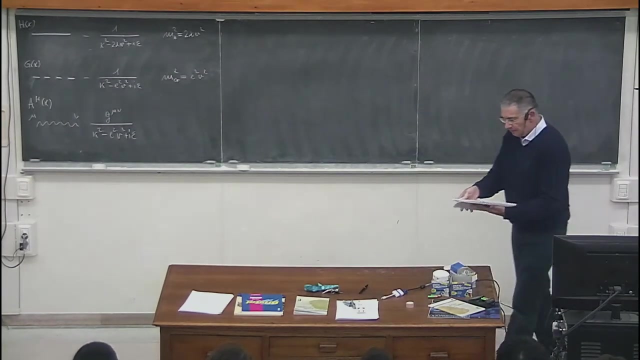 Let me. I want to study this model in some detail, because it is a simple way of seeing how the physical content of the Higgs model is composed. Then we will extend it to the standard model in an easy way. So what is the interaction? Lagrangian? 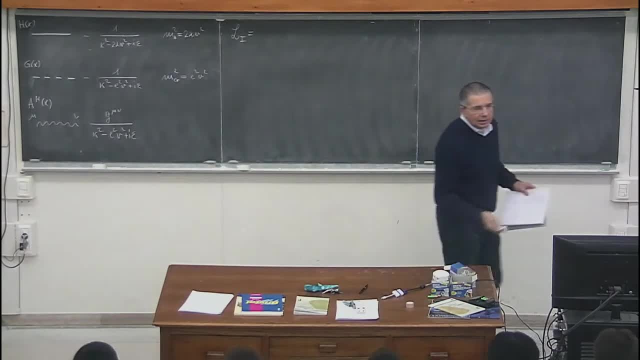 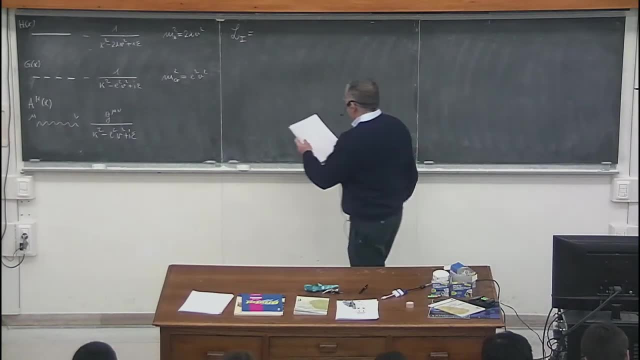 The interaction. Lagrangian is all the rest, all terms which are not quadratic in the fields. So it is just a matter of algebra to work them out. Let me write them down. There is a term which corresponds to the interaction of the vector field with the scalar field. 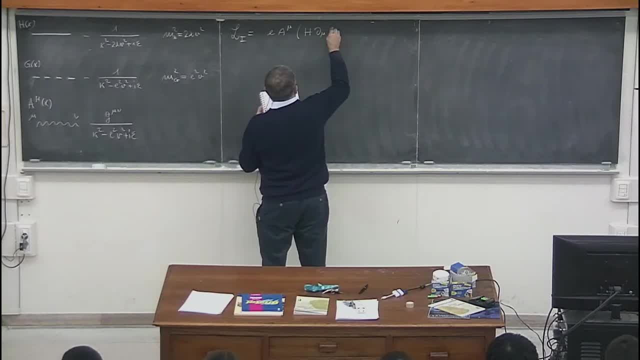 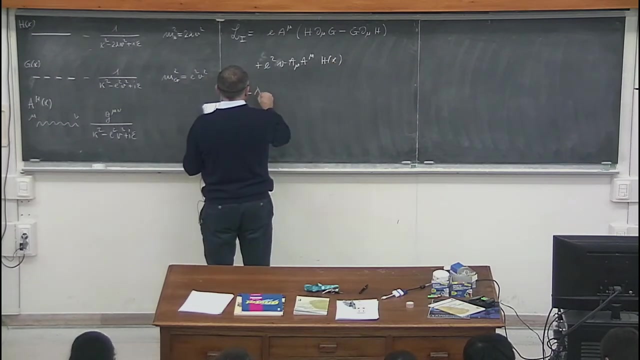 And this term is like this: h d mu g minus g d mu h. And there There is a term like this: plus. I just list them right and down. There is no particular difficulty in working them out. Thank you. 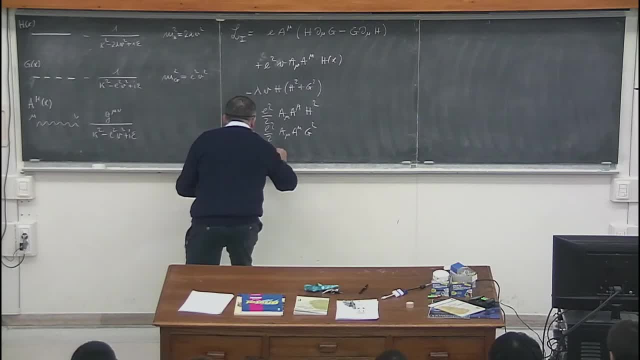 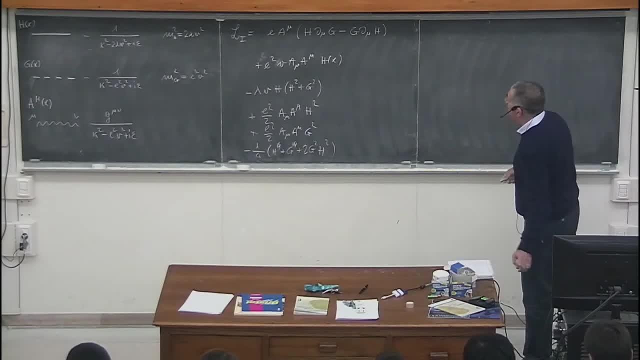 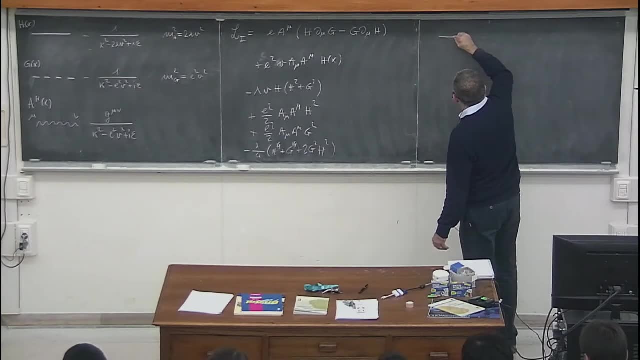 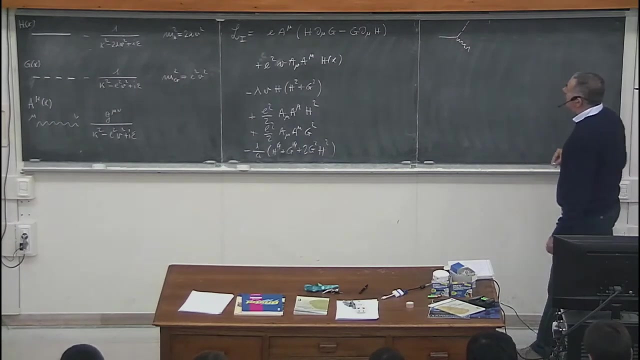 are derived as usual. for example, this first term gives rise to an interaction term which I represent like this: a trilinear vertex with a Higgs line, a Goldstone line and a vector line insisting on it. there are momenta here because of these derivatives and if I take pH and PG to be both incoming. 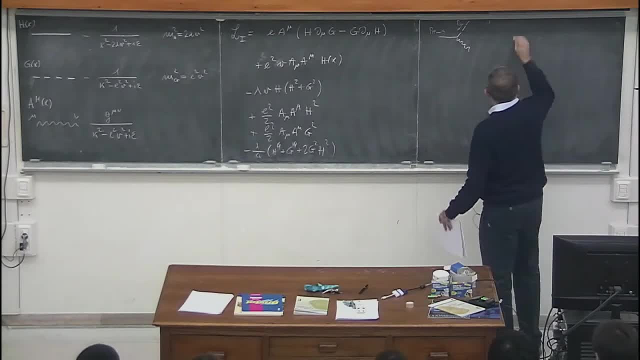 momenta. the Feynman rule is I e PG minus pH. you know how to get this Feynman rules from the Lagrangian density. you just take the virtual amplitude. you take the amplitude with corresponds to free particles as final state. you assign direction to the to the. 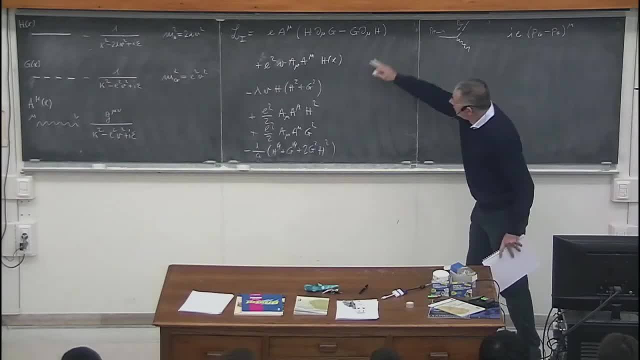 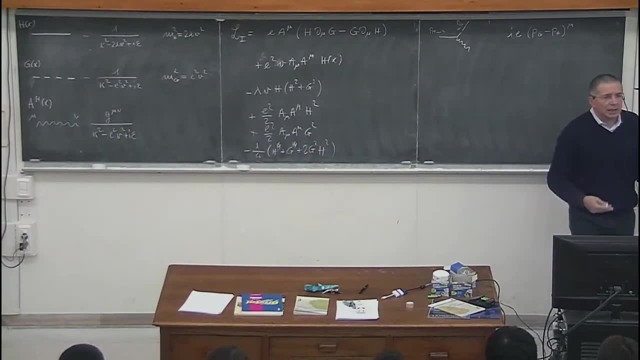 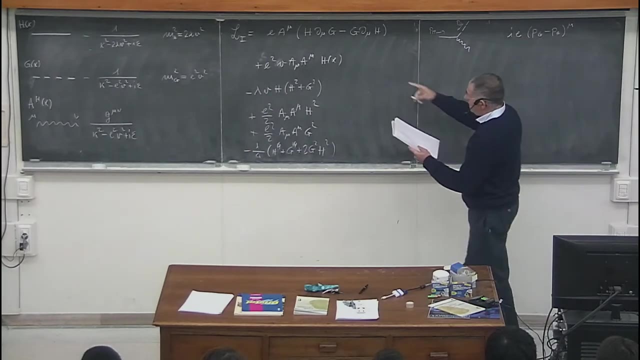 moment, and that's it. we have no other term. so the rest is just a matter of computing the combinatorial factors. there are different ways of attaching external lines to the vertices. it's very easy, so let me just write them down. this term here is a solid line with two vector. 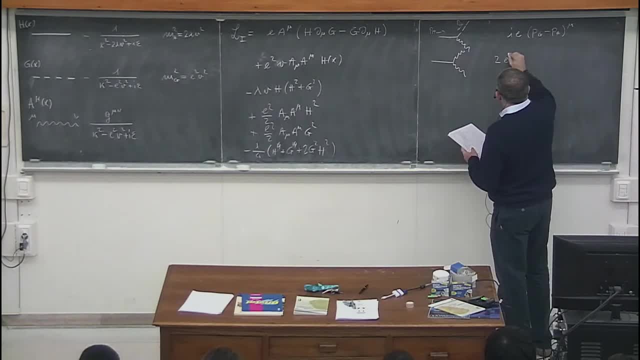 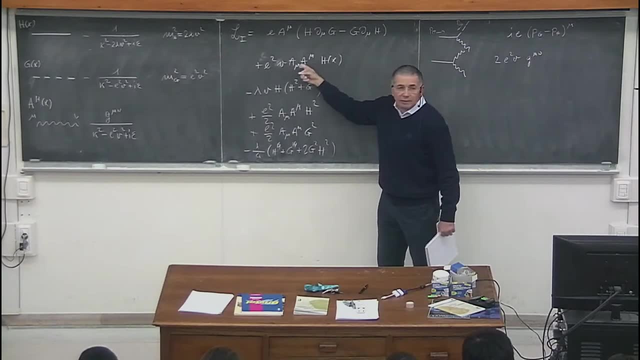 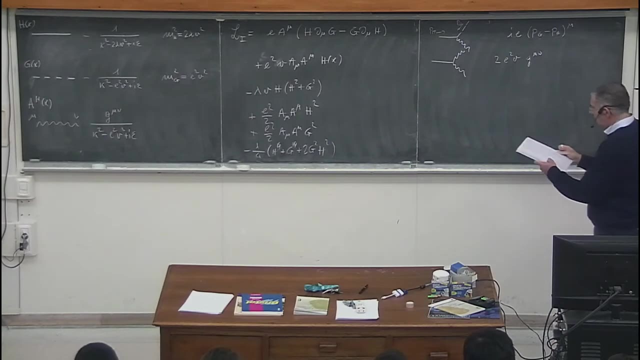 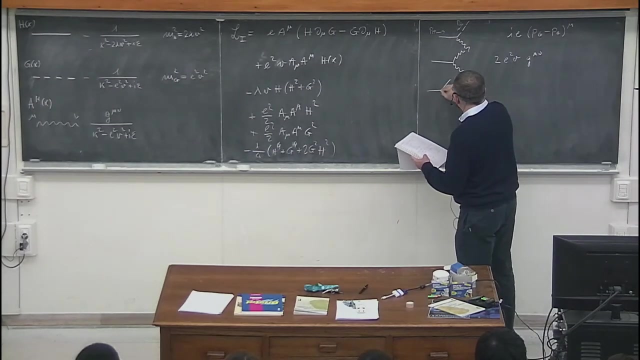 lines and the corresponding Feynman rule is 2 e square V times g mu nu. g mu nu is because the two polarization vectors of a mu are saturated with each side with each other. then I have a three linear vertex like this, which is minus six, and: 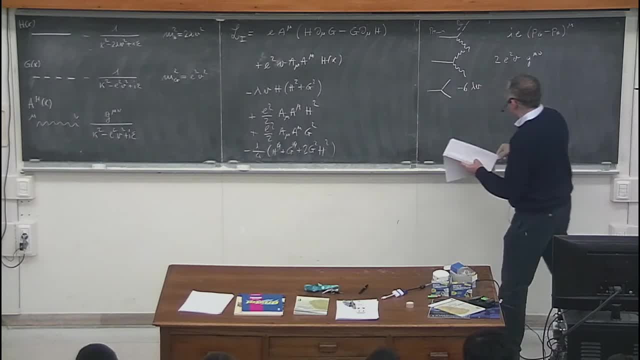 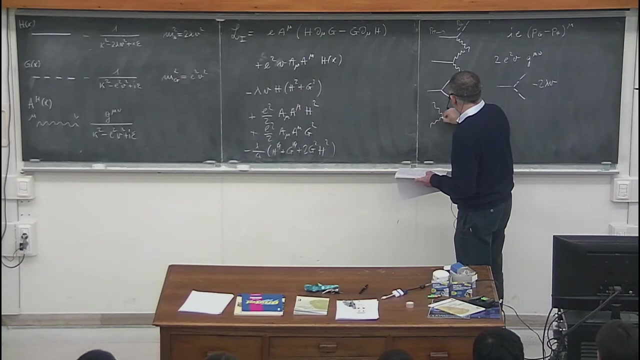 aestones right here and here they are, the four� io and the pishta this is called. that's very complex, then. what it means is less partialthood. our method is: plus to the red is equal to plus the red hundreds of the whole. 好 enough, very apple of z. lambda v: 6 is three factorial. then i have vertex like this to Goldstone and one: Higgs is minus two. lambda v: the factor of 2 comes from the two possibilities of attaching the two Goldstone lines. then i have this one. this is likeiem. lambda v a factor of 2. it comes from the two possibilities of attaching the two Goldstone lines. then I have this one: this is like this and this is like this, and this is a three standard. Goalt коп scores. is is a three standard one. this is a three standard. 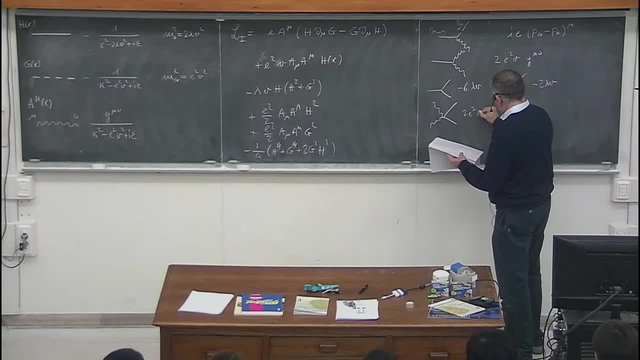 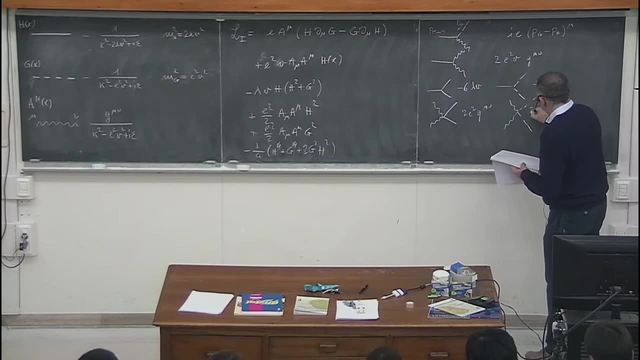 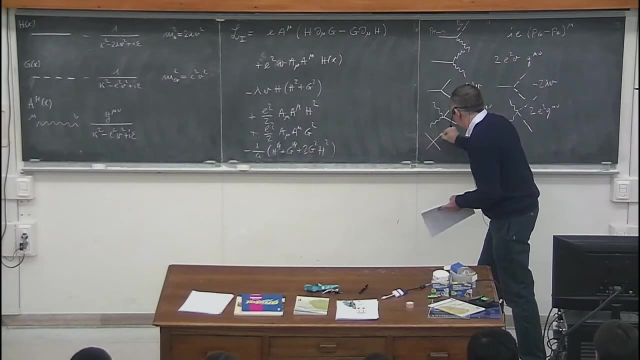 is 2e2 g mu nu and I have this one which is also 2e2 g mu nu and finally, I have minus 6 lambda for the 4-Higgs vertex, minus 6 lambda for the 4-Goldstone vertex and minus 2 lambda. 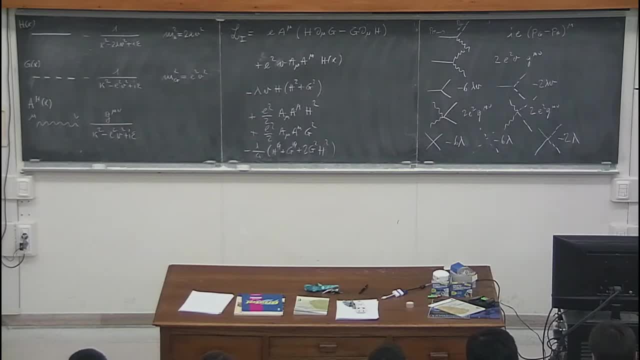 for the 2-Higgs- 2-Goldstone vertex. So this is the complete set of Feynman rules for the scalar QED model, for the Abelian-Higgs model, which is how it is usually called, in the Toft-Feinman gauge. 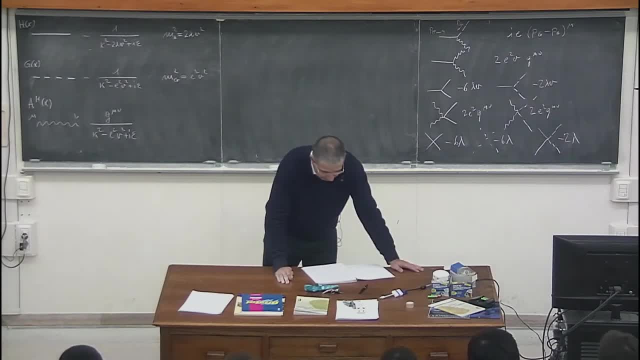 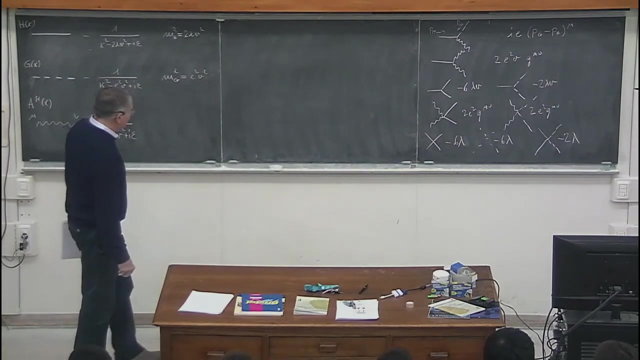 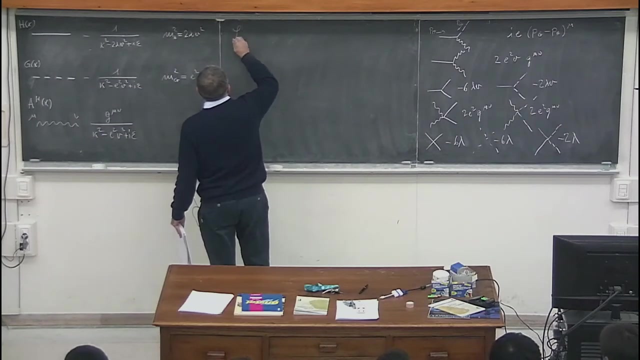 Well, there is an observation which we will reserve for the discussion session. We will need these Feynman rules at some point. Let me now tell you something about the physical content of this theory. So let's see, Let me go over here. 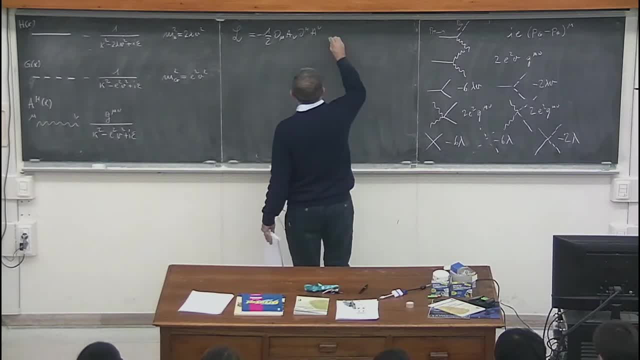 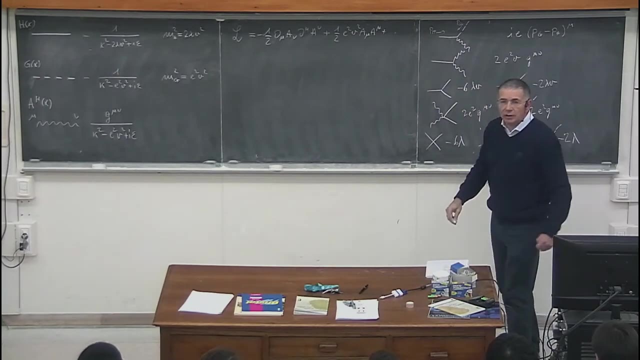 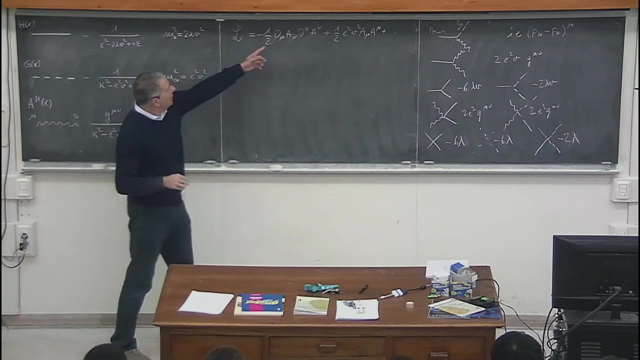 So let me first concentrate on the free Lagrangian for the vector field which has this form. you will agree with me that this is just the sum of four terms which are similar to the free Lagrangian of four real scalar fields, for example. let me write it explicitly: 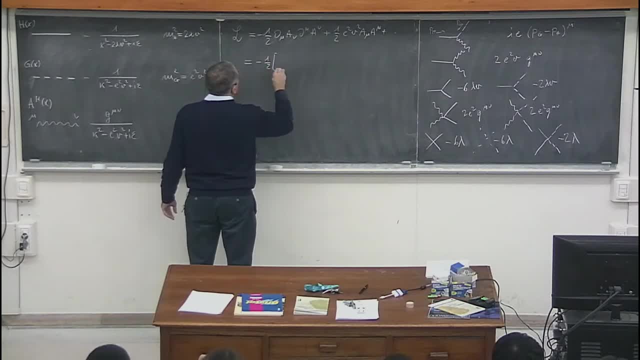 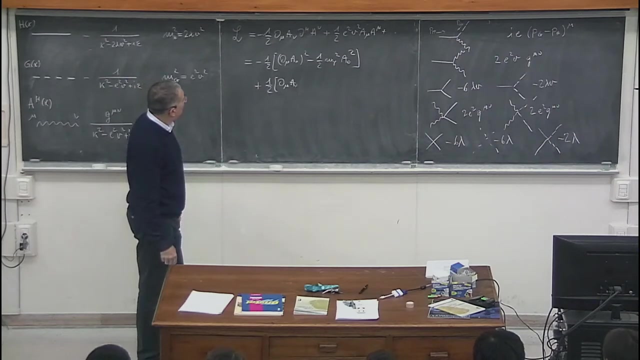 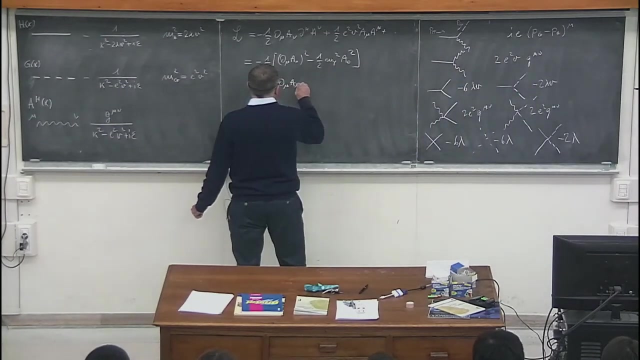 it is minus one half times d mu, a0, square minus. sorry, they are mixed by Lorentz transformation. I agree, but after you have mixed them by Lorentz transformation you can say the same thing of the transformed fields. so these are four Lagrangian for four distinct scalar fields. 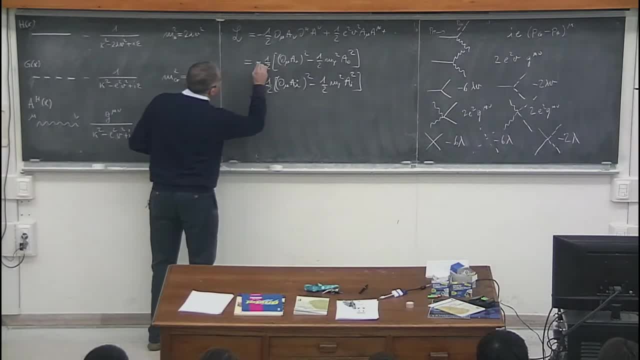 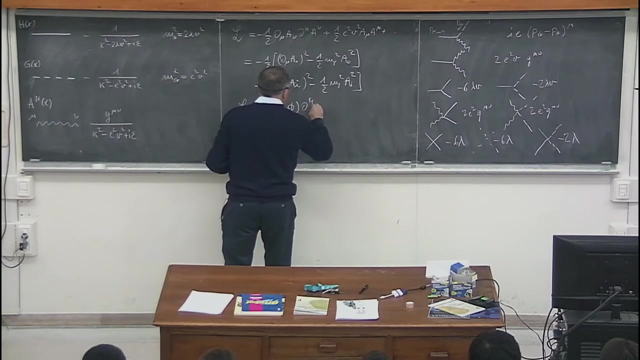 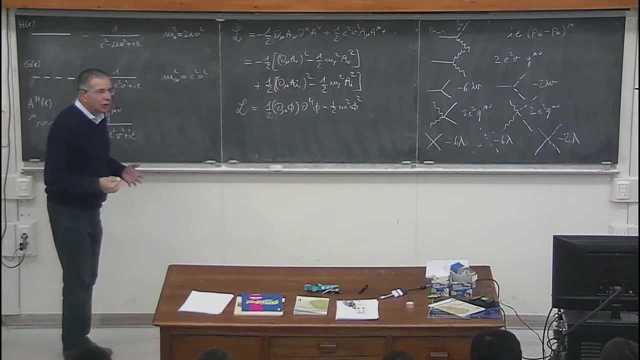 with the only difference that this component, the zero component of the vector field, has a minus sign in front of it. a minus sign in front of the Lagrangian means you remember how you quantize a scalar field. right quantization of a scalar field goes through the definition of. 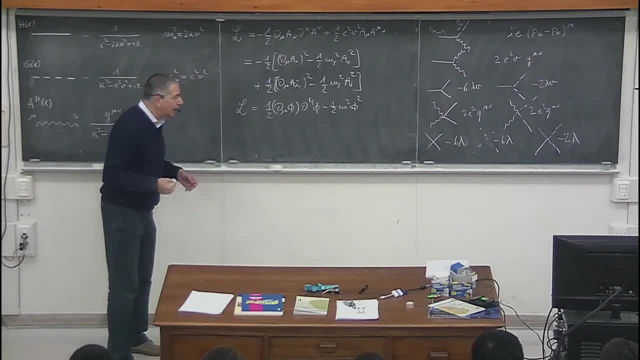 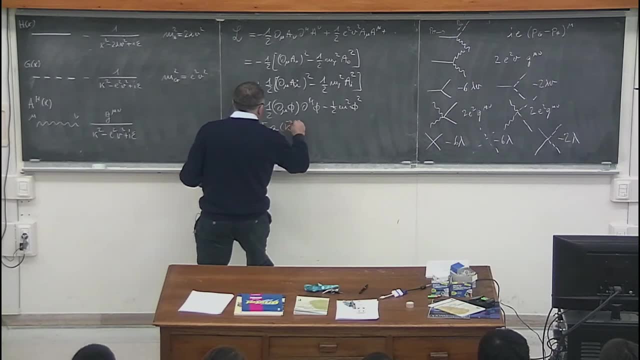 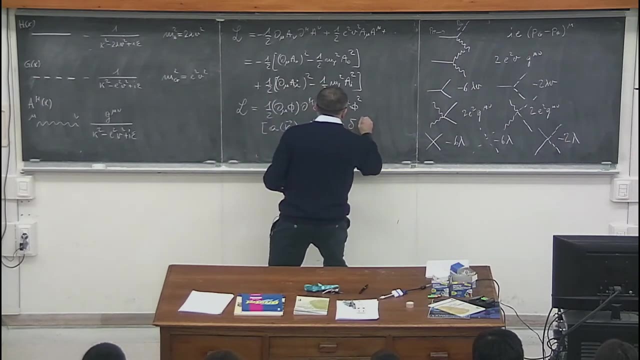 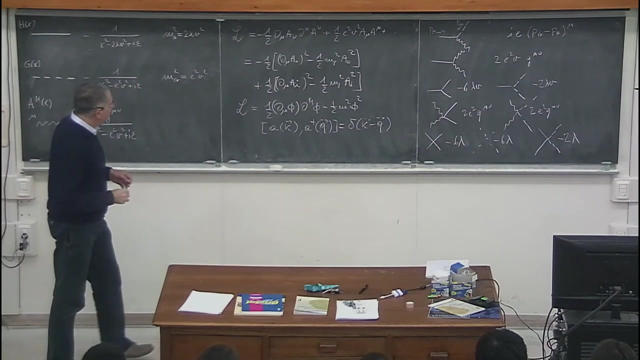 creation and annihilation operators. and the creation and annihilation operators obey commutation rules. and the creation and annihilation operators obey commutation rules which are: a of k, a dagger of q equal to delta k minus q. right now, if I change l into minus l, 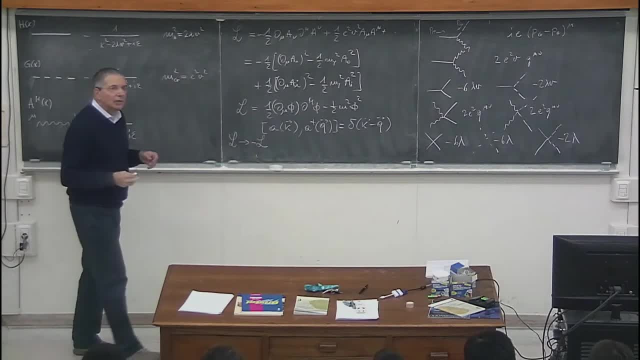 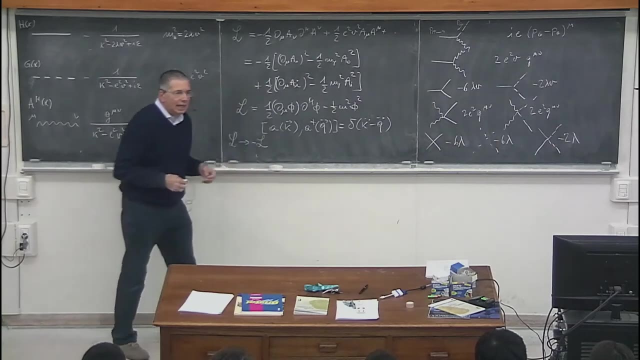 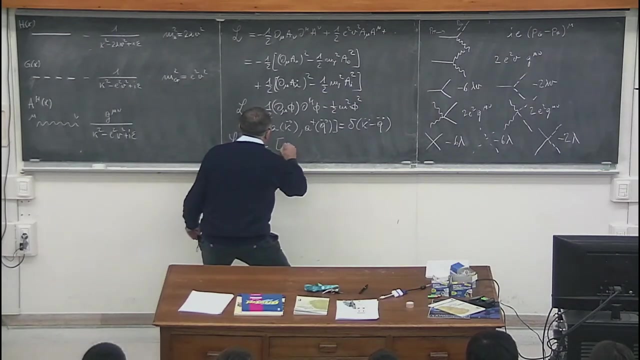 if you recall classical mechanics, this amounts to changing the sign of p of the conjugate momentum. and if you change the sign of the conjugate momentum, this is equivalent to switching a and a dagger. so if you have l transformed into minus l, what you get is a commutation relation. 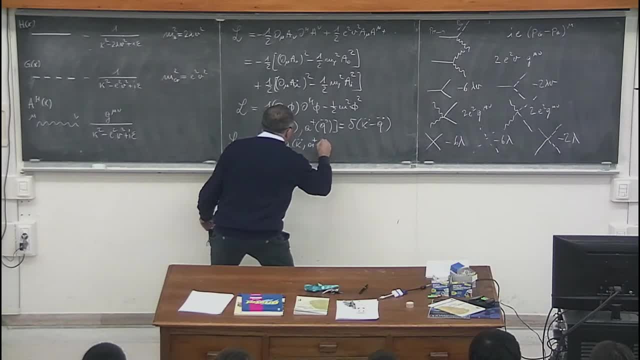 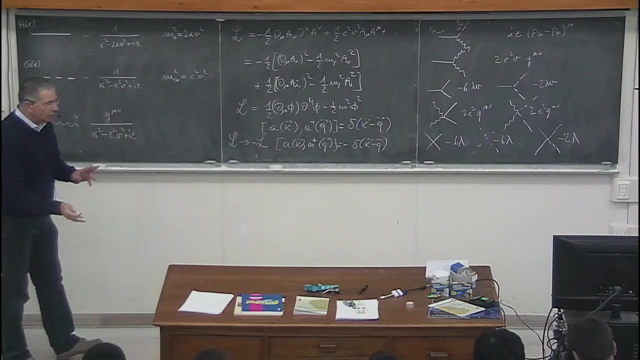 which is a k a dagger q, equal to minus delta k minus q. because changing the sign of the conjugate momentum, which is a k a dagger q, equal to minus delta k minus q. because changing the sign of the Lagrangian is equivalent to reversing the sign of the conjugate momentum. 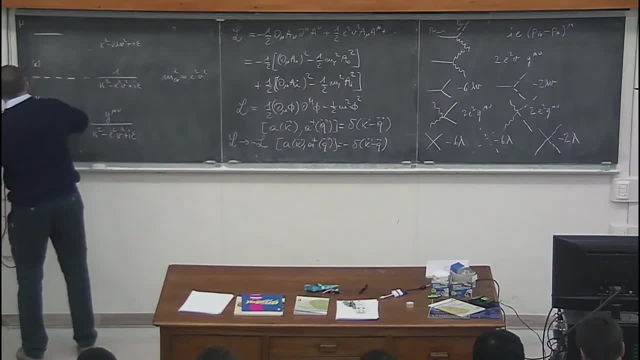 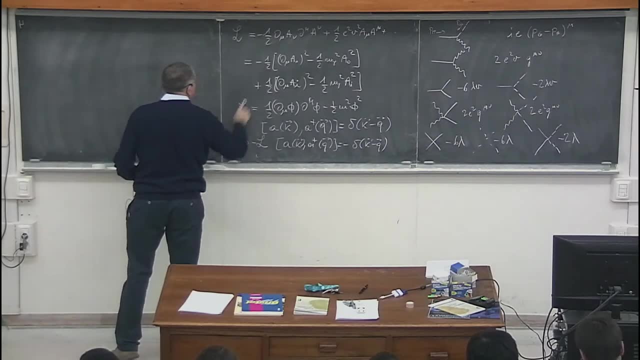 so I can write the free field solution of the equations of motion for the vector field, a mu like this: a mu of x. I can do it by mimicking the free field solution of a scalar field, of four scalar fields. I can do it by mimicking the free field solution of a scalar field. 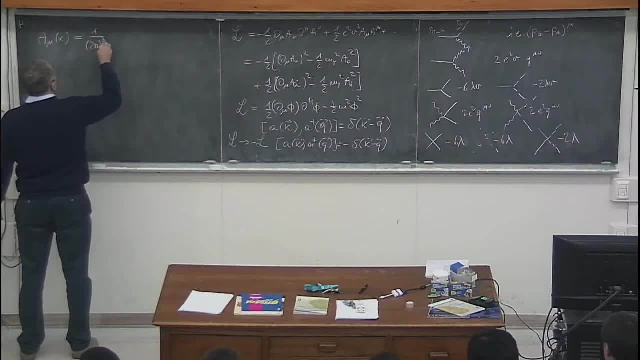 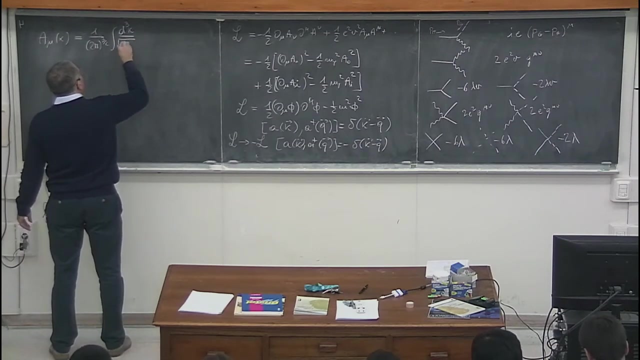 which I write like this: one over two, pi to power three halves, which is conventional to get some given normalization of the commutation relations: integral over the three momentum k divided by two, the energy associated with three momentum k times the destruction annihilation. operator a which carries an index b. 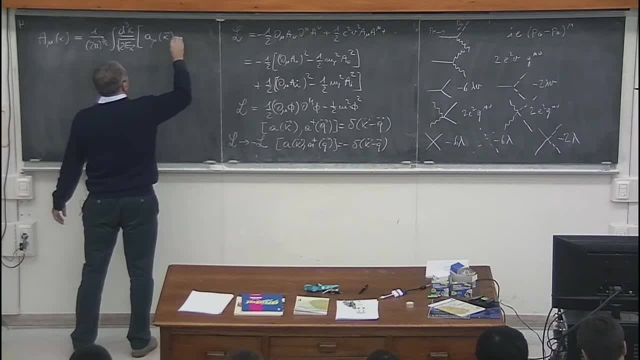 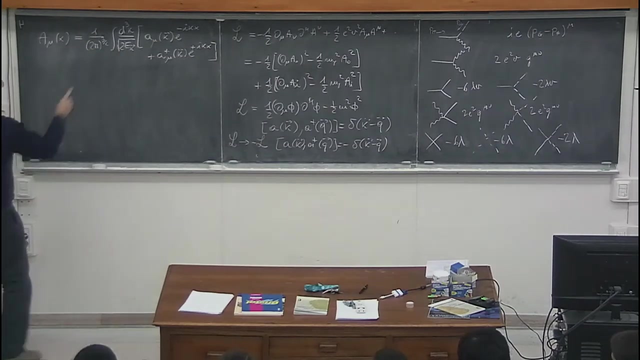 which carries an index b. which carries an index b and which is a function of k times the propagating plane wave: e to chi minus chi x, plus the emission conjugate, plus a dagger mu of k, e to plus i, k, x, the energy is plus root of k. 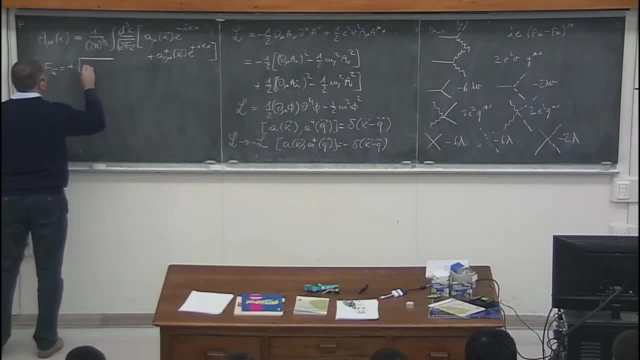 plus a dagger mu of k? e to plus i k x. the energy is plus root of k? e to plus i k x. the energy is plus root of k? e to minus i k z. plus a dagger mu of k? e to plus i k x. minus l of e of tangent r. 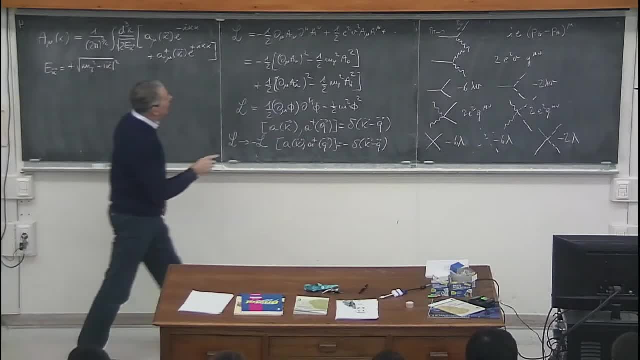 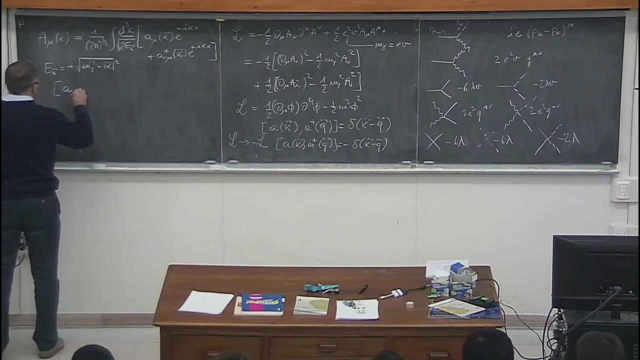 minus e k x plus a dagger mu of e to plus l of ru and the commutation relations between and the commutation relations between a and a dagger are like this: a mu function of k a ru emissions. I'm so Ahora diet charming- are so annoying. 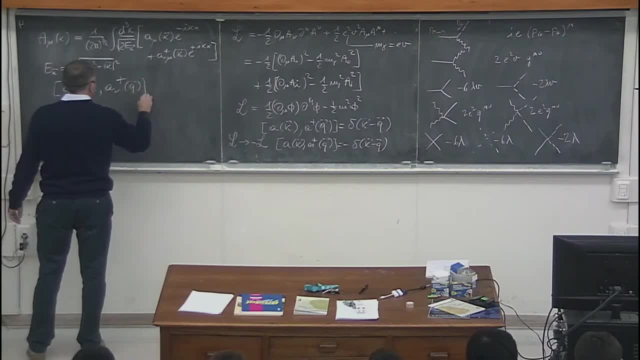 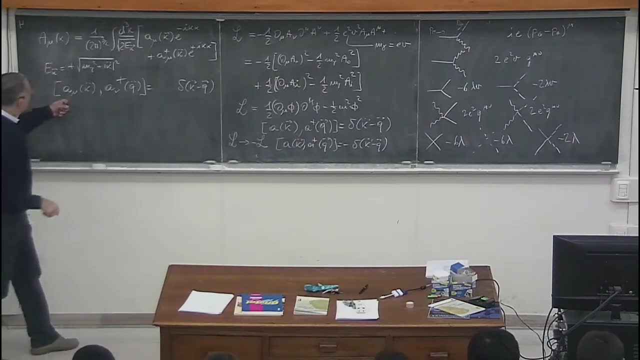 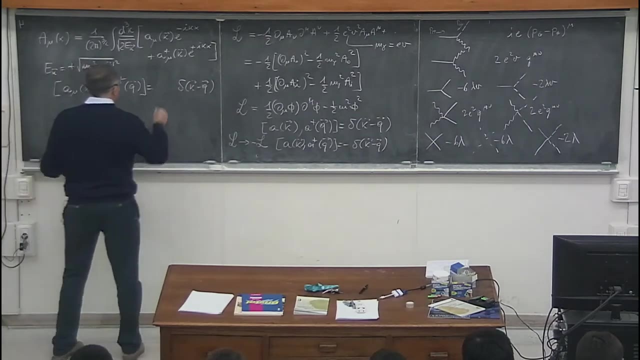 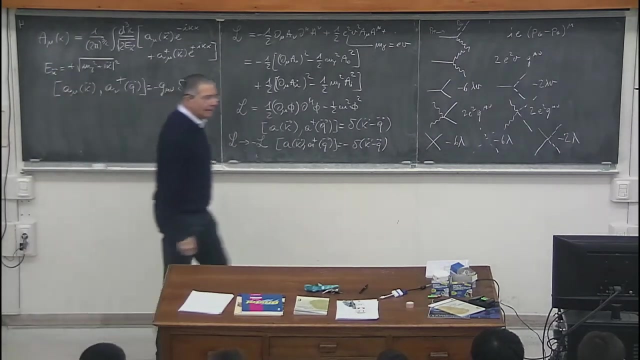 green ancient. we know what dark, I know what dark function of q. this is equal to delta k minus q, with a minus sign when mu and u are zero and a plus sign when mu and nu are equal and spatial. so this is minus g million. yes, no, i don't. 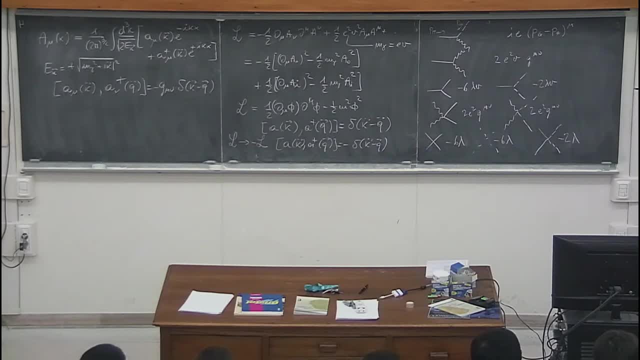 no, no, no, i i don't sum at all. there is no sum in the derivation of the final rules. if you have vectors, boson lines, as external lines, you have to saturate them with a polarization vector, and i haven't said anything about this polarization vector so far. but there is no sum here. 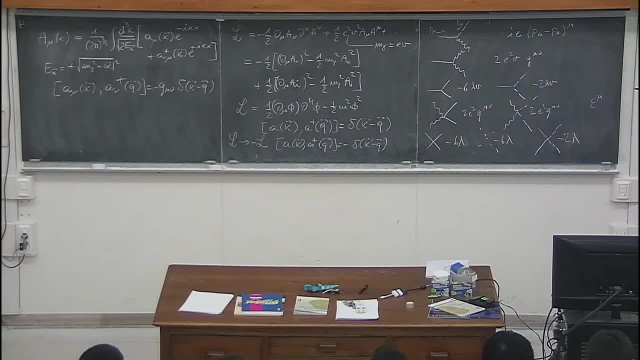 i'll. i will show you in a moment, just just a second. i still have the goldstone. i'm going to show you what happens with the goals. so these are the commutation rules for the annihilation and creation operator for the four components, four components of the vector fields. 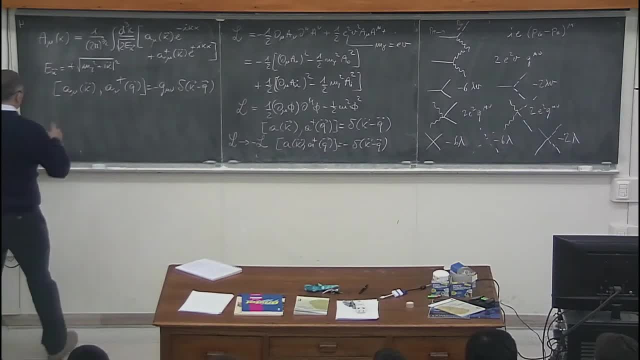 now it is convenient to expand each of these four vectors in a basis which depends on k, which means that i will write a mu of k as a linear combination. a sum over lambda and lambda goes from zero to three. there are four different directions in the space. 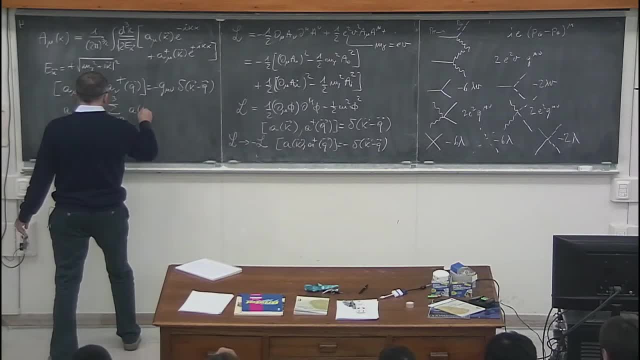 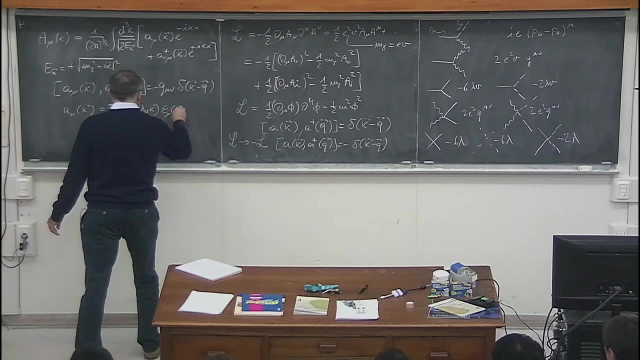 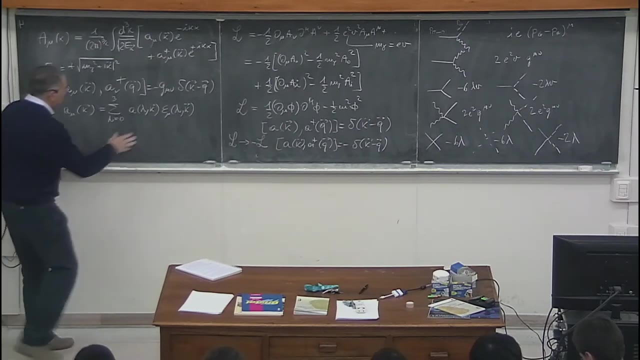 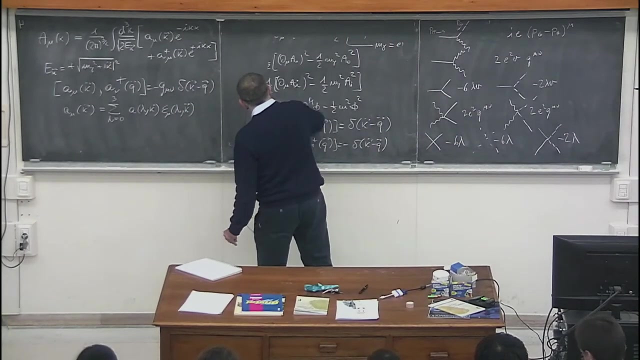 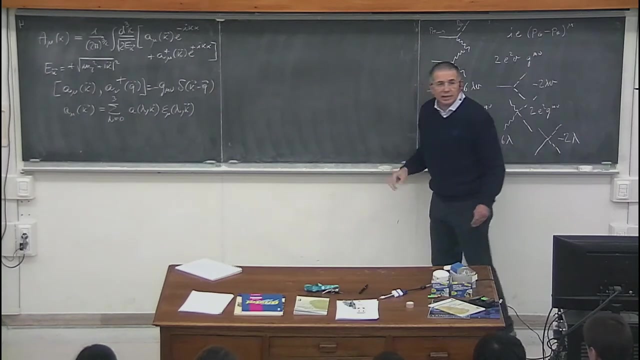 of a function of lambda and k times a polarization vector which i call epsilon mu, which is a function of lambda and of k, and i can choose the polarization vector like this: since the vector is now massive, i can go to its rest frame and choose the four polarization vectors: epsilon mu. 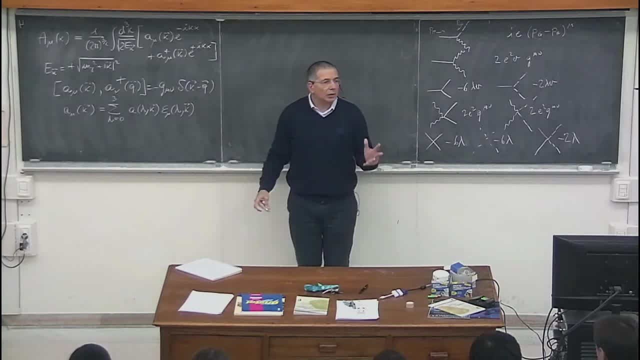 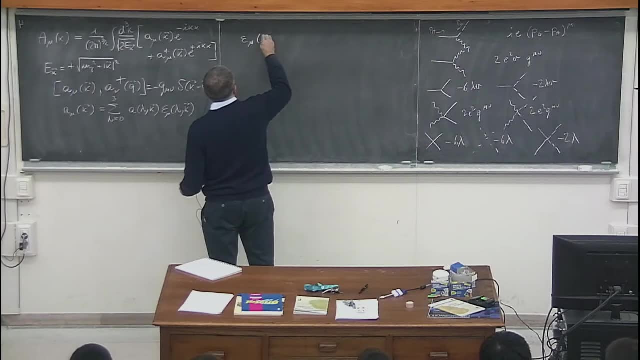 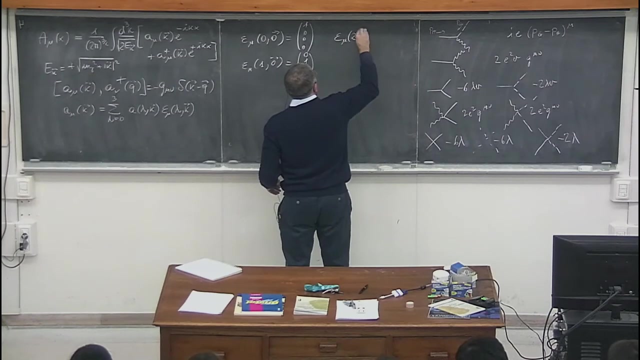 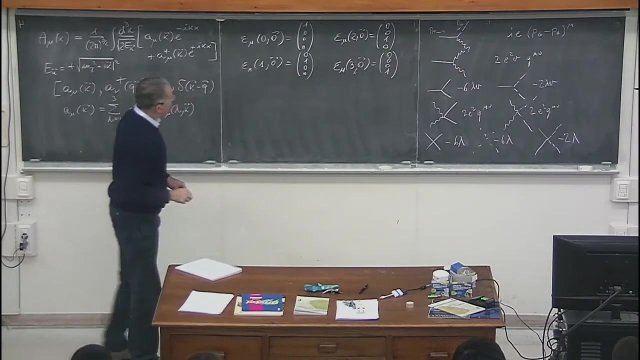 of lambda in the rest frame as the four unit vectors in the four directions. so i will choose epsilon mu of zero in the rest frame. the second zero is the three momentum as the vector one. zero, zero, zero. Epsilon mu 1, 0.. Epsilon mu 1, 0. 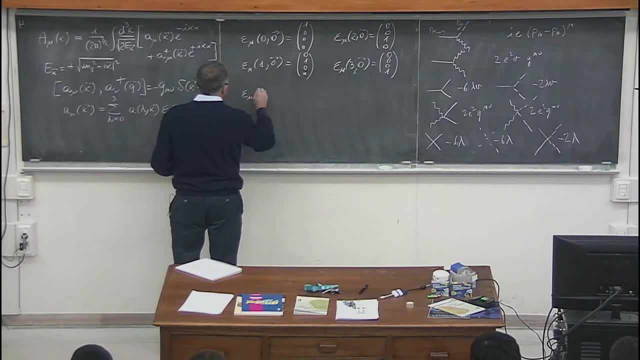 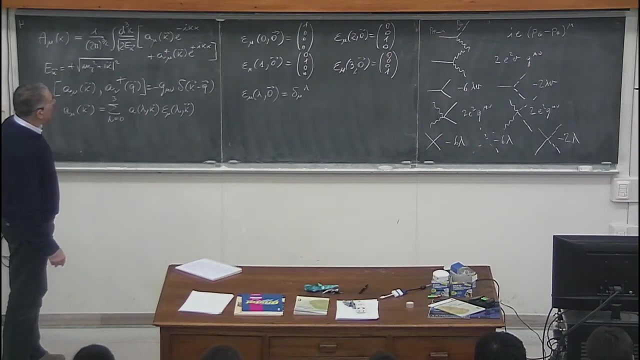 Which means that epsilon mu of lambda in the rest frame is just equal to delta mu lambda. right, There's only one component which is non-zero, which is like this: And after I have defined the four-polarization vector in the rest frame, I can get epsilon. 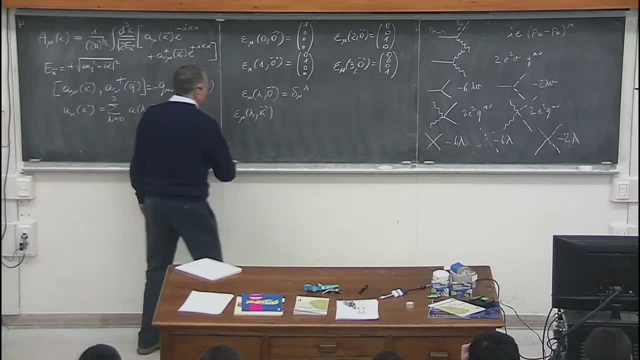 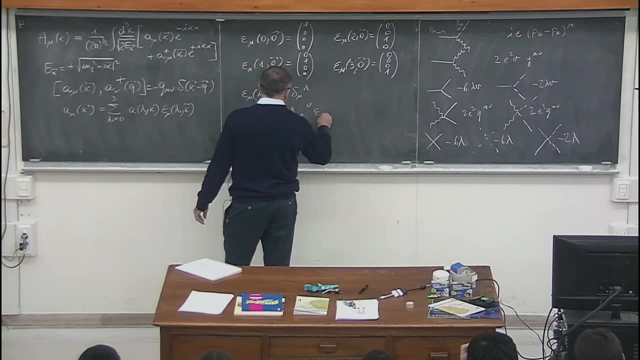 mu In the frame where the vector boson moves with the momentum k by simply boosting them. lambda is the Lorentz transformation which is a function of the momentum times. epsilon mu of lambda: yes, 0.. 0.. 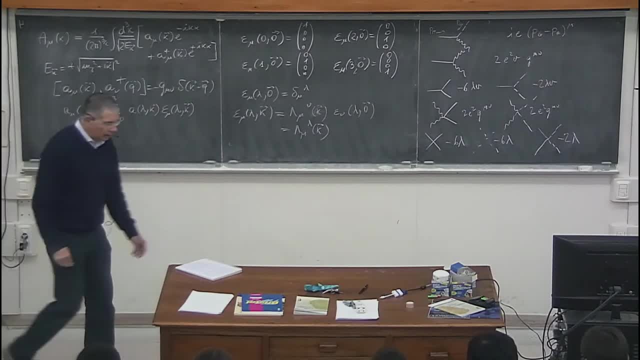 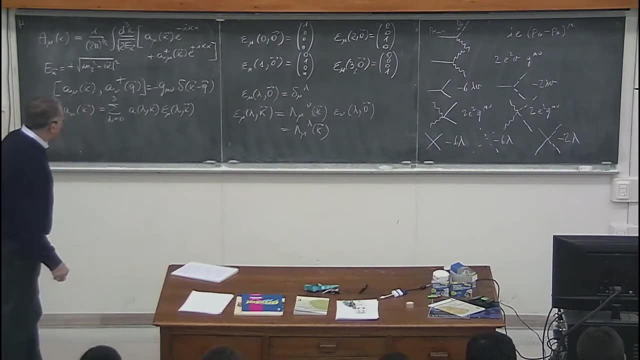 Which is equal to lambda, mu of lambda. OK, And if I do that, I can write this: relations in terms of this, I just replace each 0. And if I put one there, I just replace the 0. 1.. 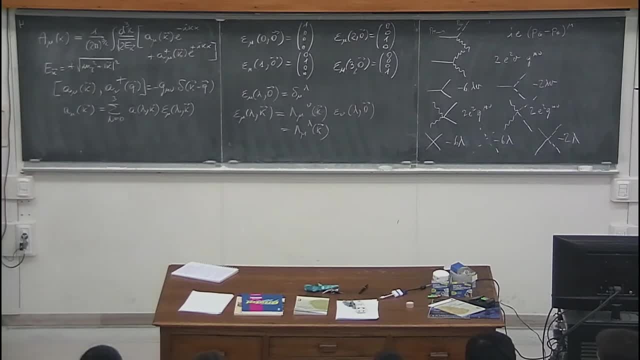 1., 1., 1. 1. 1. mu by its expansion over the basis of the polarization vector defined in this way. and then I just use the properties of the Lorentz matrices. I have to erase this beautiful Feynman rules. I will rewrite them when we need it. and what I 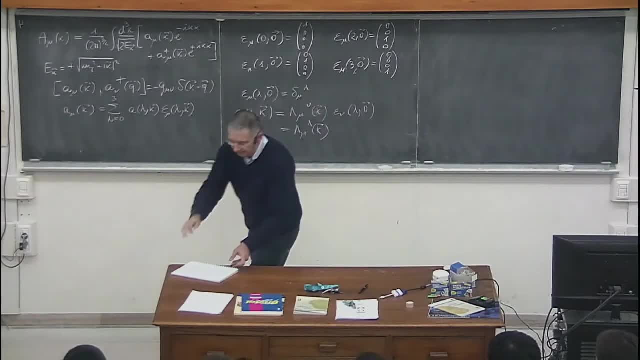 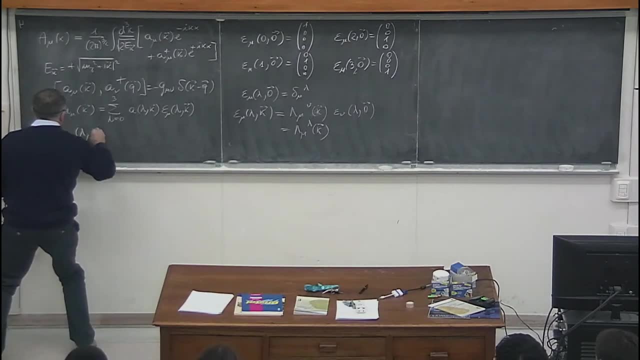 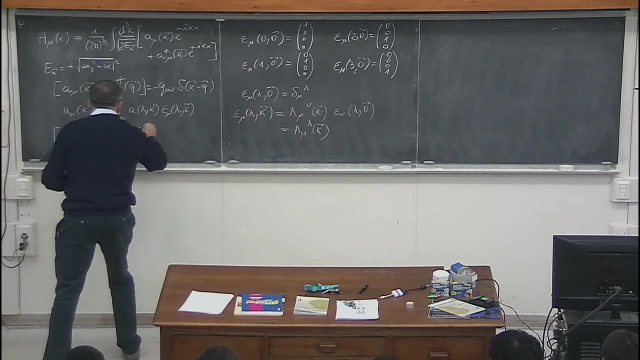 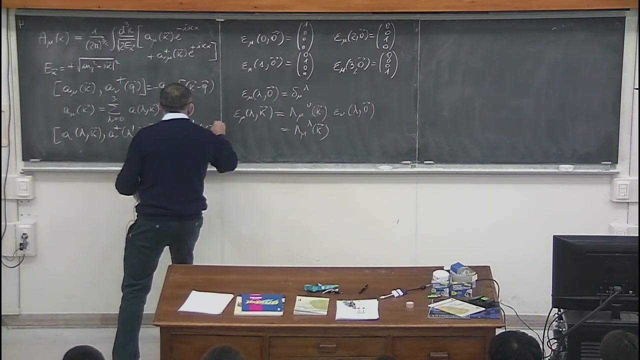 get is a lambda K commutator with a dagger lambda prime Q equal to minus. where is it minus G? lambda lambda prime Delta K minus Q. sorry it's a bit boring, but it is important and we need it. we need to show what I'm going to show you. 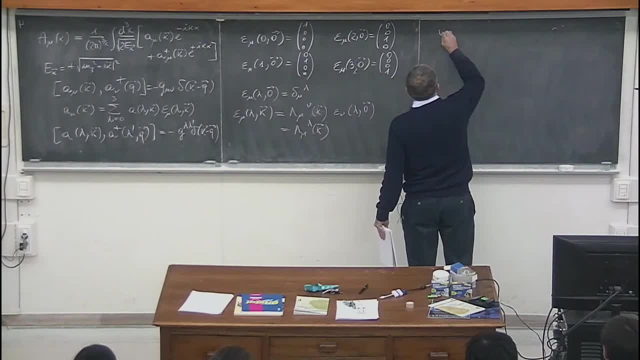 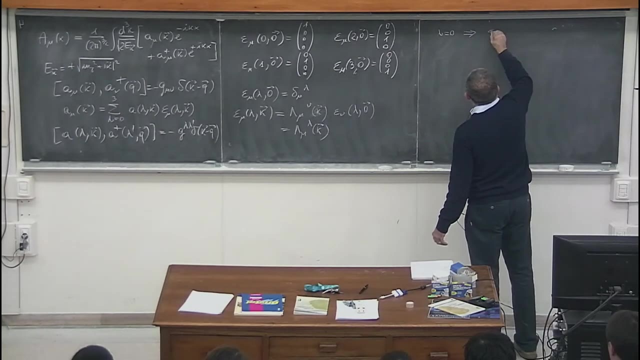 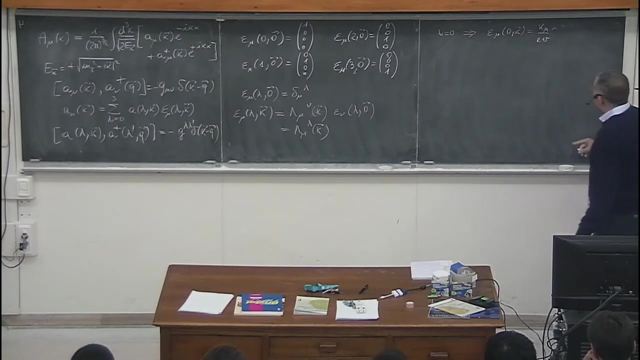 so let us concentrate on the polarization modes with lambda equal to zero. if I take lambda equal to zero, then it is easy to show that epsilon mu zero K is proportional to Kmu. It is in fact Kmu divided by the mass. this is easy to show because this is true in the rest frame. 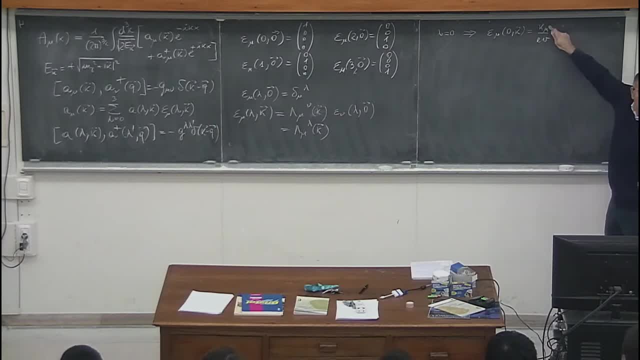 in the rest frame, vector k mu, as only the zero component, which is zero, I vegetable wanna show an example of this so we can explain it here. you form a signalticamente and everything will exist only in any two-ilahalμ, only 0 component. but it doesn't need to beelle Entre bar ف. you know the first two equations of. 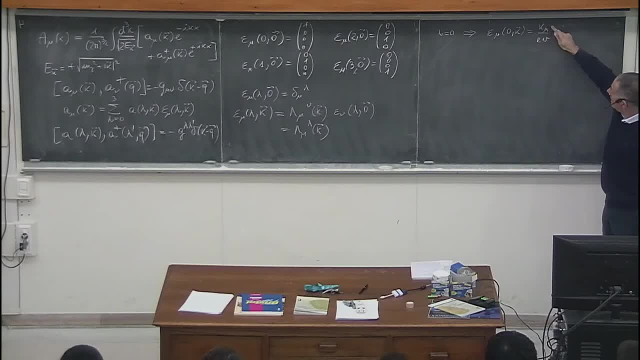 equal to the mass and zero spatial components. so this is precisely K? mu and since this is a covariant relation, this is holds true in any reference frame. so these modes with lambda equal to zero respond to a polarization which is longitudinal, which is parallel to the for momentum of the of the vector. 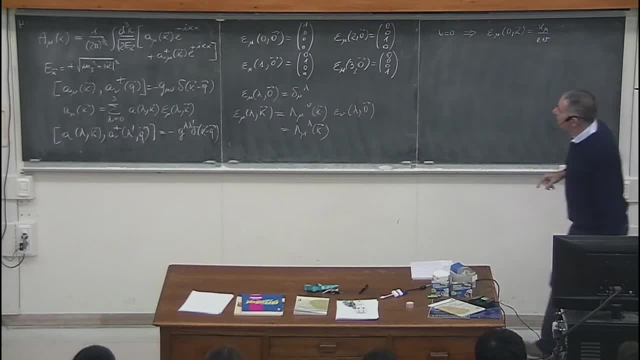 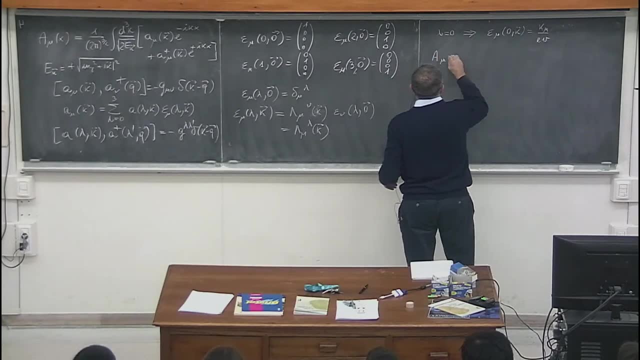 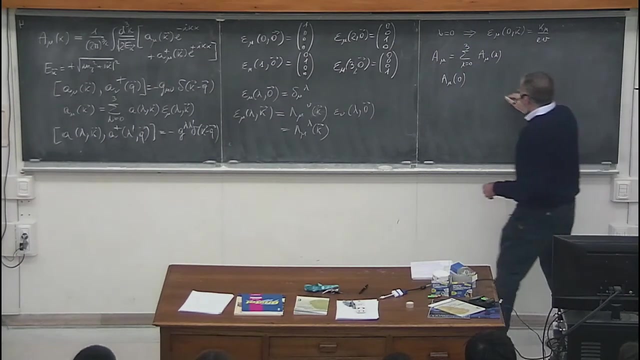 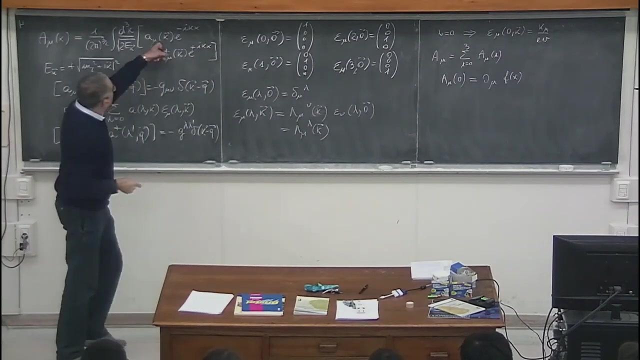 particle, which means that the corresponding field, if I write a new as a sum over lambda from 0 to 3 of a mu lambda, this means that a mu corresponding to polarization 0 is proportional to the derivative of some scalar field, because the polarization vector is K mu and if I plug K mu here, K mu times the 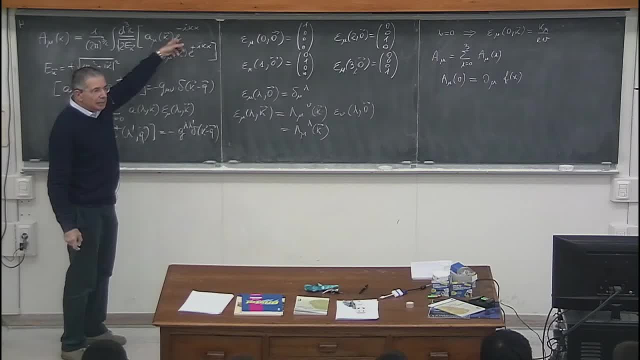 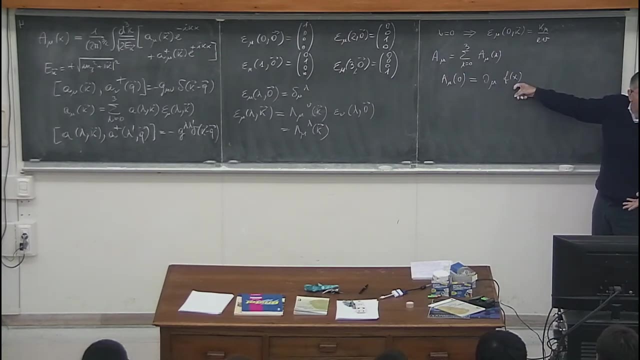 plane wave is the same as taking the derivative with respect to X mu. so the longitudinal polarization mode correspond to a scalar field, is a degree of freedom which correspond to spin 0, because it is entirely fixed by a scalar function. furthermore, this lambda, equal to zero degrees of freedom are those which have 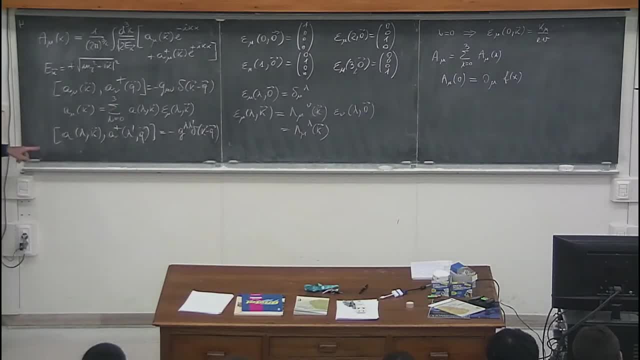 the wrong sign in the commutation relation. a of 0 K commutator a dagger: 0 Q is equal to minus Delta K minus Q and this means this implies, as I will show you in a moment, I have five minutes to make these important proof, but I will do it. 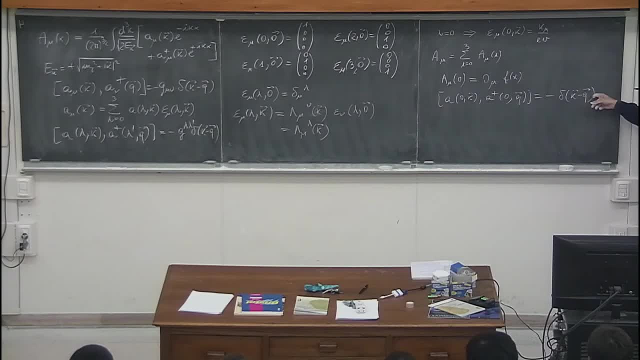 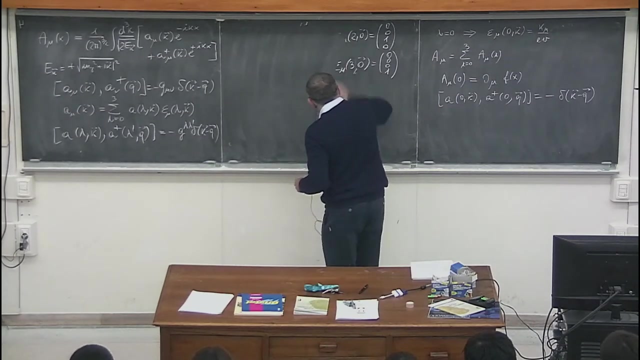 this means that the states, the physical state, the physical single particle states that you build out of these operation operators are states with negative norm, so they are unphysical states. they must be excluded from the physical spectrum. this is pretty easy to show because- well, of course, I have to. 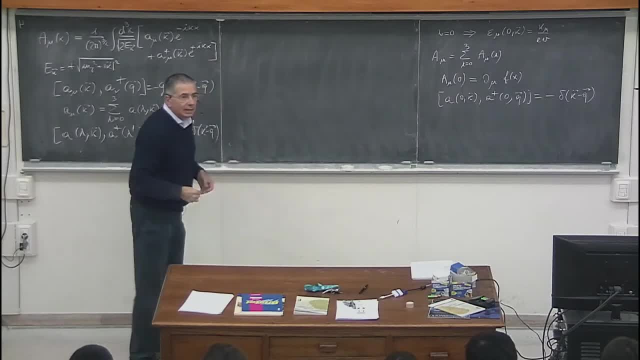 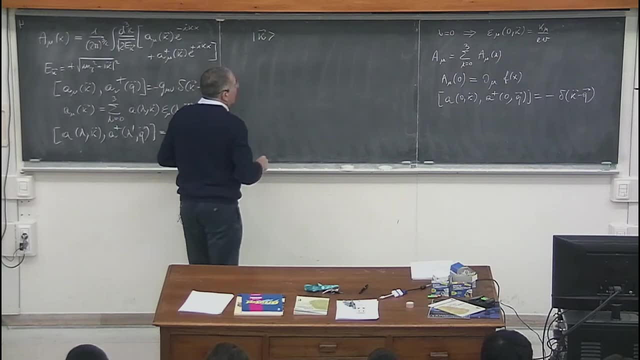 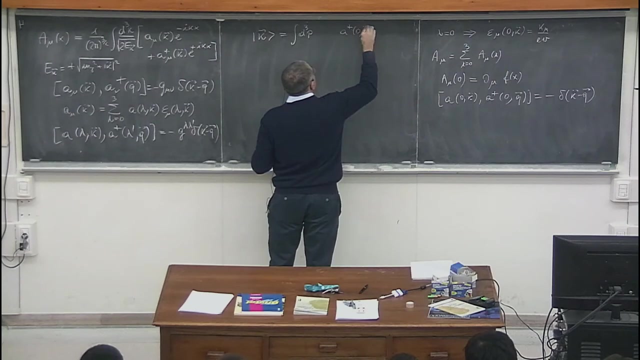 form wave packets because single particle states are plane waves. they are not normalizable. so let me define a state with momentum K built out the polarization lambda equal to 0, like this: it is an integral over three momentum, momentum p of a dagger zero p acting on the vacuum state of the theory. the state with 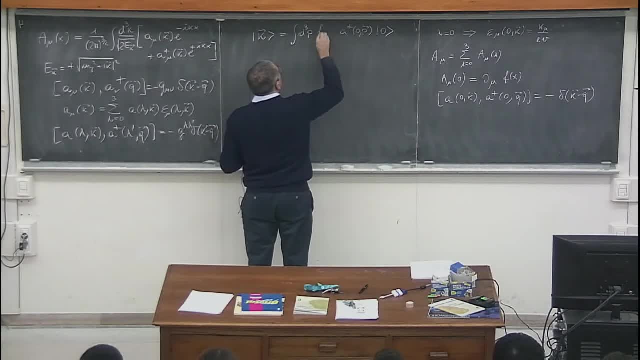 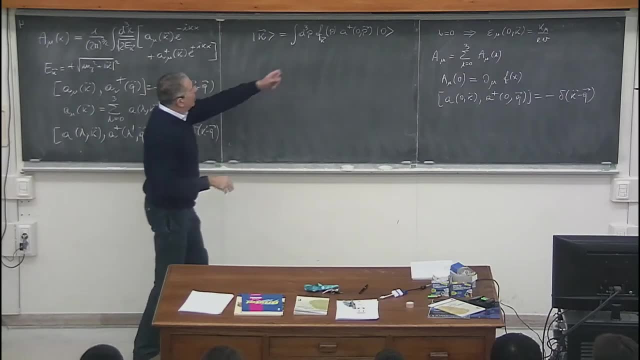 no particle times. a wave packet which I call f. This is a function of p, and this function of p has a strong peak around p equal k. This is a wave packet. This is something like a Gaussian, something like that. 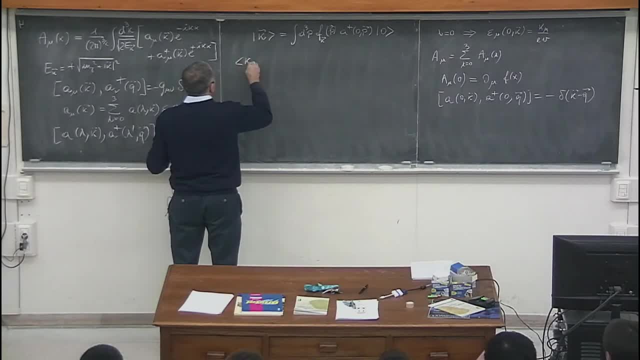 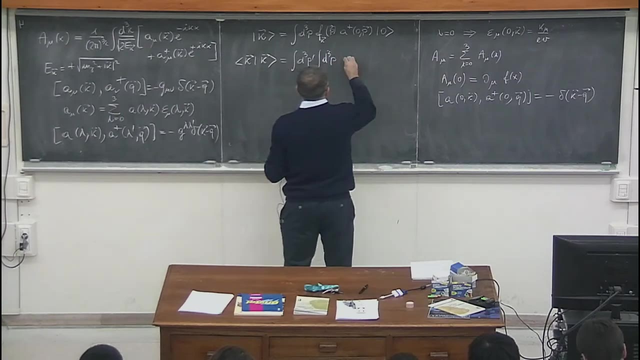 And now let me compute the norm of this single particle wave packet. This is easy to do. It is an integral over dp prime, integral over d3p f, complex conjugate peak around k function of p, prime, f, kp, and then I have a scalar product. 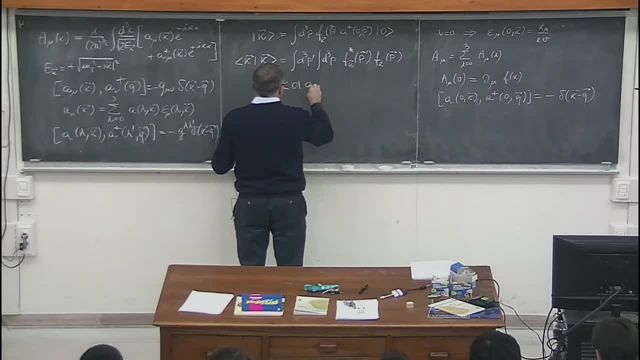 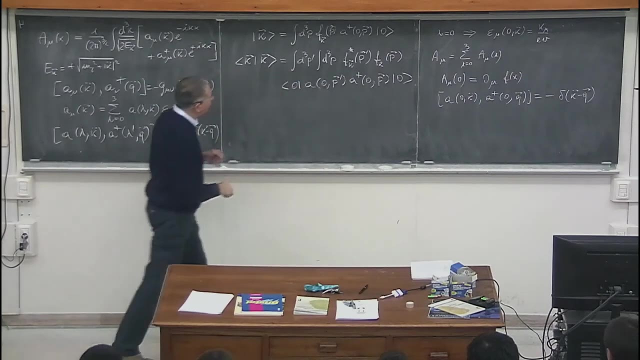 Vacuum state. a zero p prime, a dagger zero p vacuum state. Now I use the commutation relation, which has the wrong sign. And if I use the commutation relation I can commute these two: creation and annihilation operator. when a x on the right on the vacuum state gives zero. 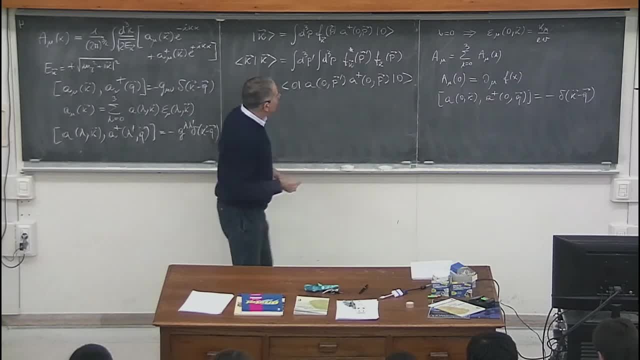 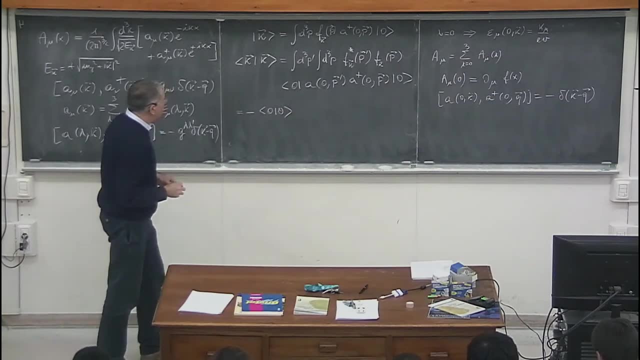 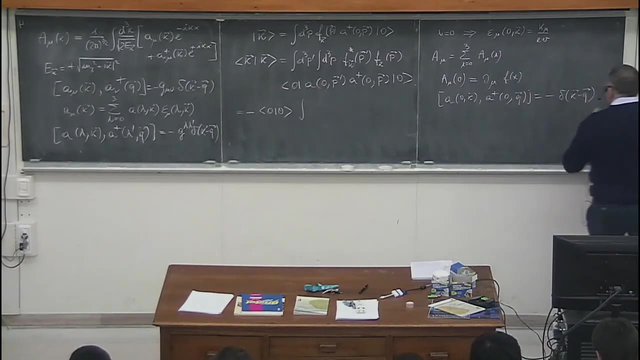 and you are only left with the commutator, which has a minus sign. So this is minus zero, zero. the norm of the vacuum state times integral. There is a delta function- p minus p, prime- which allows us to perform immediately. 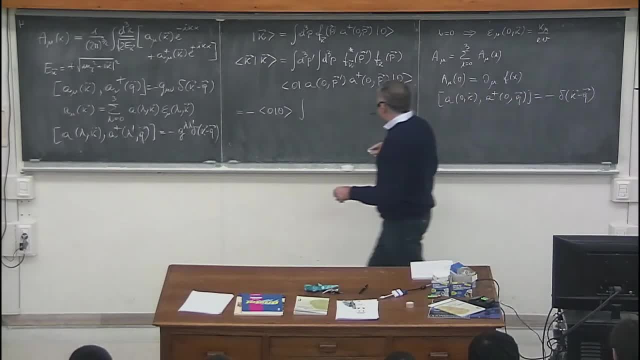 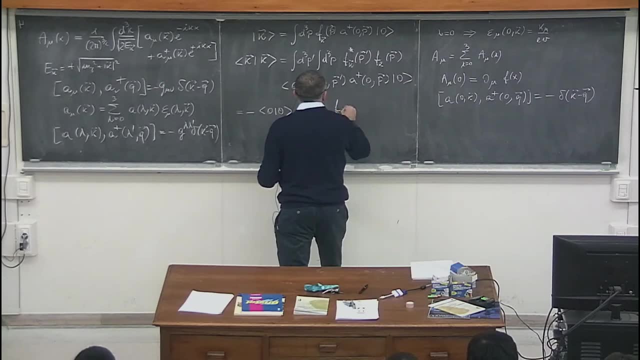 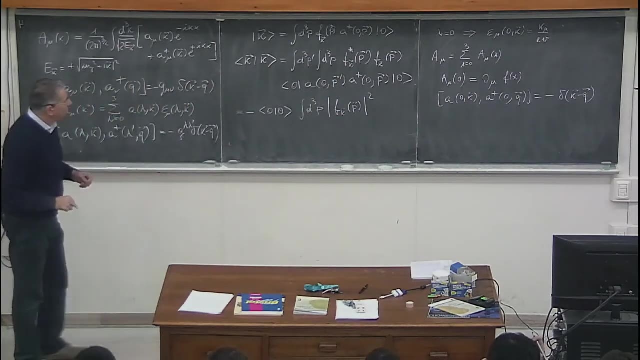 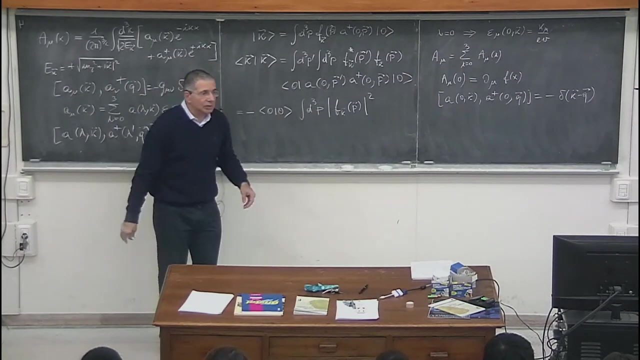 for example, the integral over p prime there And this gives you integral Integral over d3p times fk of p modulo squared. This is a finite integral because this is a wave packet, so it goes to zero rapidly at p equal to infinity. 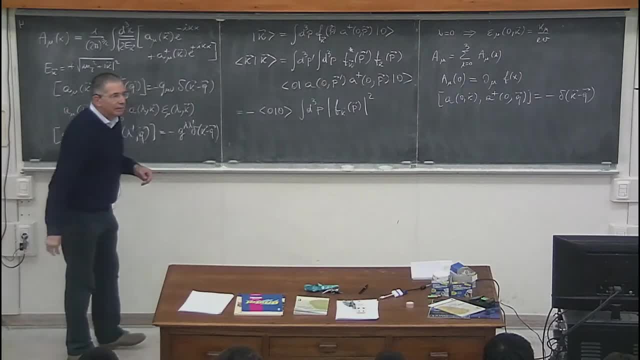 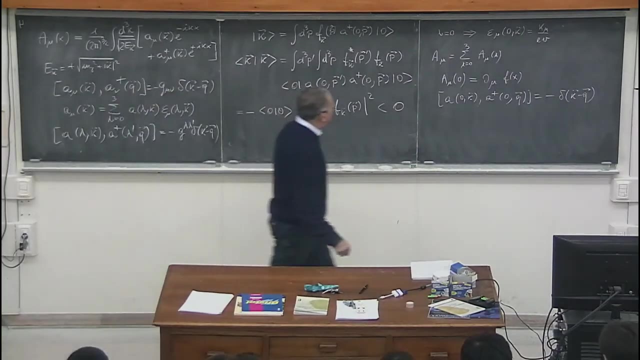 And it is positive definite because it is the integral of a positive function, The norm of the vacuum state. The state is assumed to be positive and there is a minus sign here, So this is less than zero. So I have to get rid of states with polarization zero. 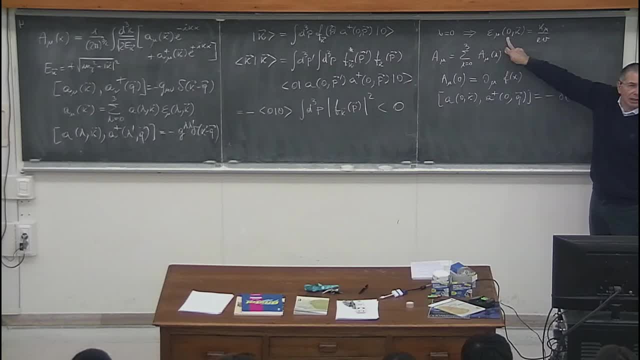 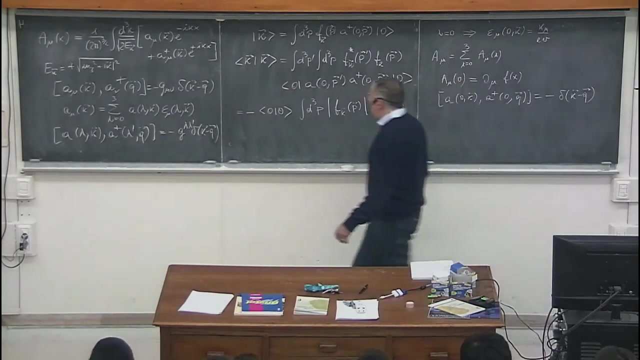 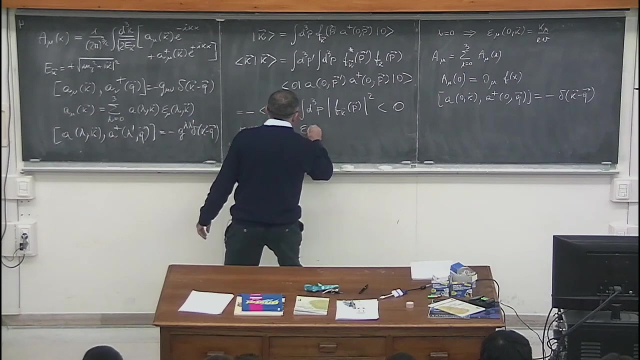 The polarization state corresponding to lambda equal to zero, do not belong to the physical state of Hilbert space of states And it is easy to get rid of them. So let's look at them. The way you get rid of them is to require that the polarization vector are such that